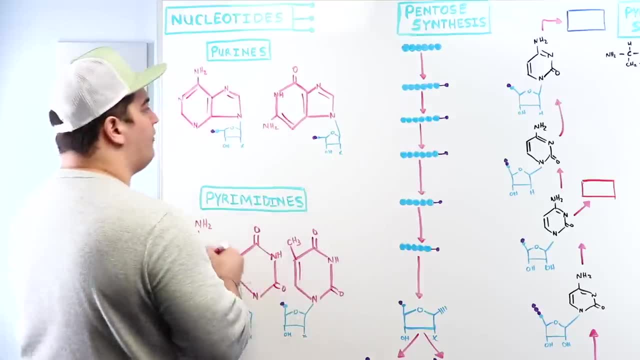 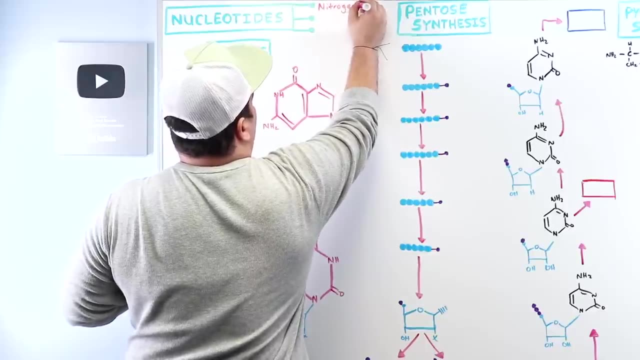 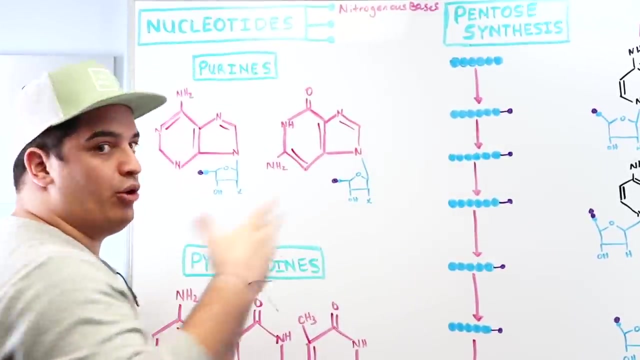 a nitrogenous base product And we're going to primarily focus on that in this video. but you need a nitrogenous base and we'll talk about those nitrogenous bases. Okay, That's one thing that we need. Okay, The second thing that we need is pentose sugars. Okay, So pentose sugars. 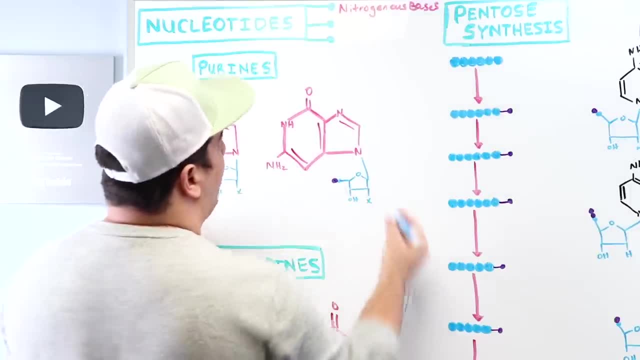 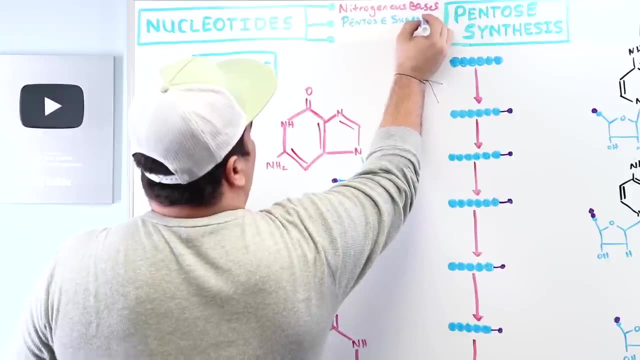 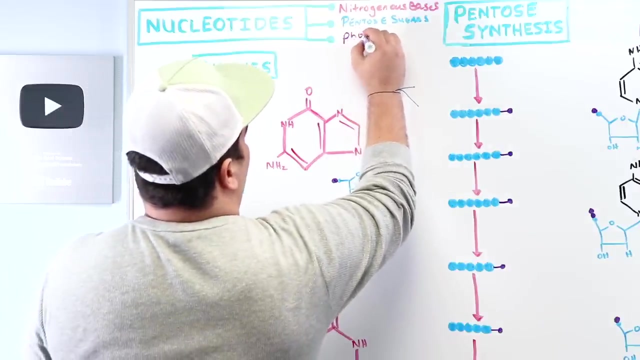 and that can be a deoxyribose pentose sugar, or it can be a ribose sugar, Okay. So we're going to need some sugar molecules, which we're going to call pentose sugars, Okay. The other thing that we're going to need is phosphate groups, Okay, And that's the last thing that we'll need here to 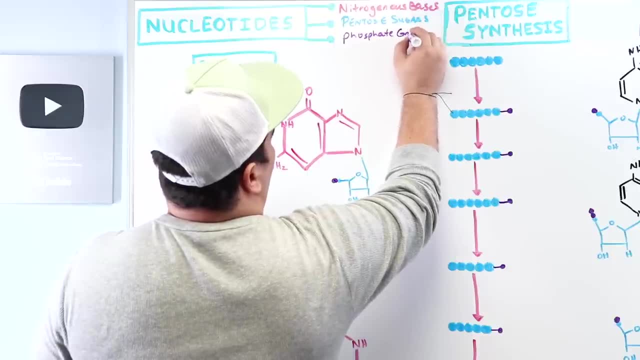 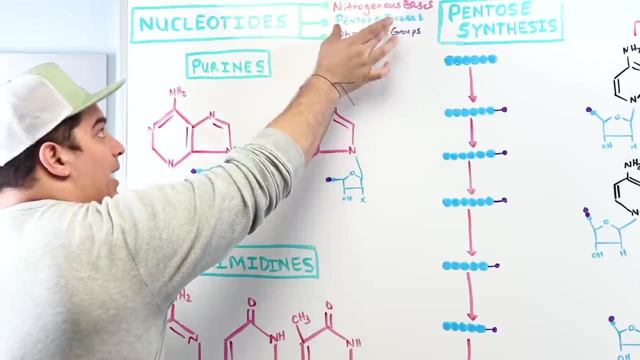 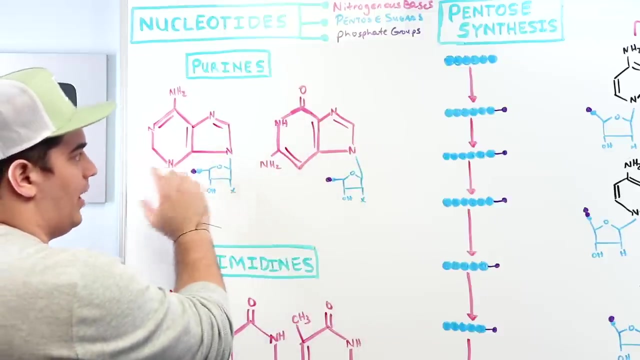 make these nucleotides So phosphate groups. So, now that we know the main components of our nucleotides, which is a nitrogenous base product, a pentose sugar, a phosphate group? what we're going to primarily focus on here is the nitrogenous bases, right? So this nitrogenous base, if you? 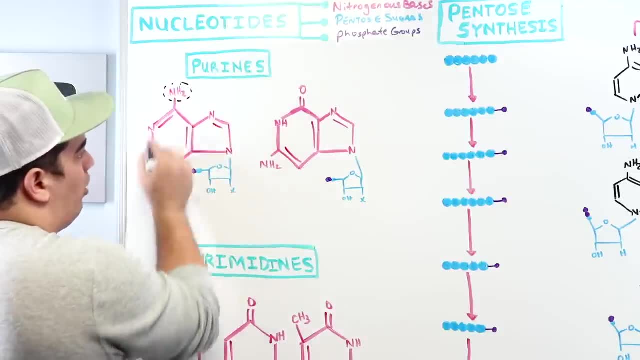 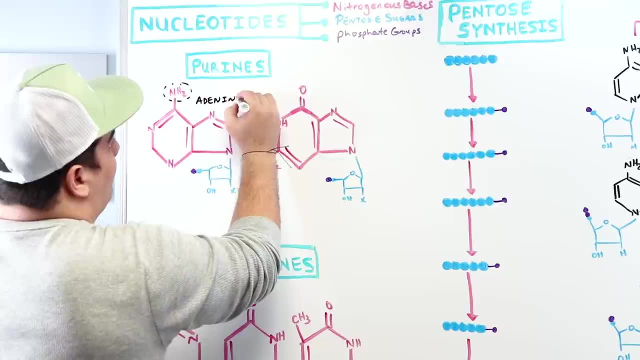 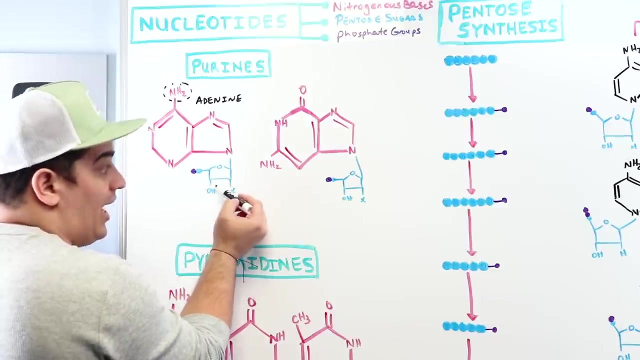 look here it's got this amine group here. We technically call this nitrogenous base adenine, So it's actually called adenine by itself. But then when you take adenine and you combine a pentose sugar with it, which could be either deoxyribose sugar, 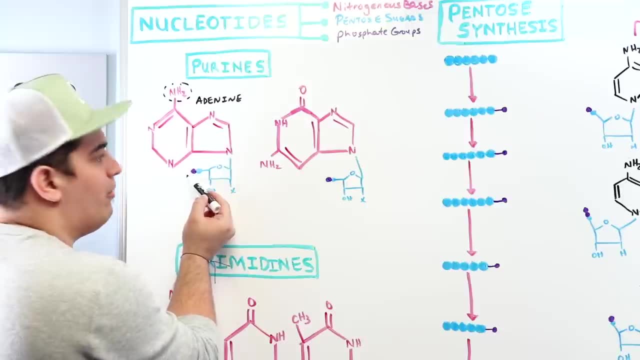 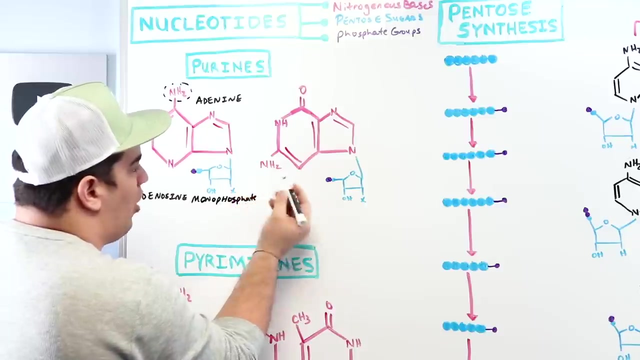 or it could be a ribose sugar and one phosphate which is a monophosphate. then we have a specific name for it. It switches from adenine to adenosine mono because one phosphate, monophosphate. That is also abbreviated AMP. So I want you guys to get used to that. I'm going to use some. 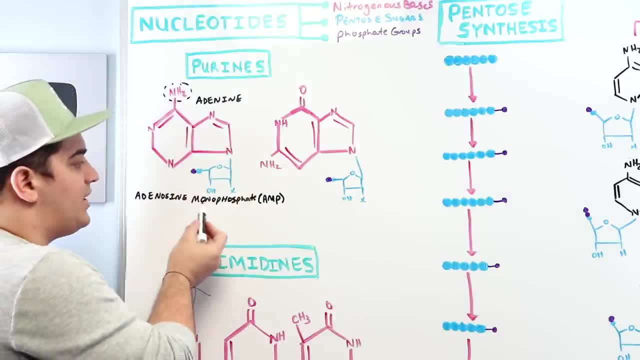 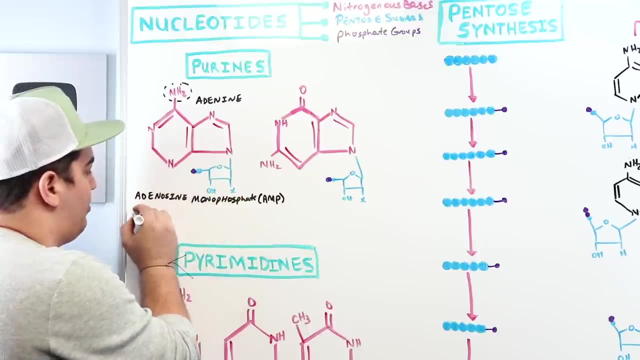 abbreviations in here, and that way you guys know where the heck it came from. Now this is: if it was a ribose sugar, right, A ribose sugar or ribonucleotide. If I want it to be a deoxy, I just 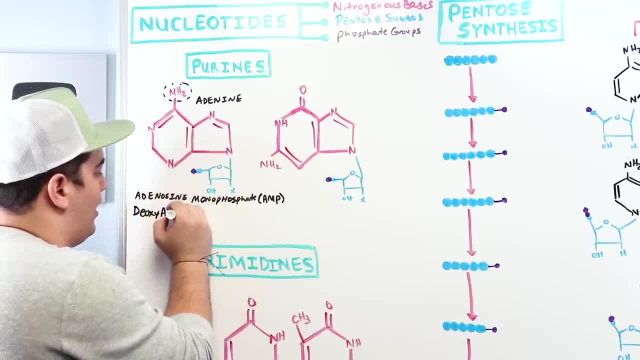 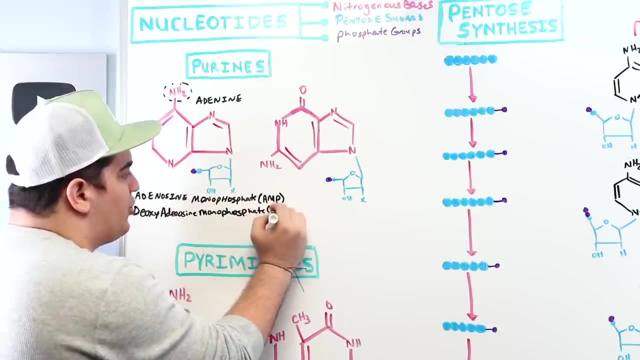 put the deoxy in front of it, And now it's deoxyadenosine monophosphate, And I'll show you what the difference truly is. And we put D A M P. Pretty simple, right. I'll show you what the 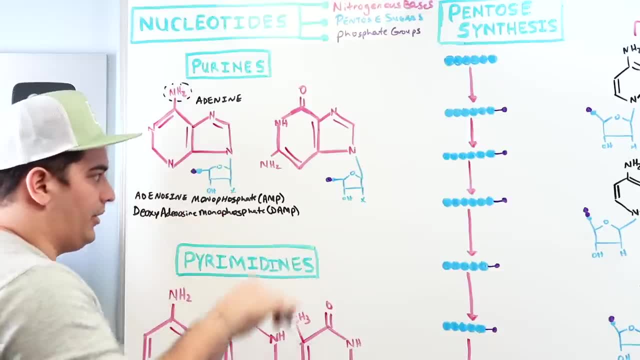 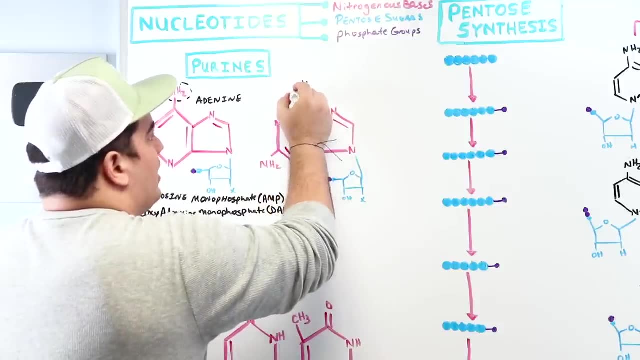 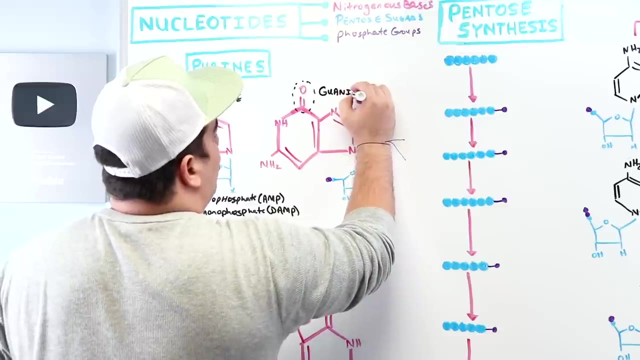 difference is between a deoxyribose and a ribose. sugar is in a little bit, All right. So the next one, the next purine over here, is going to be specifically a little bit different because it has this carbonyl group here and this is called guanine. Okay, It's called guanine, just the. 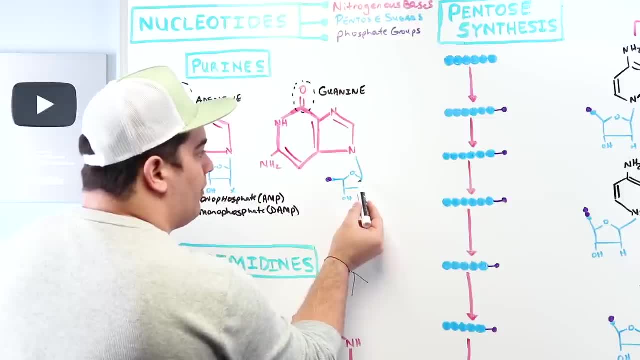 nitrogenous base product. But if we add on the ribose sugar it's going to be a deoxyribose sugar. If we add on the ribose sugar or the deoxyribose sugar with the monophosphate, then it changes. 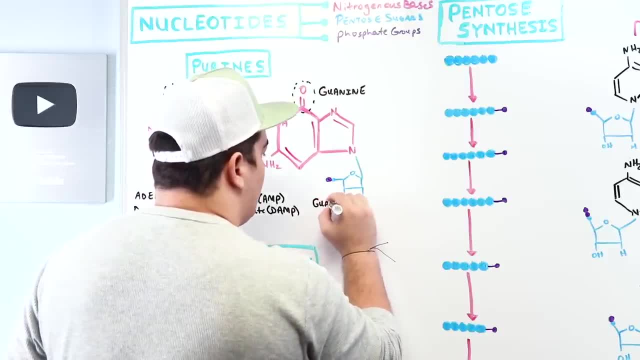 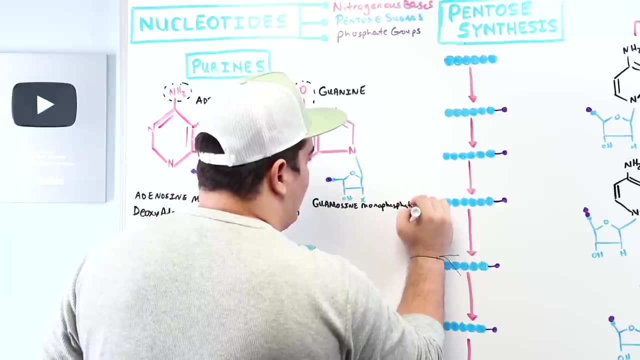 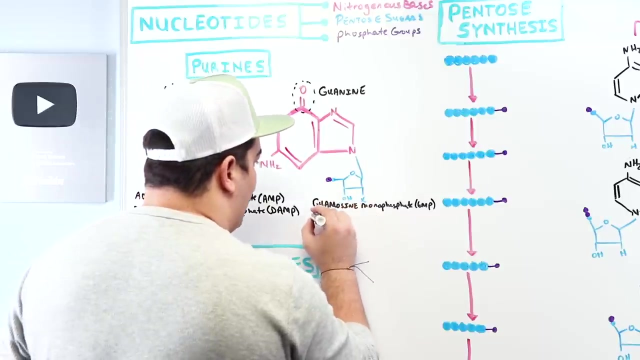 right, It changes to guanosine monophosphate, And this we can label G M P. If you want to make it a deoxy, we just make this a deoxyribonucleotide, And so it's now going to be deoxyguanosine. 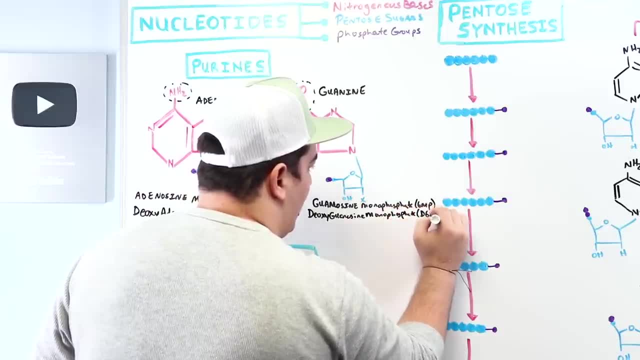 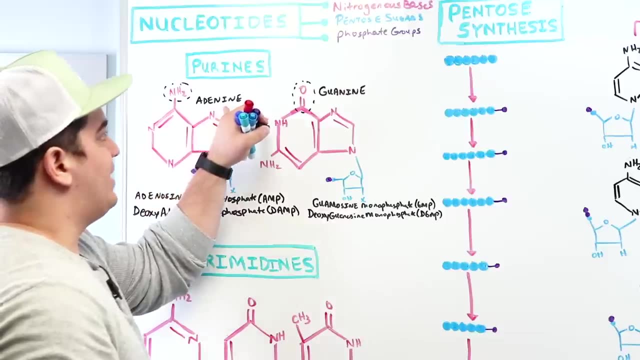 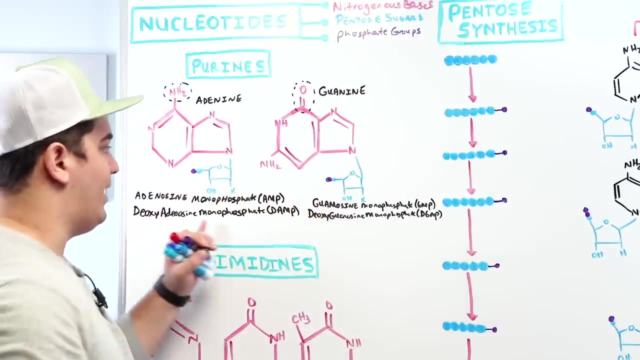 phosphate, And we abbreviate that D, G, M, P. Pretty simple stuff, right? That's our purines. Okay, Now, if you just want to remember the nitrogenous bases, it's adenine and guanine. But if you add on these sugar molecules and the phosphate, then we have to add this particular name to it. Okay, 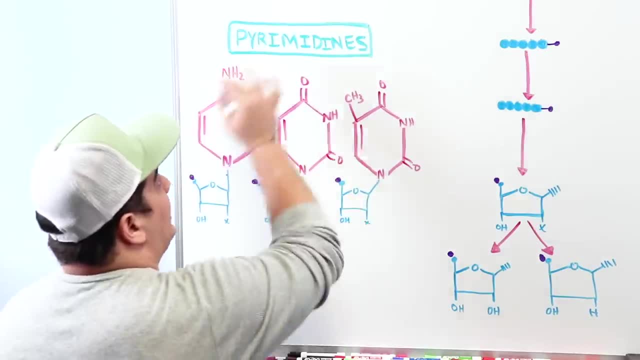 Now pyrimidines. let's move on to that, All right. So now we have our pyrimidines. Pyrimidines are going to be your single ring structures, And there's three of these types. So let's actually 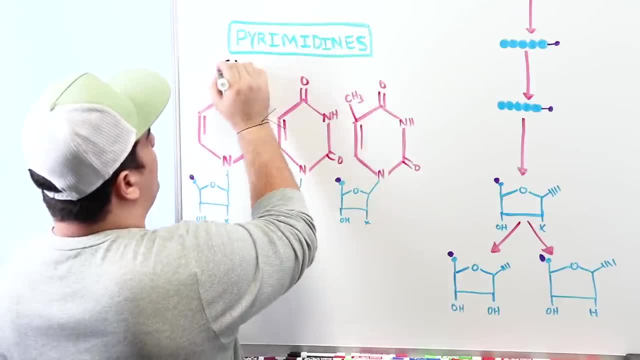 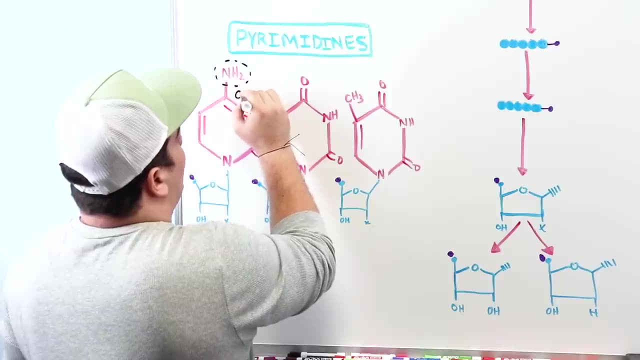 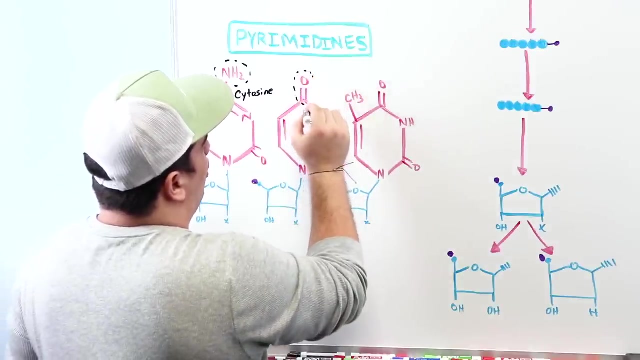 label the different types of nitrogenous bases. This one here, with its amine group and the single range structure, is particularly referred to as cytosine. Cytosine, This one here, and it has this carbonyl group here. right, But no methyl group. 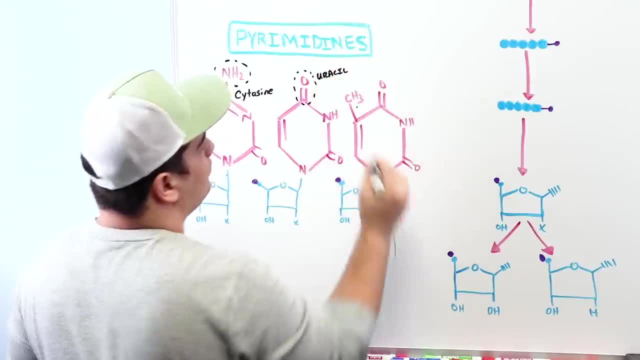 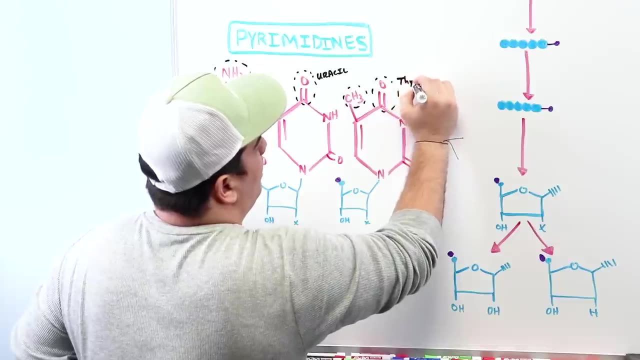 is referred to as uracil, And then this one here with the carbonyl group and this methyl group here is called thymine. Now we're going to go a little hardcore now, right, And we have to add on the name if it. 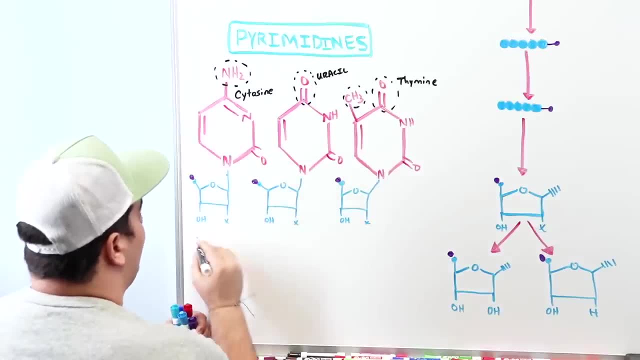 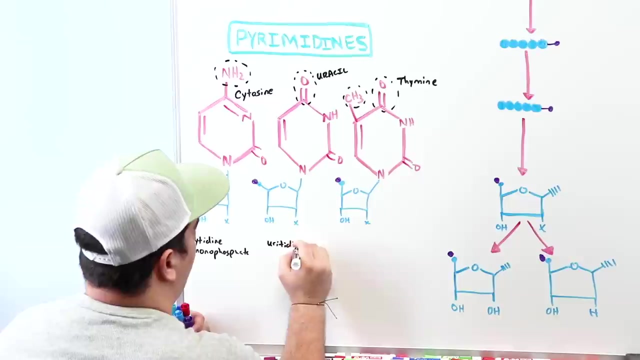 has a pentose sugar and a monophosphate, So now it changes from cytosine to cytidine monophosphate. If it's uracil, it's called uritidine monophosphate, Monophosphate, Monophosphate. 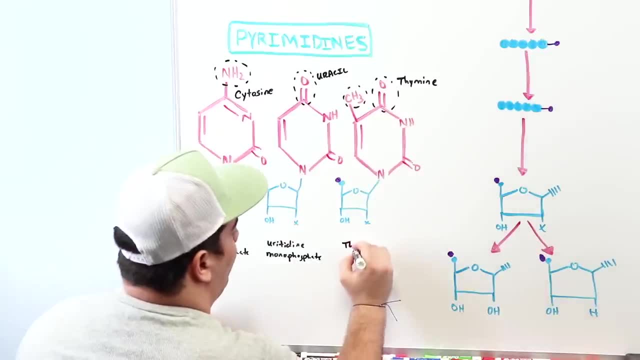 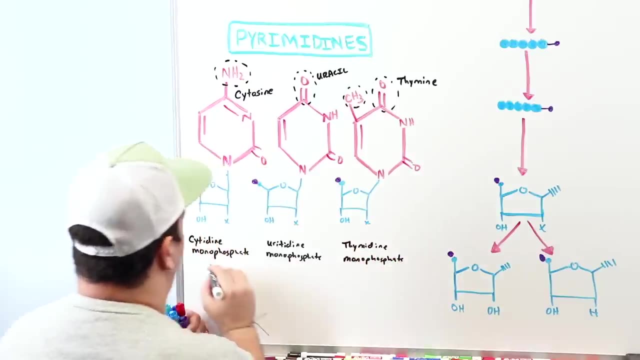 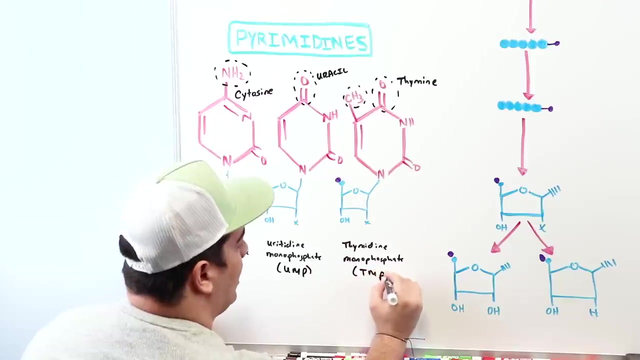 Monophosphate, Monophosphate, Monophosphate, Monophosphate, thiamine, it's called thymidine monophosphate and again, if we abbreviate, this is CMP, this is UMP and this is TMP. now, if I wanted to go another step, 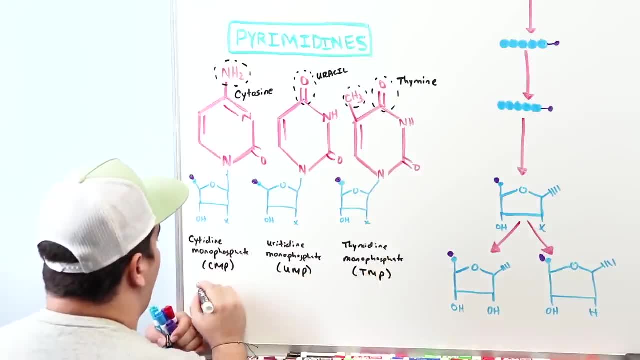 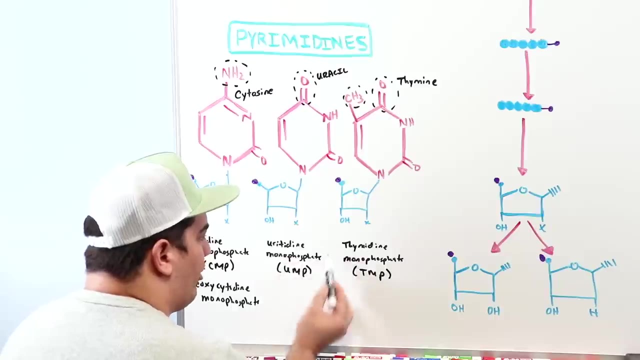 further, I could make it a deoxy. this would be for RNA. if I want to make it a deoxy for DNA, it would be deoxycytidine monophosphate. now, if we wanted uritidine to become a deoxy, even though it's not incorporated into DNA, we use it. 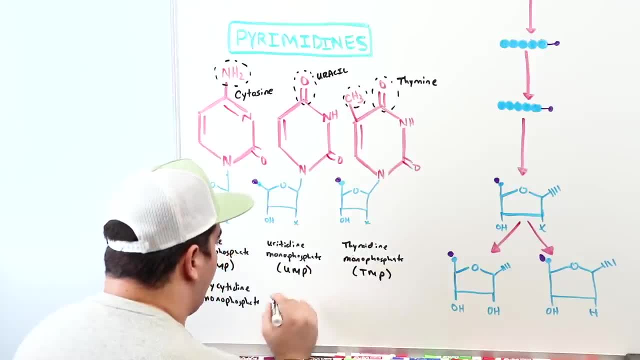 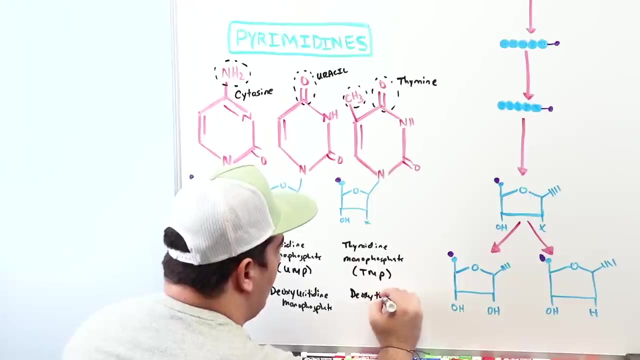 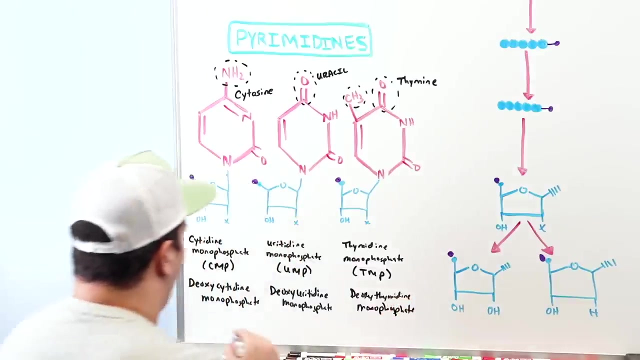 to make a deoxy thymidine monophosphate, we should write it as deoxyuritidine monophosphate and lastly, we should have deoxy thymidine monophosphate. now, what's the abbreviations DCMP, D UMP and D TMP, that is, the different nucleotides that we 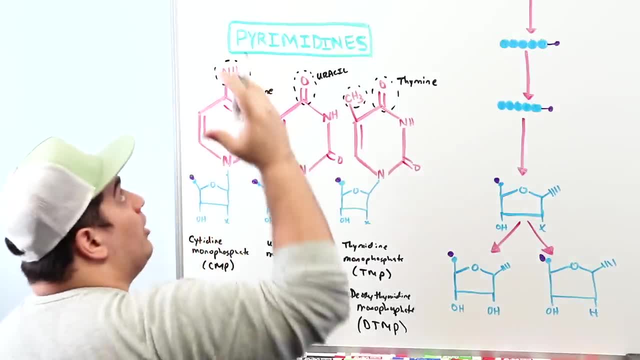 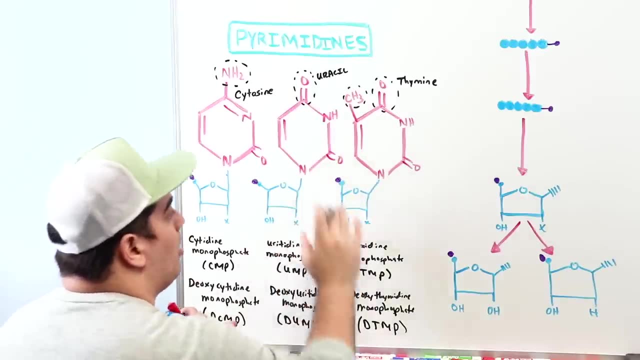 should be aware of. so now, now that we understand the names of the purine and pyrimidine nucleotides, as well as their individual nitrogen and nicotinases bases, let's move on next to talk about the pinto sugar synthesis. alright, so we talked about the nucleotides, we talked about purees, and 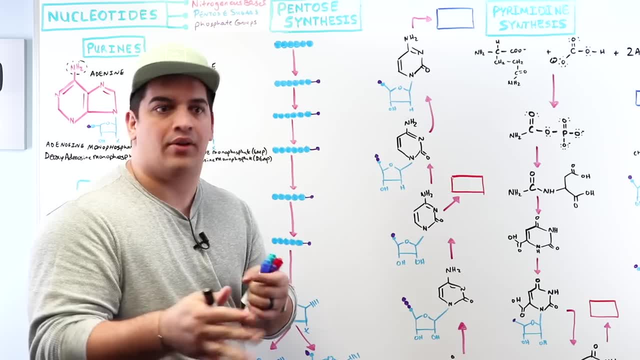 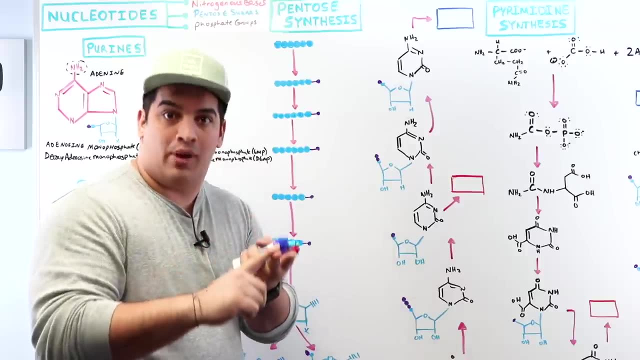 pyrimidines, what they technically are their names. get the nomenclature down. now we got to build these puppies up. alright, now that we know, understand the nomenclature for purees pyrimidines, their nitrogenous basis and we know what it makes up a nucleotide, let's go ahead and start making them in order to make. 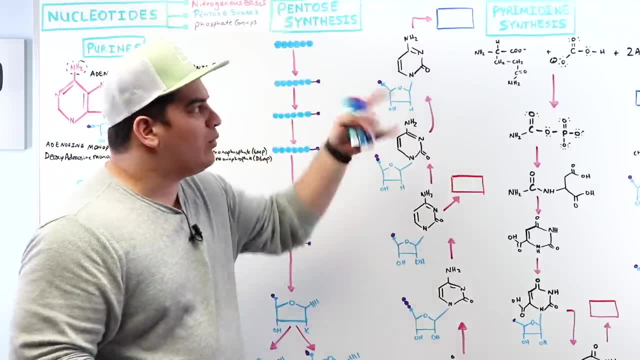 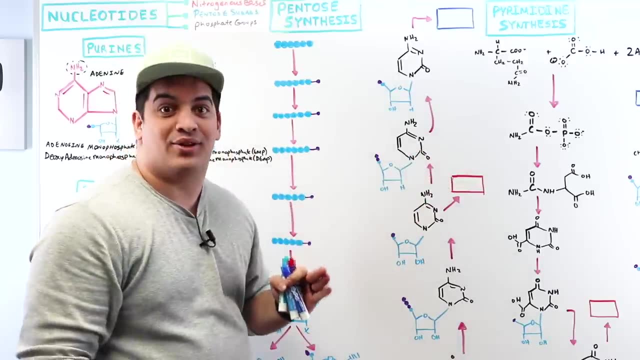 them. we have to have pinto sugars, and let's see what our original male was doing. we'll talk about some of the nitrogenous bases and how they're synthesized, and then how we can combine the nitrogenous bases as well as these pinto sugars to 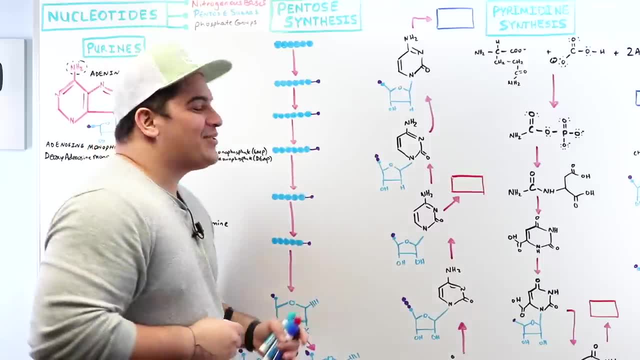 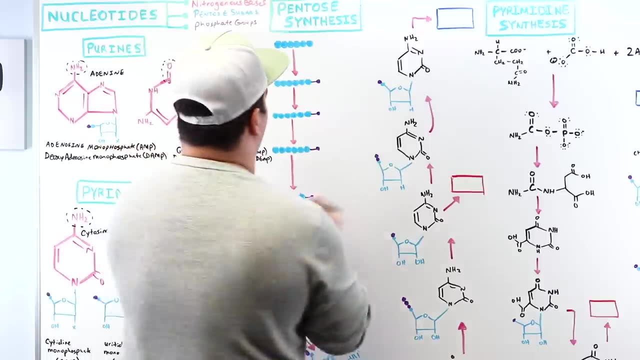 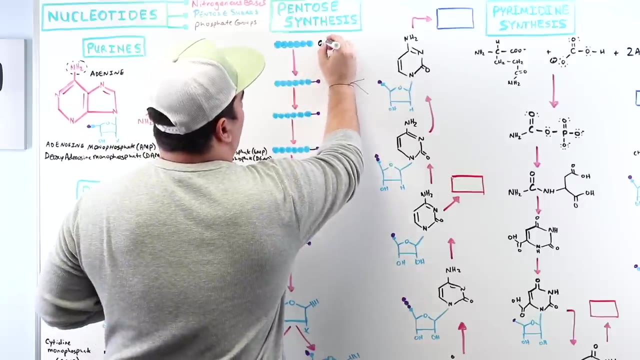 give us these potential nucleotides. all right, you guys remember the pentose phosphate pathway. it's bad. so if you guys remember back from the pentose phosphate pathway when a cell has glucose coming into it, right. so here's our six carbon sugar molecule called glucose. glucose once it enters into a 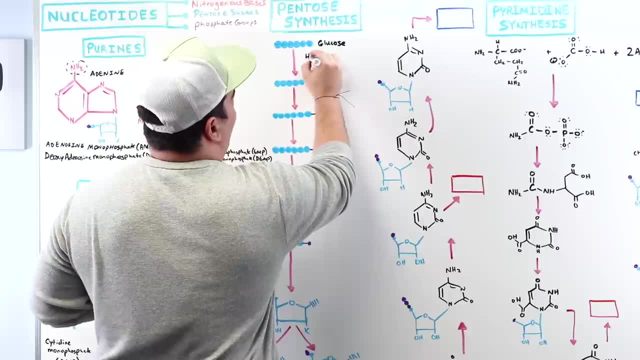 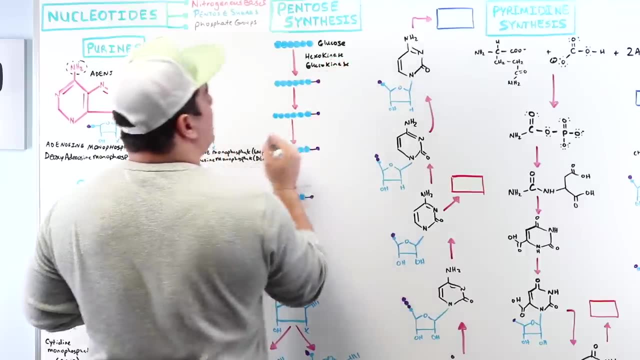 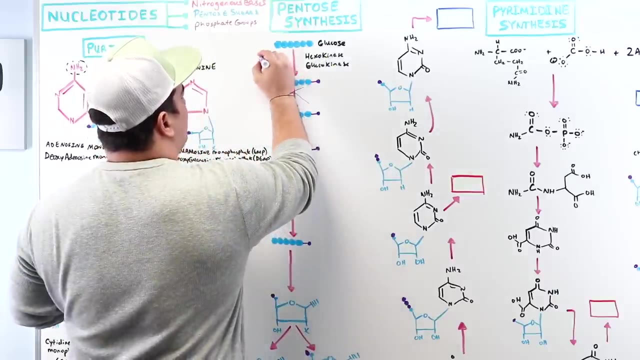 cell right. there's different types of enzymes, maybe a hexokinase, or there could be what's called a glucokinase, and what these molecules do is is they take and they phosphorylate glucose at the six carbon right. so in other words, we take ATP and we put a phosphate onto this, so we lose one of the phosphates. 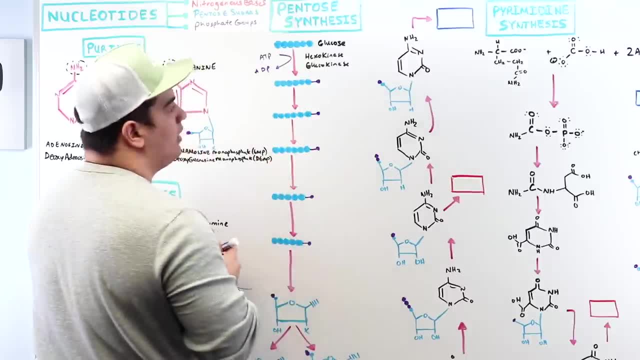 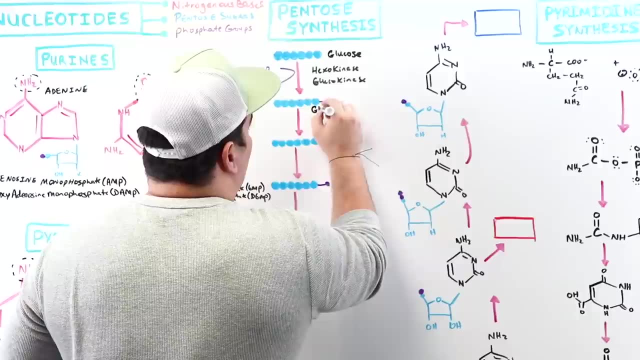 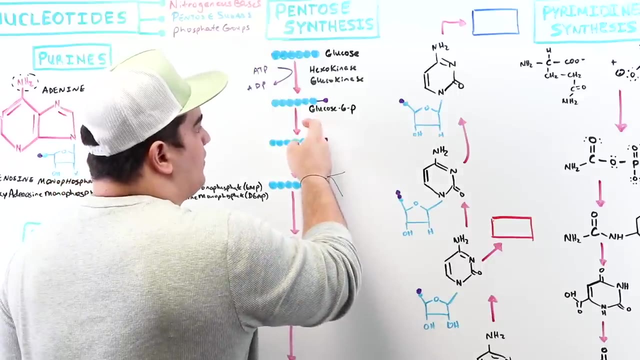 and that gives us ADP. where'd that phosphate go? right there. so now we have to give a name to this new molecule that now has a phosphate onto it, and this is called glucose six phosphate. right, pretty simple. right now. glucose six phosphate can either go through the glycolysis pathway or can go through this pentose phosphate pathway. 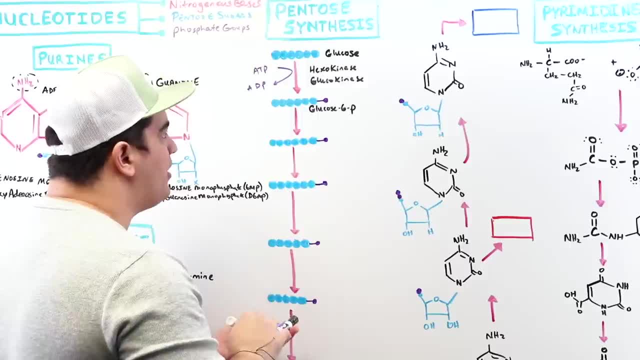 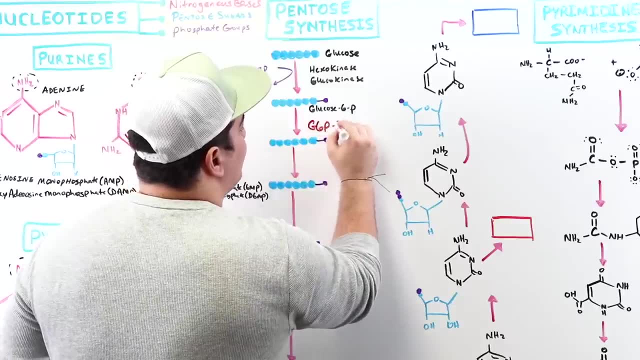 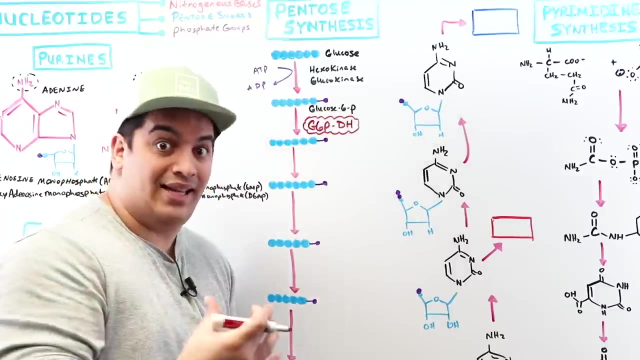 if it goes via the pentose phosphate pathway. you remember, there's a particular enzyme- we're gonna abbreviate it- called glucose six phosphate dehydrogenase and, if you guys remember, a hydrogenase enzyme pretty much always utilizes an NAD or an NADP positive molecule. Well sure, 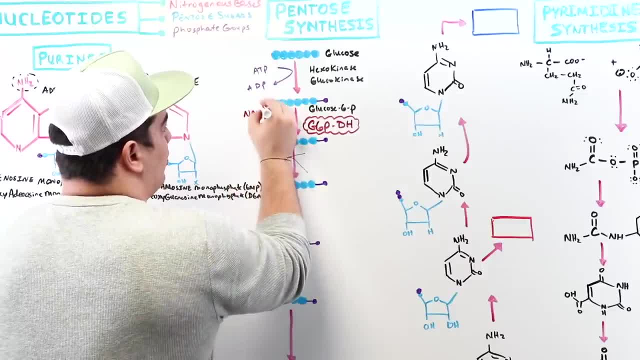 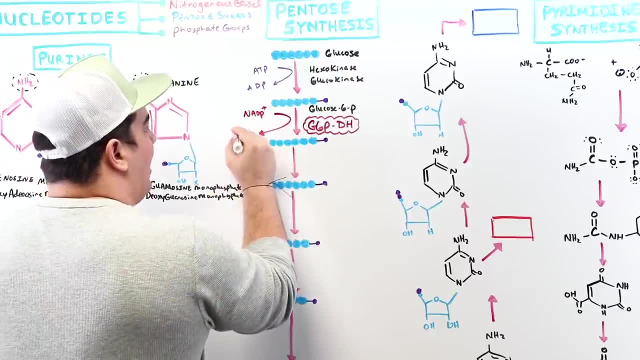 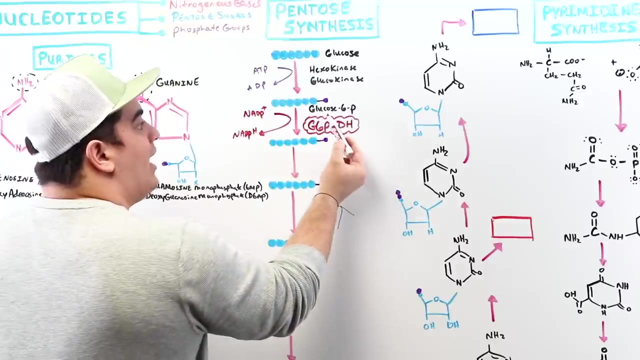 enough. that's what happens. We take an NADP positive molecule and we pick up some hydrides, which is a hydrogen with basically two electrons and a proton right, And we add on to that a hydride, So now it's NADP positive to NADPH, And in that process we convert glucose 6-phosphate. 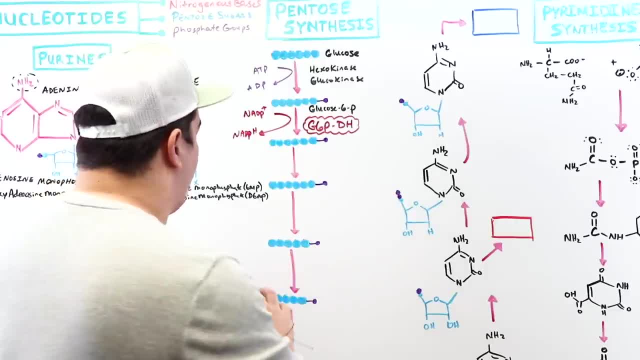 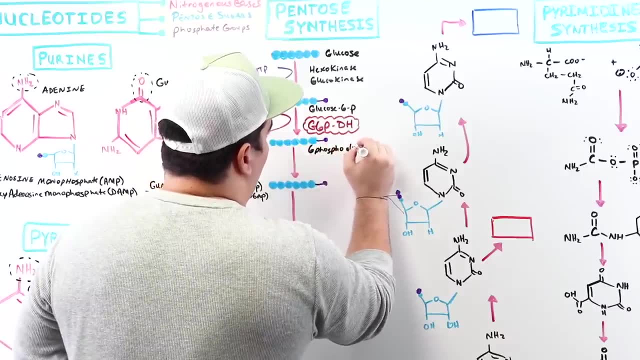 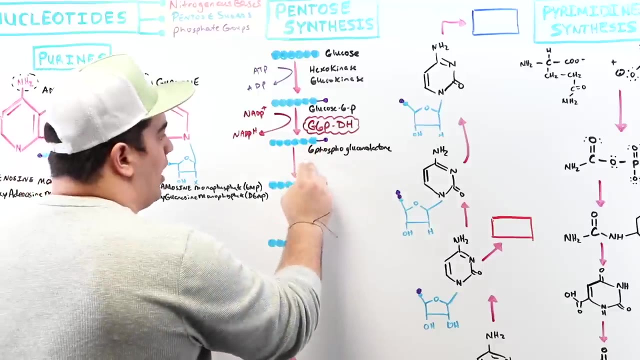 into a new molecule when we pull off those hydrides. This new molecule is called 6-phosphogluconolactone. Then what happens is, with 6-phosphogluconolactone, what we're going to do is we're going to add. 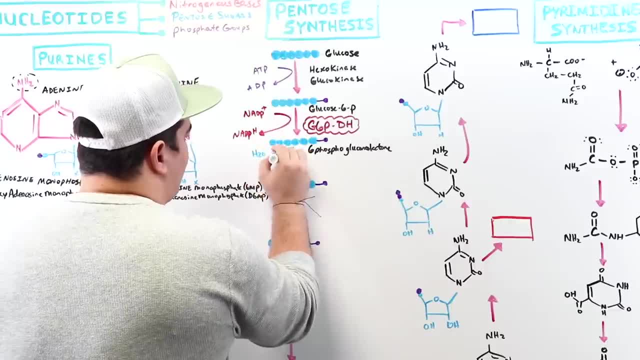 some water into this reaction. So we're going to take and add some water into this reaction, And when we do that, we convert 6-phosphogluconolactone with this water, And when we do that, we convert 6-phosphogluconolactone with this water. 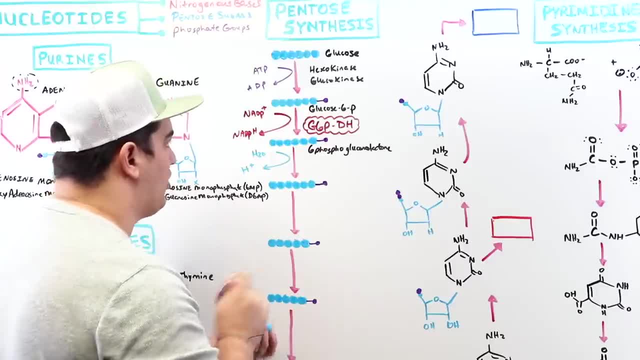 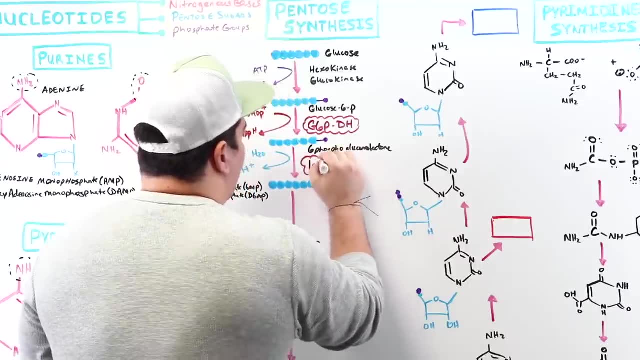 And a particular enzyme. if you guys wanted to know the enzyme, it's called lactanase. It's called lactanase. Again. we go over all this in the pentose phosphate pathway, But lactanase facilitates this process and converts 6-phosphogluconolactone into. 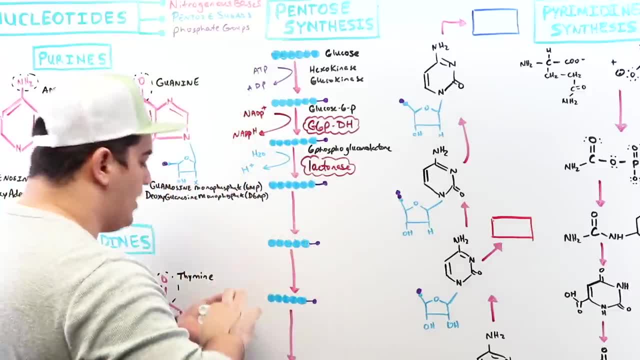 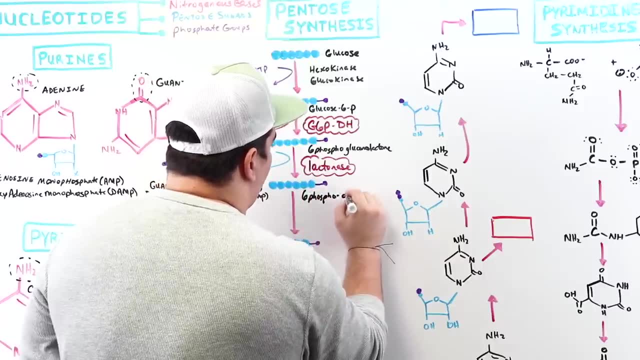 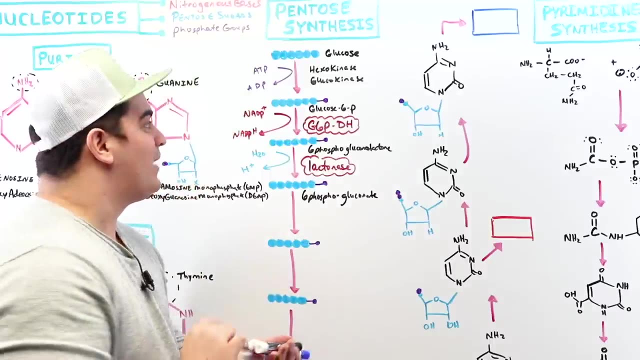 6-phosphogluconate. So now, this next molecule is called 6-phosphogluconate. Now, 6-phosphogluconate is a molecule that's called 6-phosphogluconate. Now, 6-phosphogluconate has to react with another enzyme. This next enzyme is called: 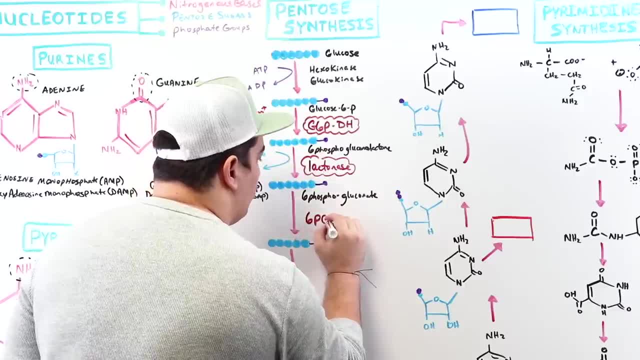 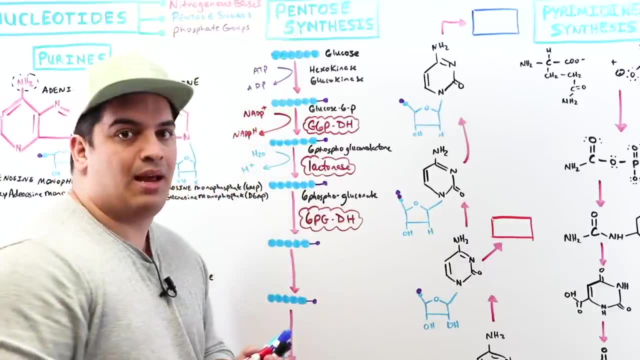 I'm going to abbreviate it: 6-phosphogluconate dehydrogenase. Oh boy, If we got this bad boy coming in here, what does that mean? We need an NADP positive to convert it into an NADPH. 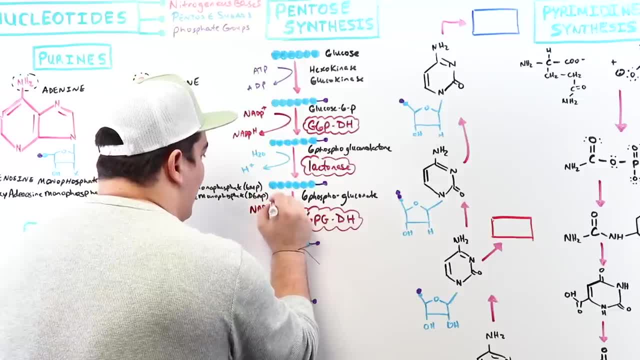 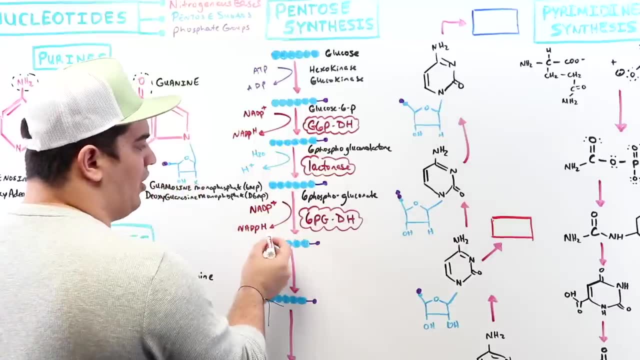 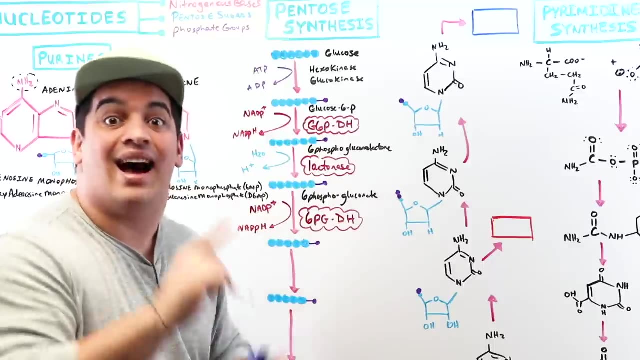 So I need to pick up some hydride ions off of this molecule and convert this into NADPH, And you guys remember where the NADPHs go to right? Remember they're involved within the glutathione pathway, which is important for basically helping to regenerate that antioxidant-like type of molecule. 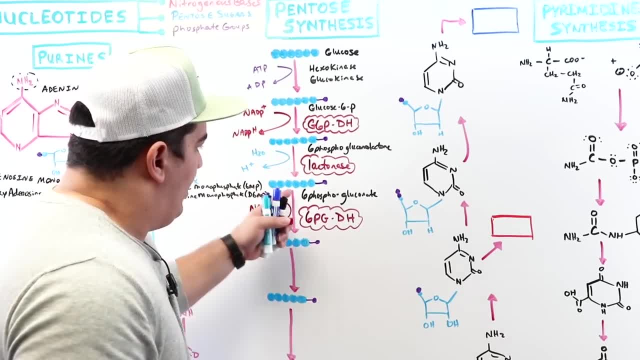 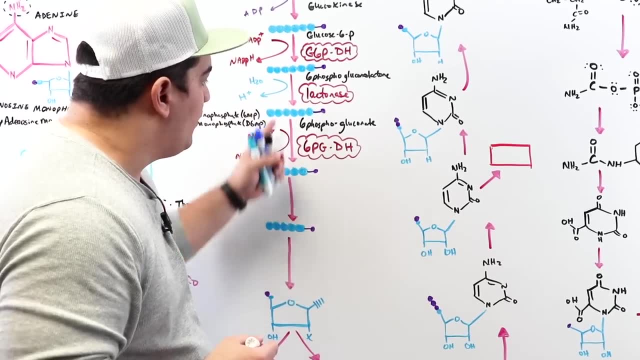 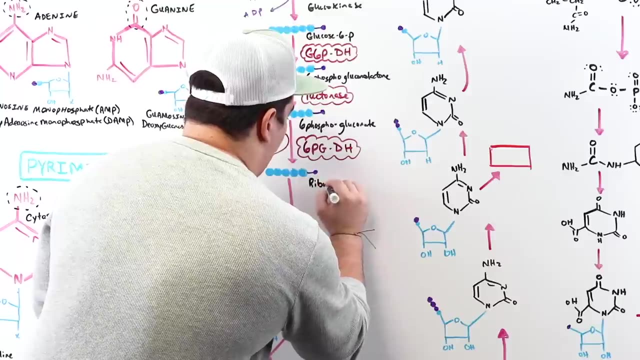 whenever there's a lot of free radicals. Now, whenever you do this reaction where you reduce the NADP positive to NADPH and oxidize 6-phosphogluconate, you turn it into another molecule called ribulose 5-phosphate. So now we have what's called ribulose 5-phosphate. 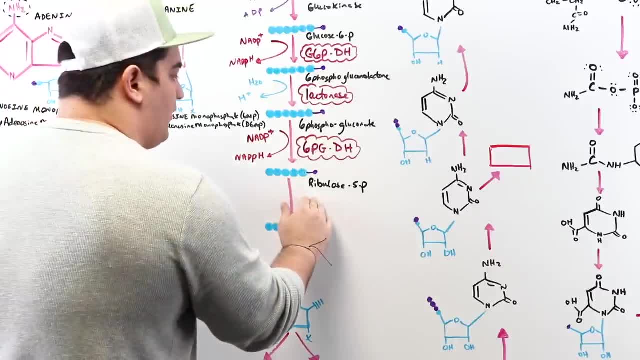 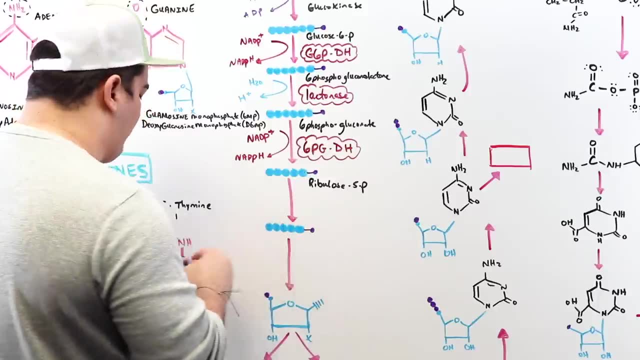 Phosphate, Now ribulose 5-phosphate, is then going to undergo another type of reaction here and there's an enzyme, and it's an isomerase enzyme. You know ribulose 5-phosphate. it technically has a ketone. 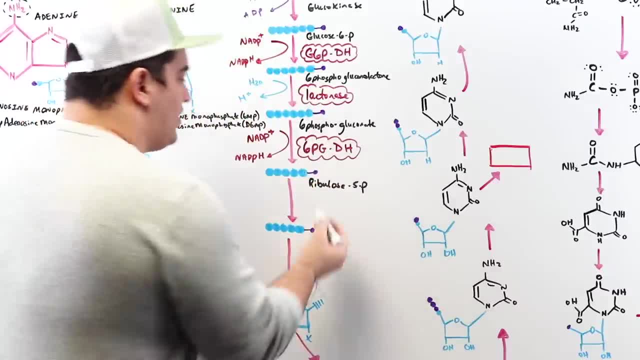 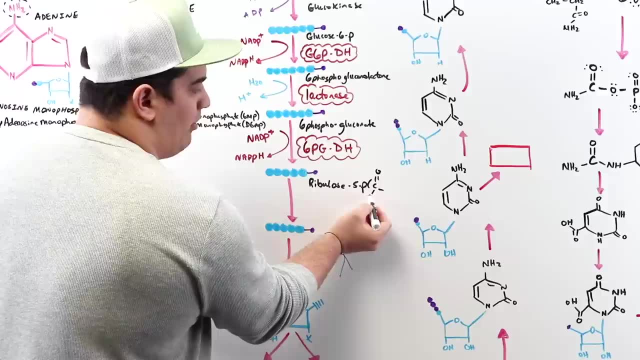 Sorry. Okay, So you know, ribulose 5-phosphate. it's technically a ketone, which means it's carbon doubly bound to oxygen and then bound to two carbons on the side here. Well, what we're going to do is we're going to convert this into an aldehyde. 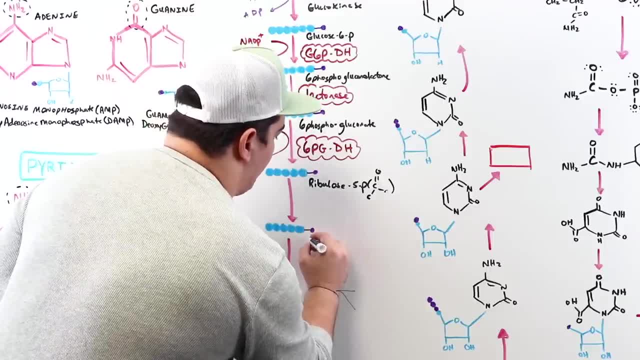 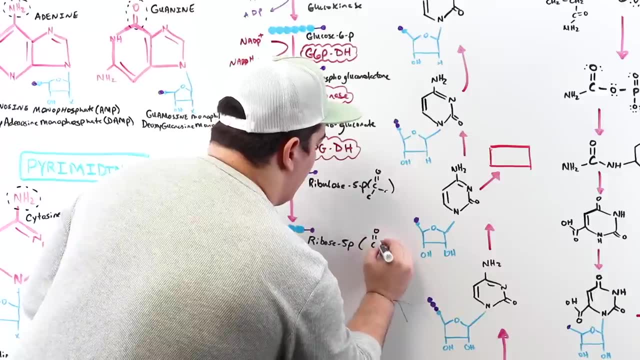 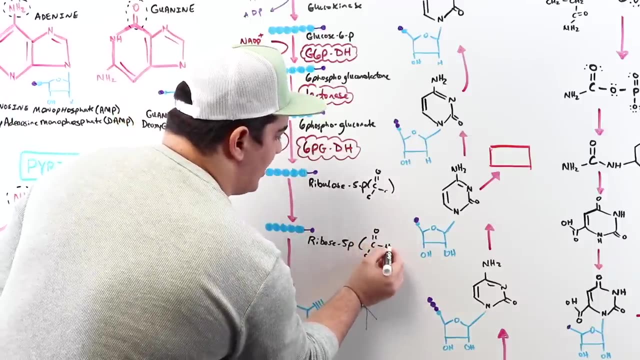 And whenever we convert this into an aldehyde via an isomerase enzyme, we convert this into ribose 5-phosphate, And now we just converted it into an aldehyde. Okay, And this actually is a carbon here. So it's a carbon doubly bounded to an oxygen. 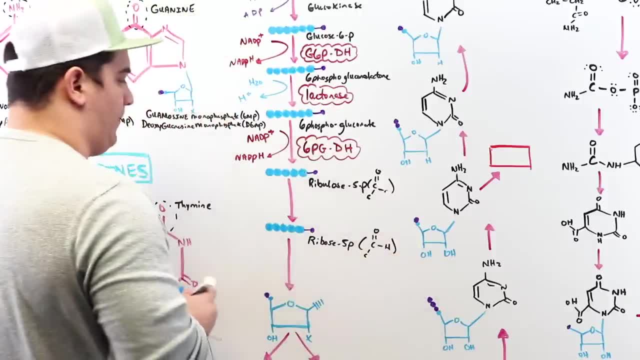 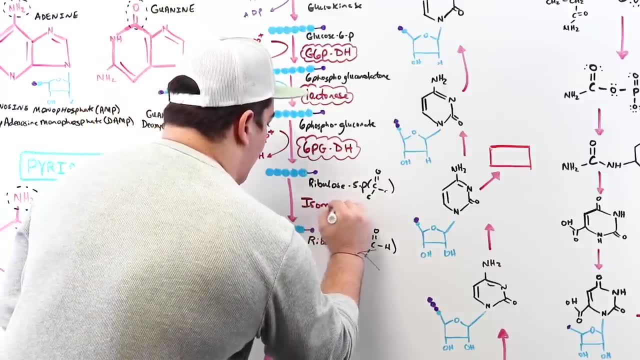 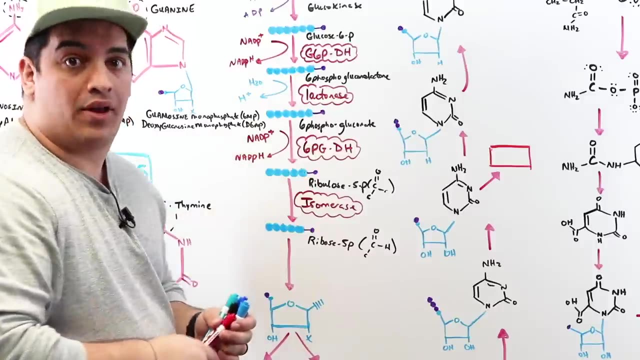 singly bounded to a hydrogen, singly bounded to another carbon, That's our aldehyde. And in order to do this we need that enzyme called isomerase. So this is a isomerase enzyme. Okay, So we're not adding anything, We're just kind of flopping the atoms around on that molecule. 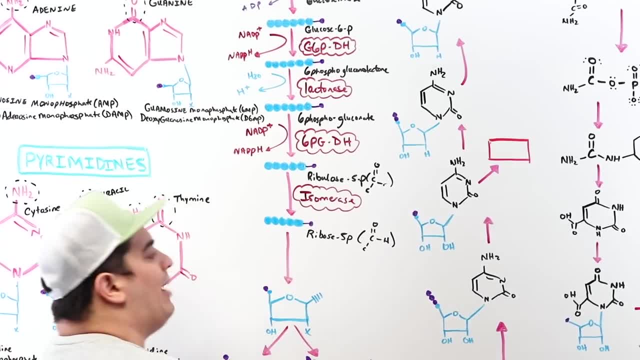 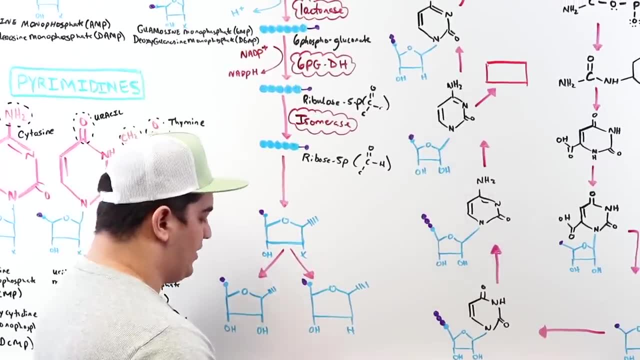 Now here's where we get into the next big thing: Ribose 5-phosphate. we're going to kind of make a ring out of it, Okay, And in order to make a ring out of this, we need what's called a ribose. 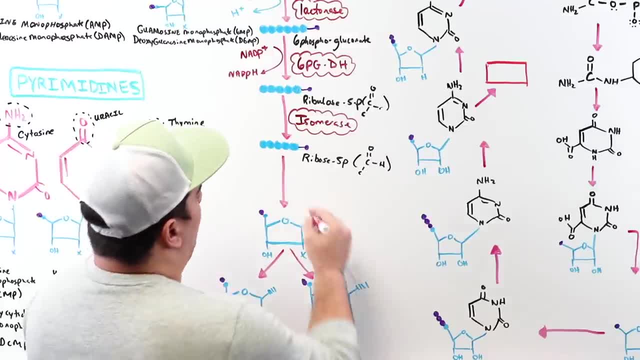 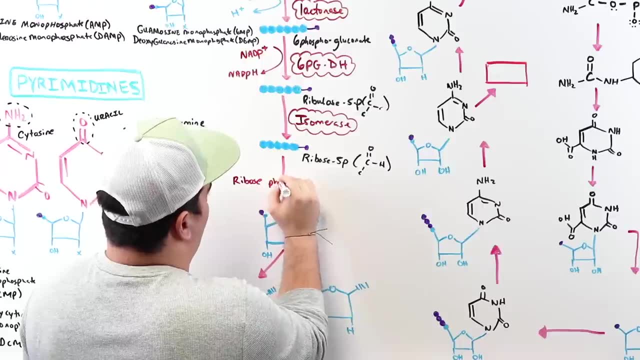 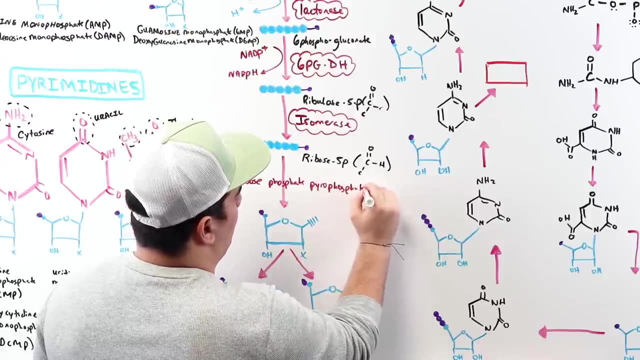 This enzyme has one heck of a name. It is called- and I'm going to write this, I'm going to need all this space here- Ribose phosphate, pyrophosphokinase, This enzyme, okay, which is a pretty cool enzyme. 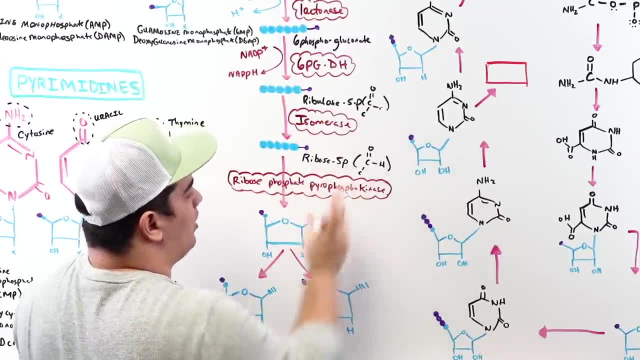 What it does is: it helps to kind of take this ribose 5-phosphate and make it into a ring, And whenever we do that, we're going to get a ring out of it, And we're going to get a ring out of it. 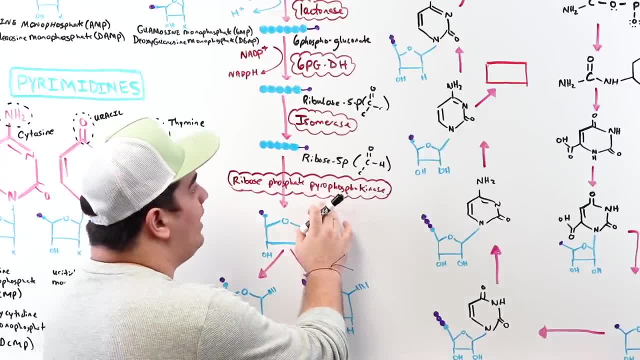 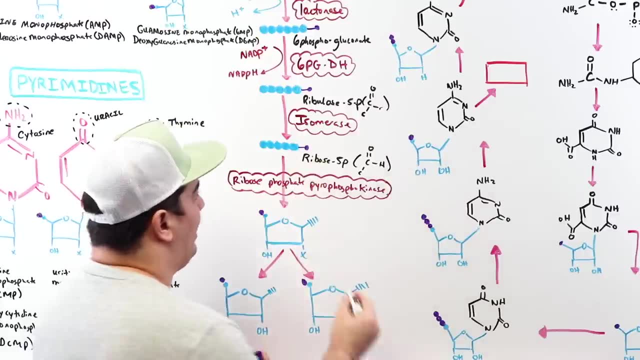 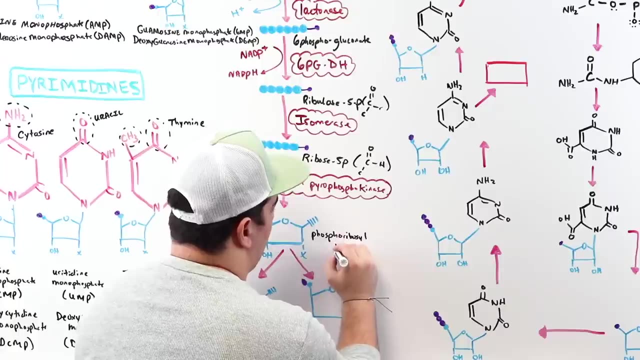 Now we have this new molecule. So now what we made is- you know what we did- is we're going to add another phosphate group onto ribose 5-phosphate and we're going to help to close this structure and make a ring, And now we make what's called phosphoribosyl pyrophosphate. 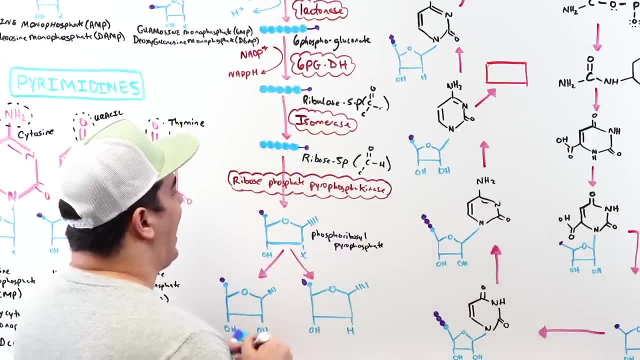 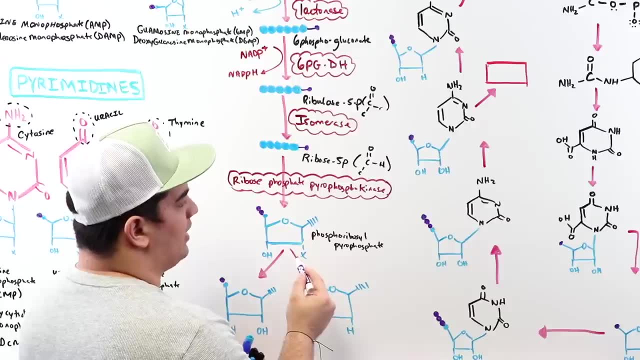 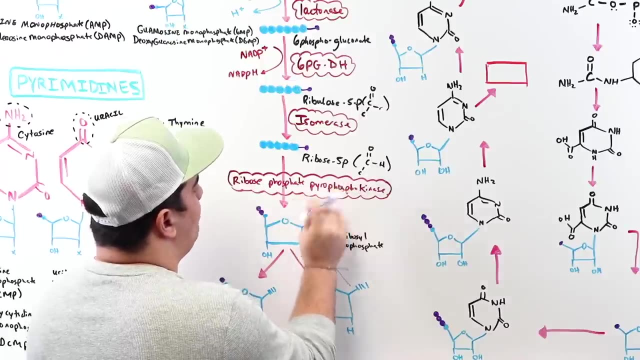 So, in order to do that, we make the ring and then we have to add on another phosphate group. So that means that we had to utilize um, an ATP molecule, within this process, right? So we had to utilize a phosphate- actually two phosphates- in this process, So we had to take ATP. 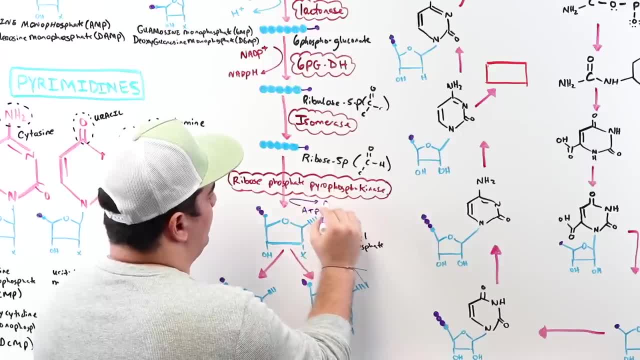 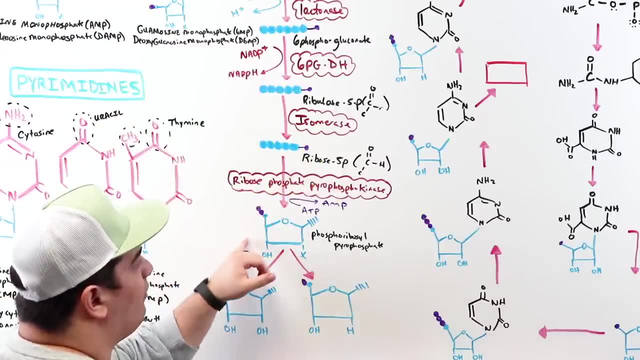 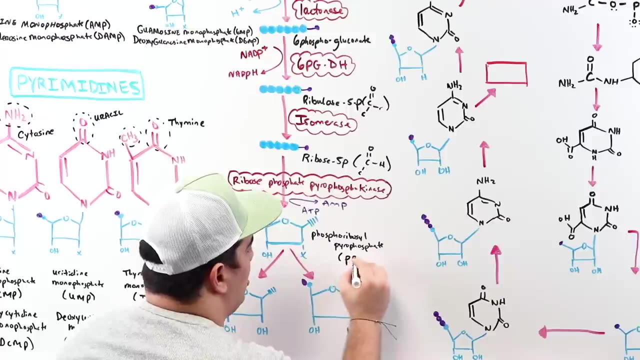 and convert this into AMP. Okay, Now here's where I wanted to tell you guys the difference here. So we have our phosphoribosyl pyrophosphate, which is also commonly abbreviated as PRPP, So you might see this written as PRPP. 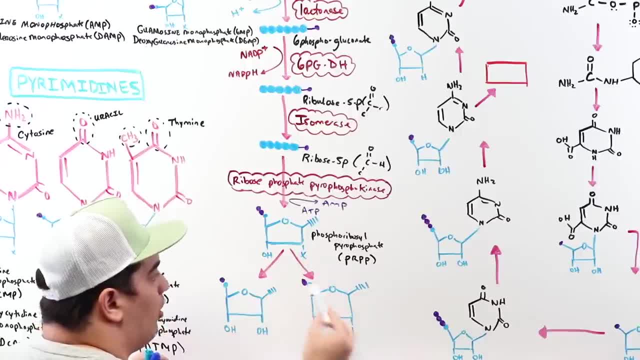 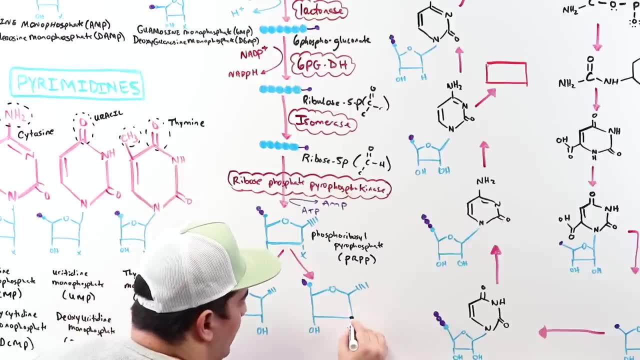 What happens is, remember, I told you that there's two different types of ribose sugars. One is called a deoxyribose. The big difference here is that on this carbon, here you notice, here on this carbon, that we have two different points right, And, if you guys remember, you have a one carbon two. 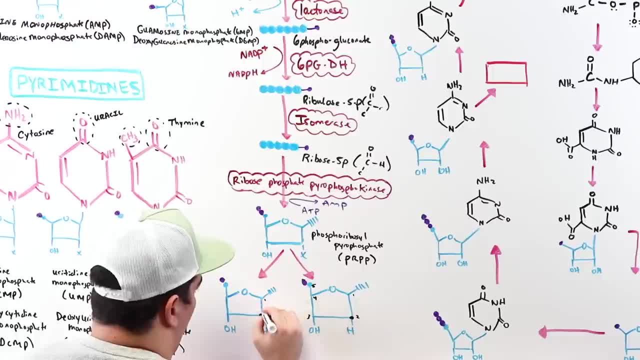 carbon, three carbon four carbon five carbon, one carbon, two carbon, three carbon, four carbon five carbon. On the second carbon, what happens is it Differentiates these two based upon what atom you have hanging off of that carbon, If there's a. 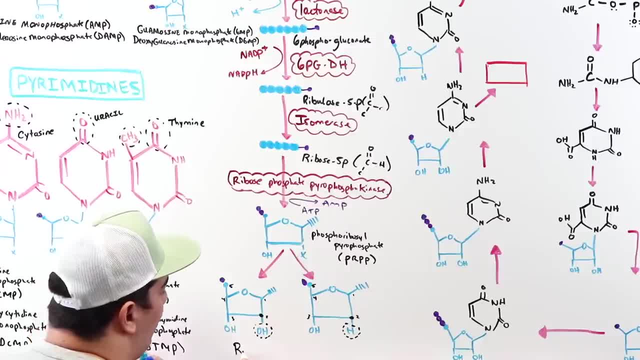 hydroxyl group on the second carbon, then it is a ribose sugar, And if there is a hydrogen hanging off of that second carbon, then it's a deoxyribose sugar. Okay, Now, what we're going to do is: 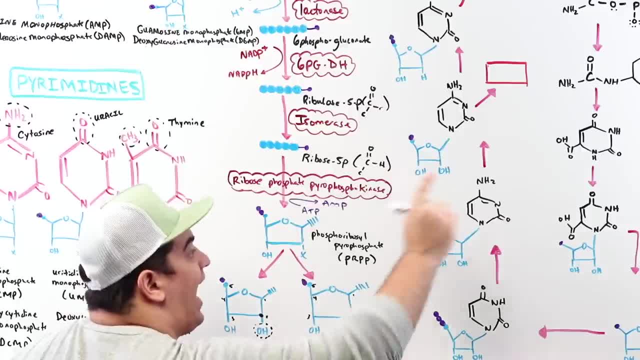 is we're going to take these PRPP molecules and we're going to add it to the nitrogenous bases When we go over those steps, which is going to be now all right. so now we're going to do is we're going to talk about the 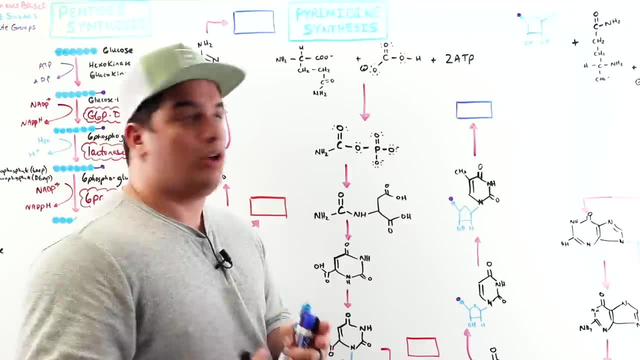 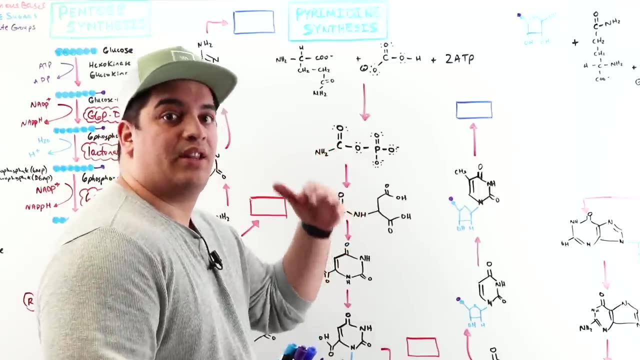 synthesis of perimeter, And so we've already synthesized our Pinto sugars, which are going to be components of the primitives. but now we have to add in those other molecules- right Which was the site to seeing the URA cell, and the thymine into that to help us to make these nucleotides. 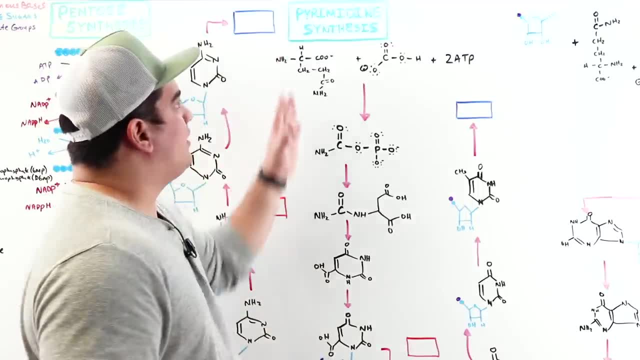 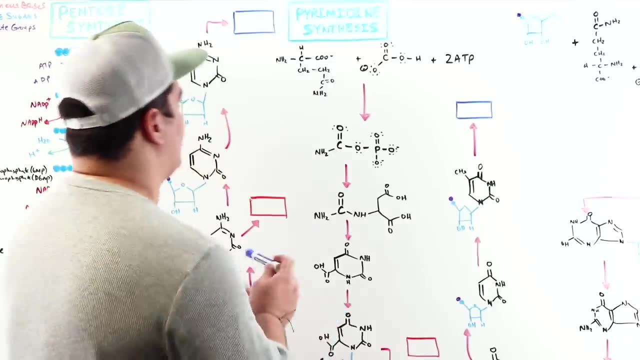 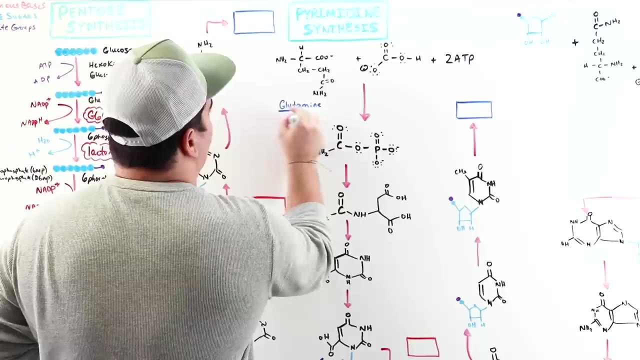 in combination with the phosphates as well. So how do we synthesize perimeter? Well, technically, what you start off with is three molecules. One of these is called glutamine. Okay, So you have this amino acid called glutamine And what you need with the 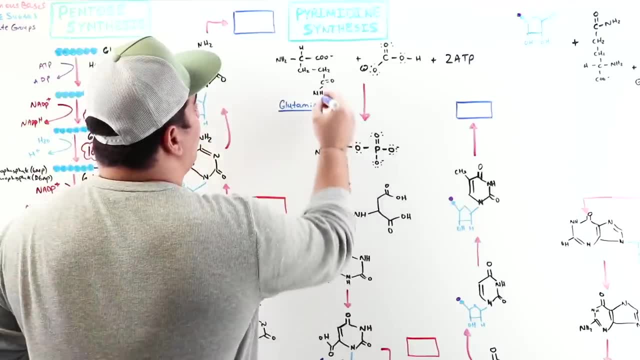 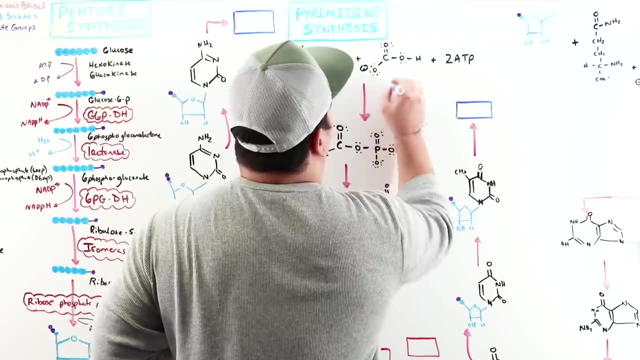 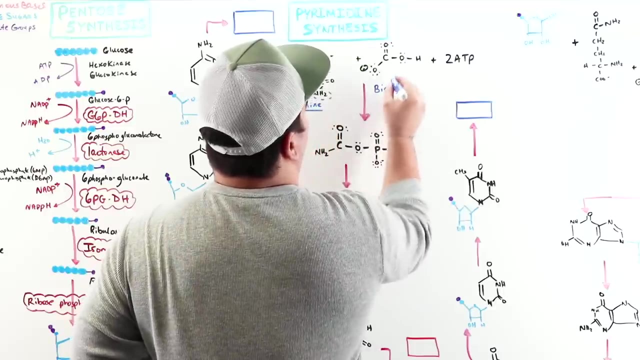 glutamine is actually the amine group, So we're going to be utilizing an amine group off of this glutamine. Okay, The next molecule is going to be called carbon bicarbonate, So the other one here which we have here is called by carbonate, And we need this bicarbonate to help us to build up this. 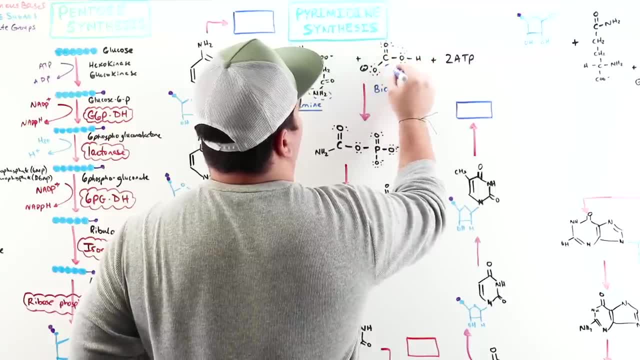 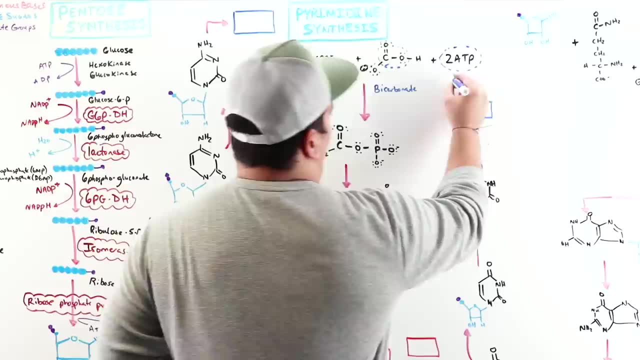 carbon, along with this double bond oxygen component. here We're going to need this As well. And then we're going to need ATP in this reaction because we're going to be adding phosphates on, So again, we're also going to be having ATP. So glutamine bicarbonate, ATP. 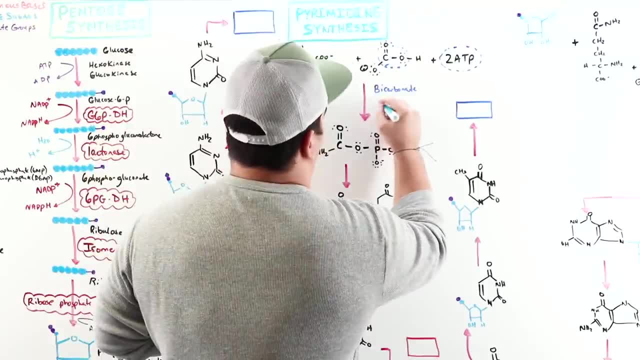 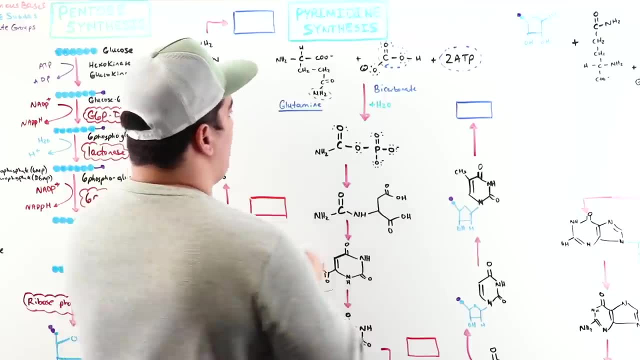 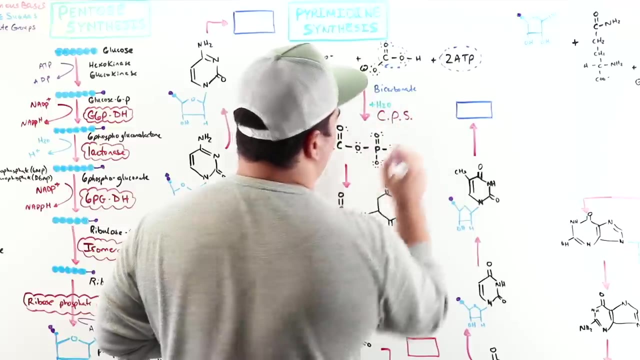 and also some water in the reaction as well. You also be utilizing, if you want to remember, some water, and through this we have to use a special enzyme, And this enzyme is called carbon oil phosphate synthetase. That should sound familiar, Isn't that? from the 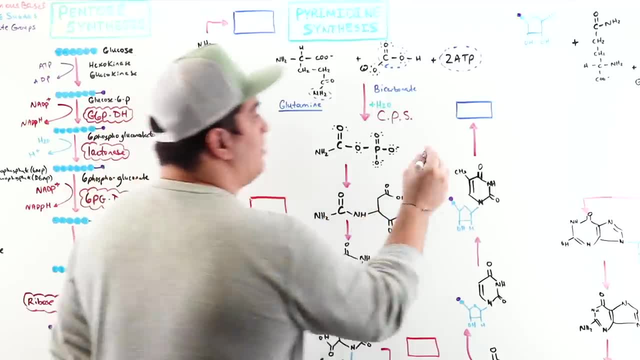 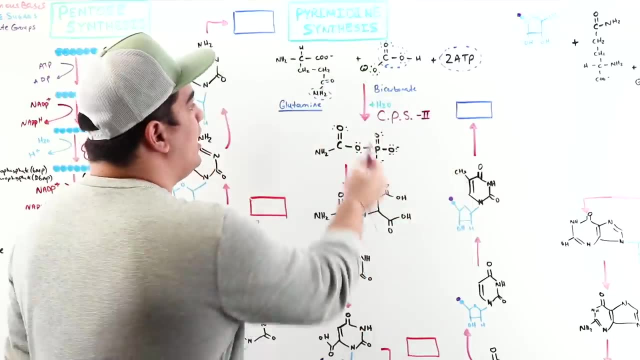 cycle? Yes, it is, But there's two enzymes, type one and type two. This is the enzyme in this pathway is type two, So carbon phosphate synthetase. type two is going to take glutamine, bicarb, water and two ATP molecules and synthesize a new molecule. 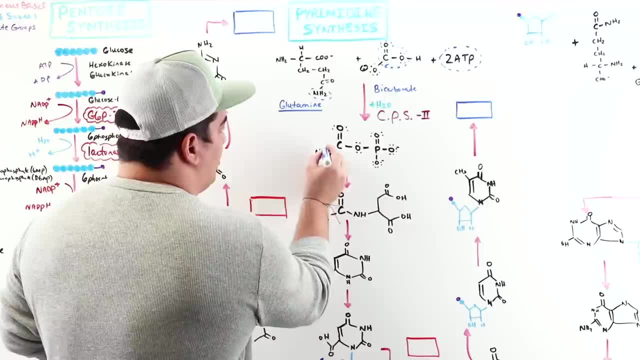 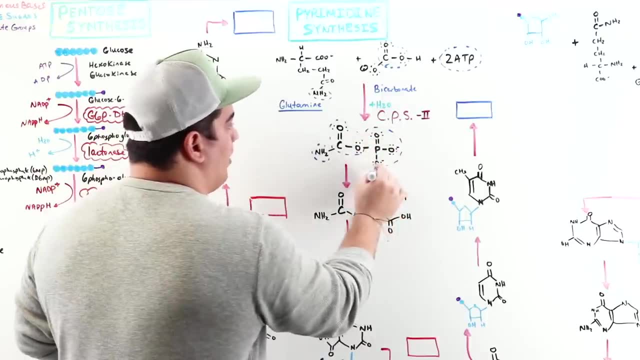 What is this new molecule here called this new molecule which got the amine group here from the glutamine? It got this carboxyl group here from the bicarbonate and the phosphate here from the ATP. This is called carbamoyl phosphate. So what is this called Carbamoyl. 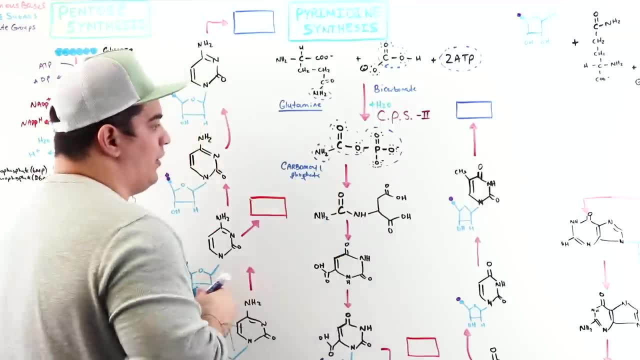 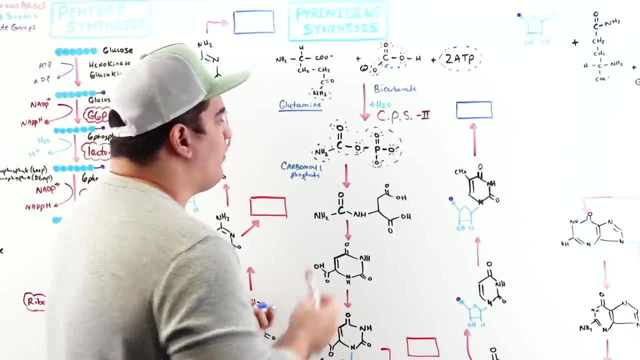 phosphate. Now what we're going to do is we're going to go even further. We're going to take this carbamoyl phosphate and we're going to add another molecule onto it, And in order for us to do that, we have to use a special enzyme, right? So what we're going to do next is we're going to add: 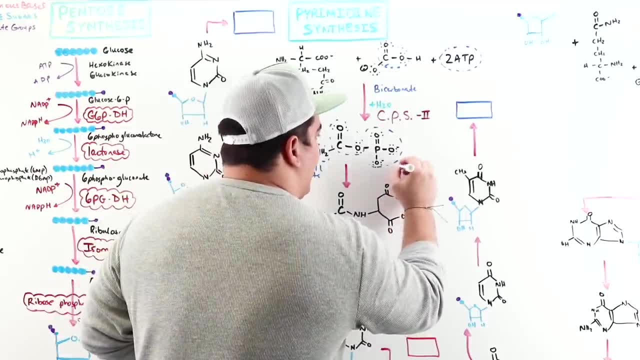 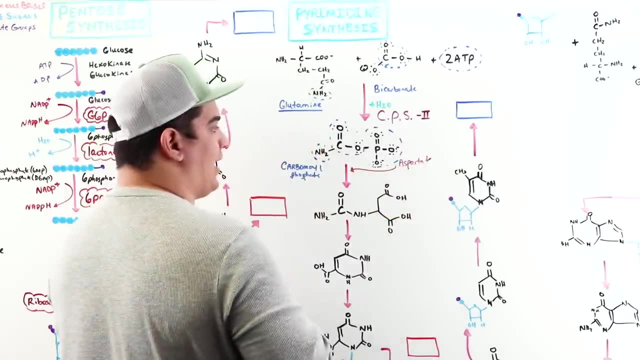 aspartate into this reaction. So what we're going to do is we're going to take here, we're going to have aspartate, Let's write him Out here. Aspartate is an amino acid and we're going to funnel him into this reaction. 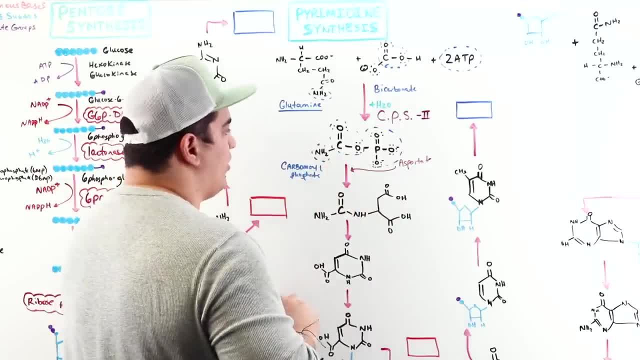 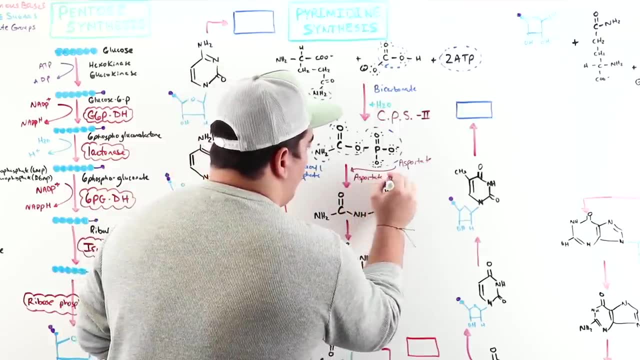 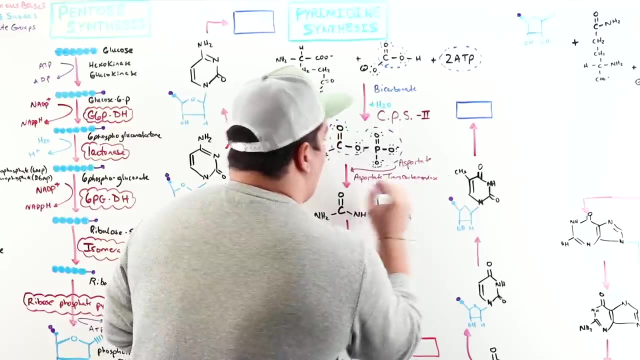 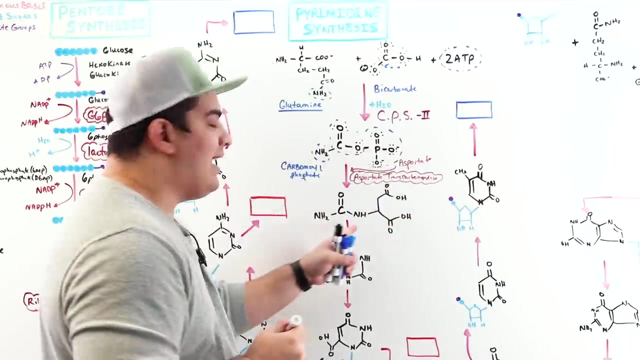 and add him onto the carbamoyl phosphate, And in order to do that, we need a particular enzyme, And this enzyme is called aspartate transcarbamoylase, And aspartate transcarbamoylase will combine this aspartate with the carbamoyl phosphate, and 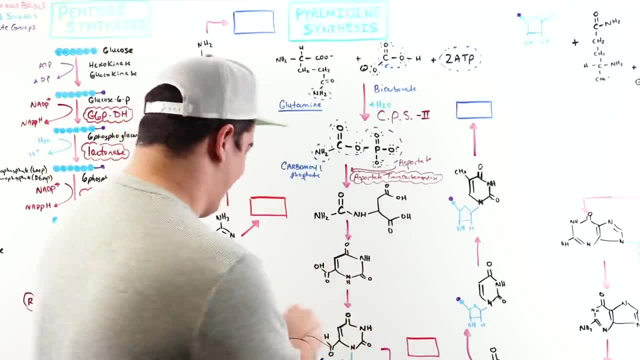 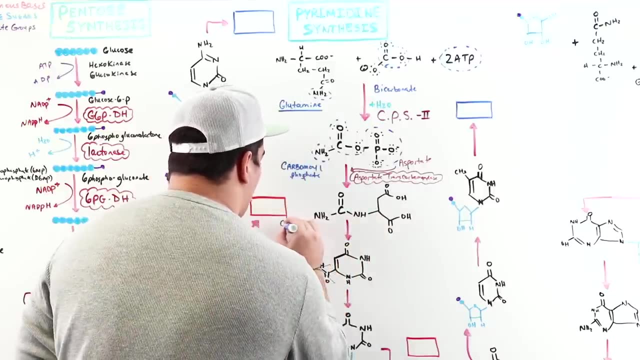 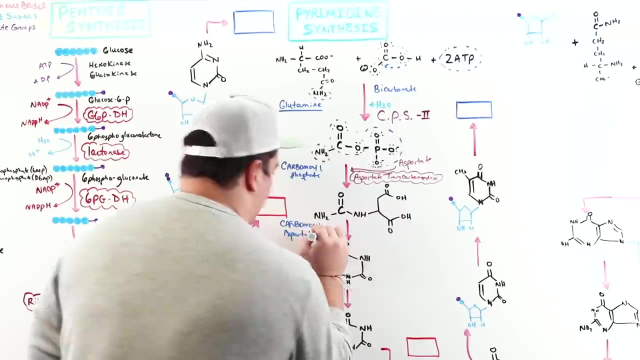 now make carbamoyl aspartate. All right, So now we're going to make this new molecule, And this new molecule here is called carbamoyl aspartate. Okay, Now, the next thing we're going to do is: 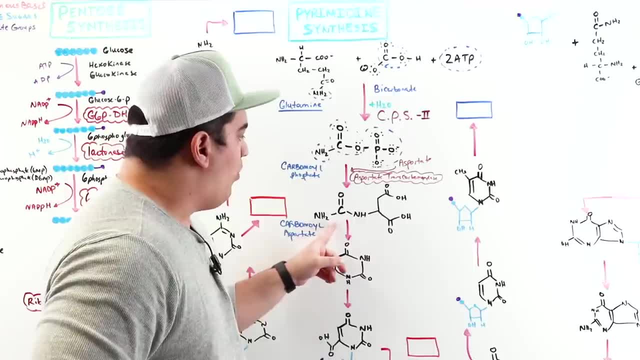 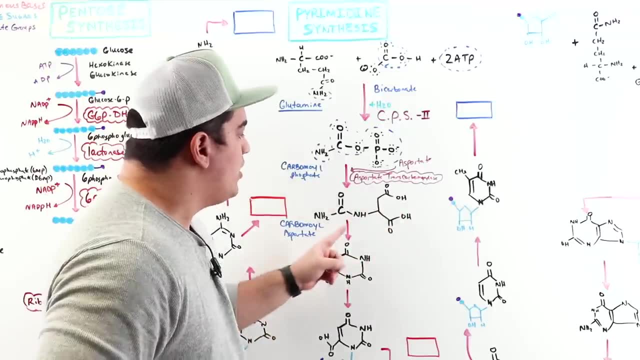 is we're going to take this carbamoyl aspartate And what I want to do is is I want to dehydrate this, So I'm going to kind of Uh, help to basically make a ring structure here. So I'm going to use an enzyme here. 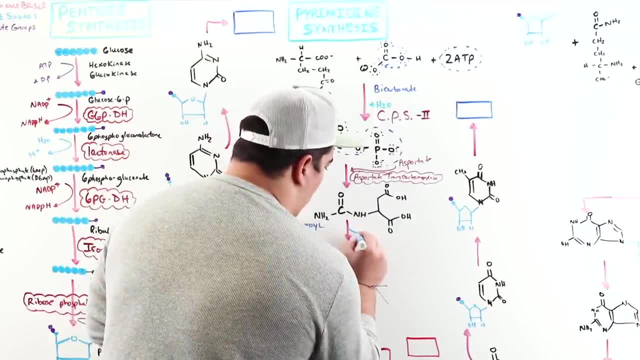 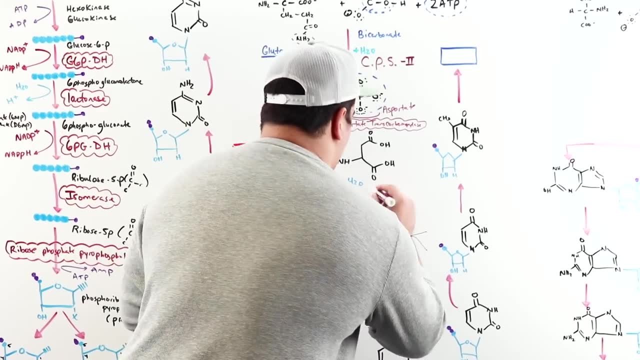 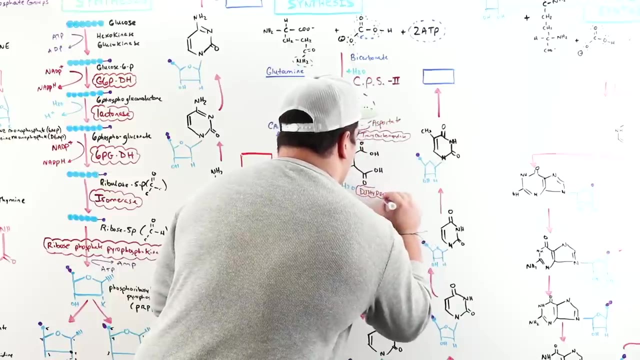 and I'm going to dehydrate this structure. So I'm going to pull some water off of this And by doing that I use this enzyme called dihydratase. So there's an enzyme here called dihydrotase And the dihydrotase is basically going to help in this reaction. 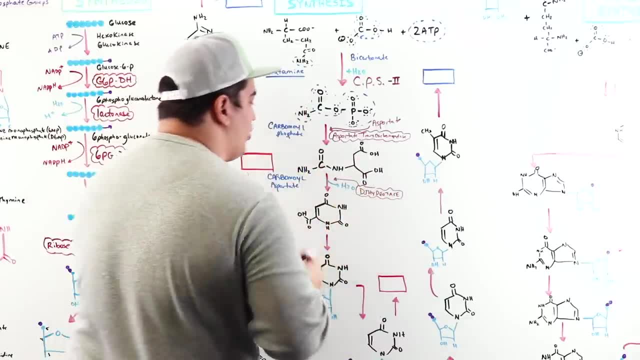 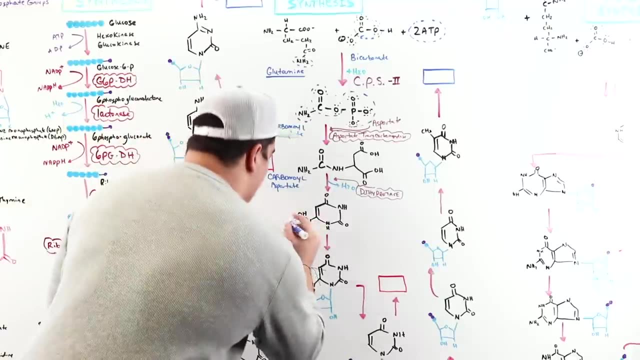 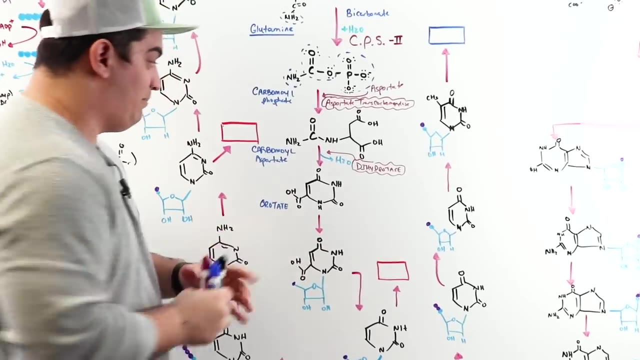 to help close this carbamoyl aspartate and turn it into a ring structure. This ringed structure is now called orotate, So this molecule is called oro tate. Now orotate is beginning to look like some of my actual 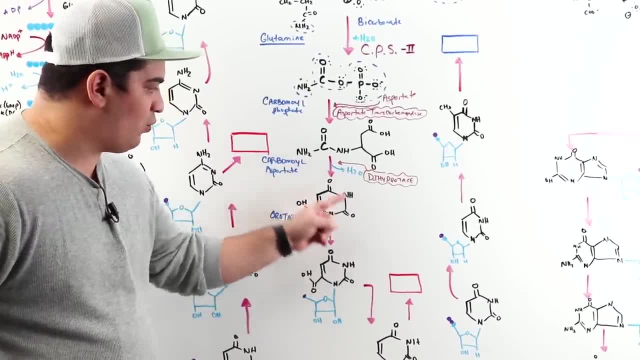 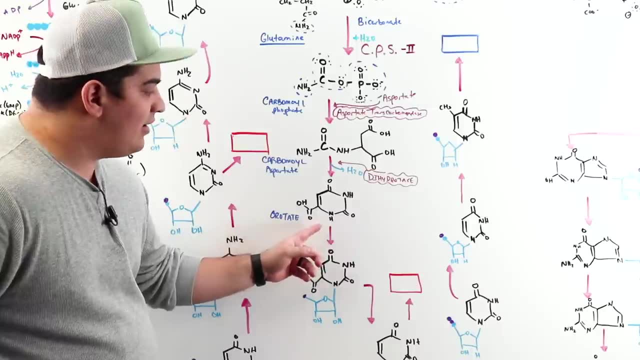 primidine structures. right, Oh, it's a six ring structure. It's a nice ring here. Oh, we're getting pretty darn close. Well, guess what? Remember that panto sugars that we were synthesizing. Let's go ahead and add it onto the Orotate. 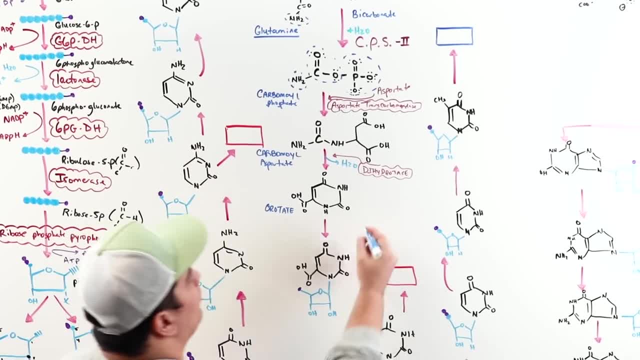 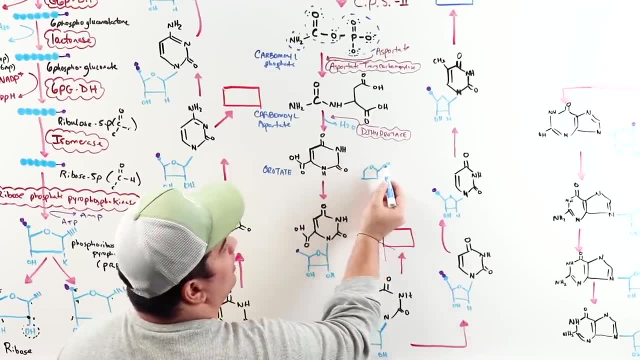 So now what I'm going to do is I'm going to take that molecule. You guys remember that molecule. We had that PRPP right. So here it is. I'm going to have here. this is the component which is going to bind to the nitrogenous product. 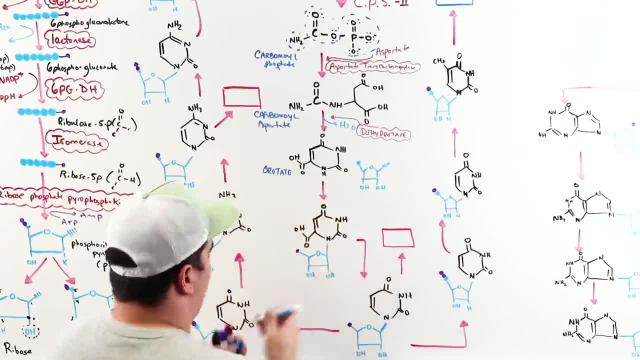 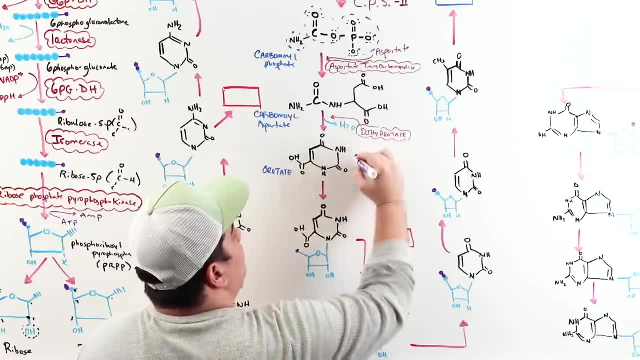 Here's going to be my CH2.. Here we'll put an OH. We'll put an OH here because we'll just assume that this is a ribosugar here And remember we had the two phosphates on it, And what I'm going to do is I'm going to add this bad boy into this reaction. 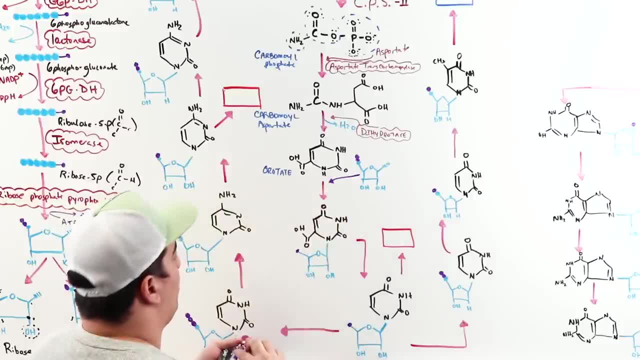 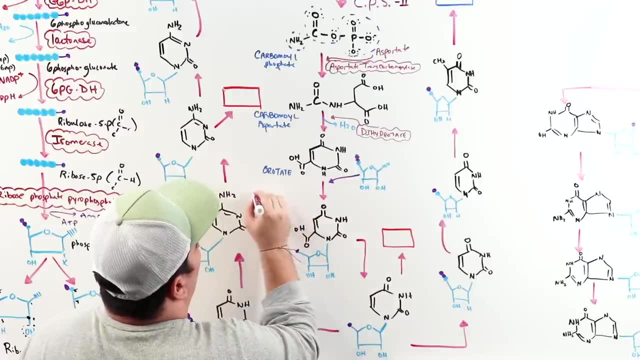 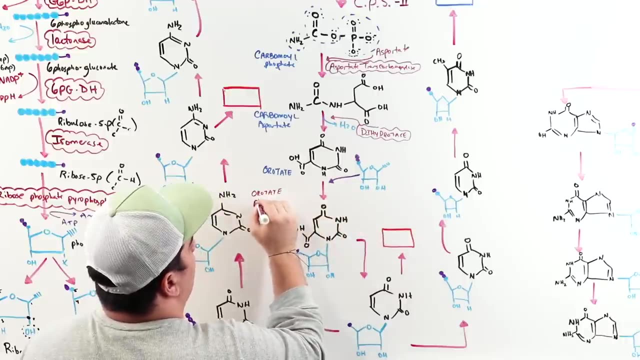 Well, in order to add this on, I obviously need an enzyme. Let's go ahead and make an enzyme. that is very difficult to say, Well, that's what they love to do, right? So the next enzyme is called orotate phosphoribosyl- phosphoribosyltransferase. 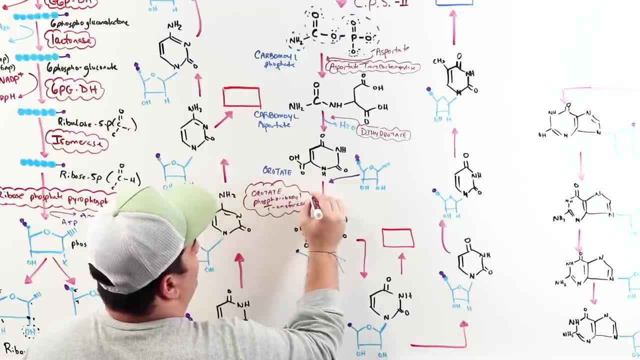 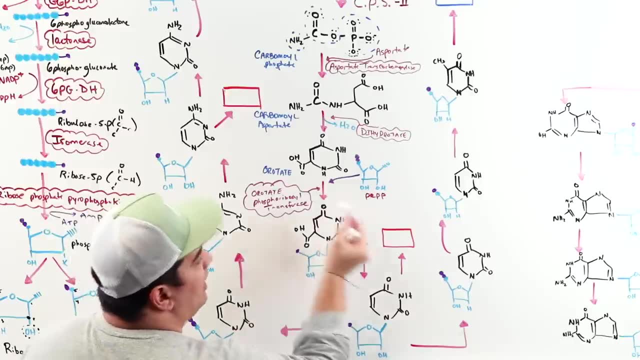 It's not so bad. but you know, that's the name of the enzyme that's going to catalyze this step And it's going to add this PRPP to the orotate and make this new molecule. What is the name of this new molecule? 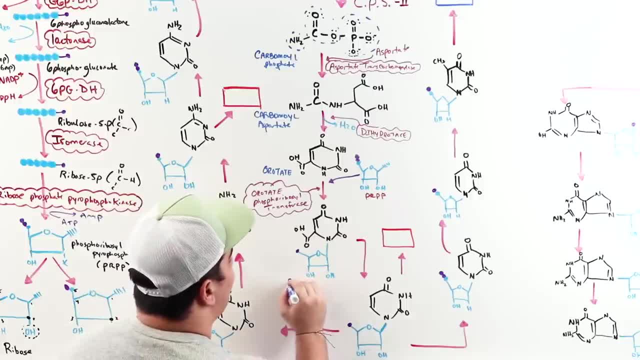 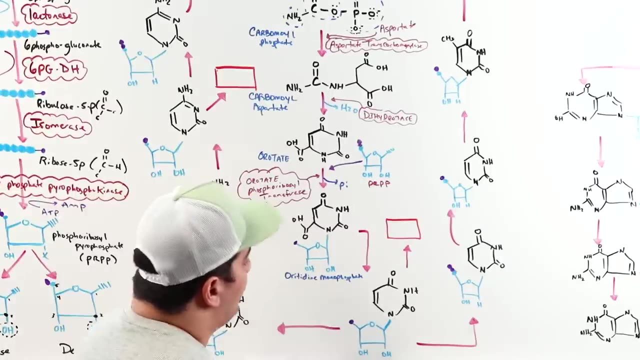 This new molecule is called oritidine monophosphate, So in this process we popped off also a phosphate group, because now we only have one phosphate. All right, so oritidine monophosphate is commonly abbreviated. right, We abbreviate it as O-M-P. 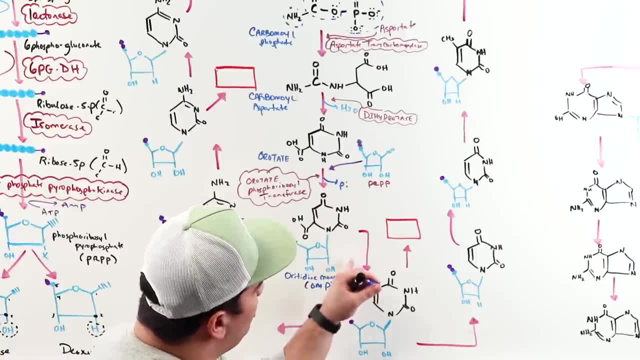 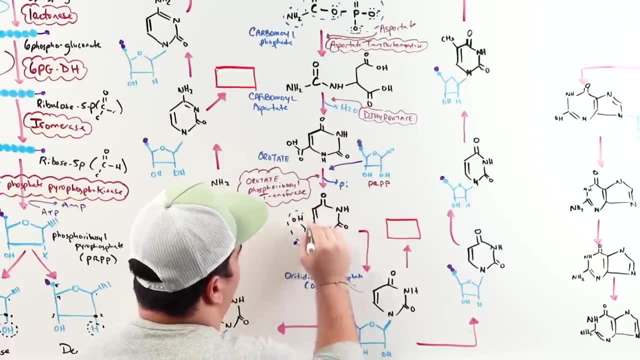 Well, what I'm going to do now is I'm going to use an enzyme And what I'm going to do is I'm going to chop off that, this carboxyl group here. So I'm going to chop this off and I'm going to release this out as CO2.. 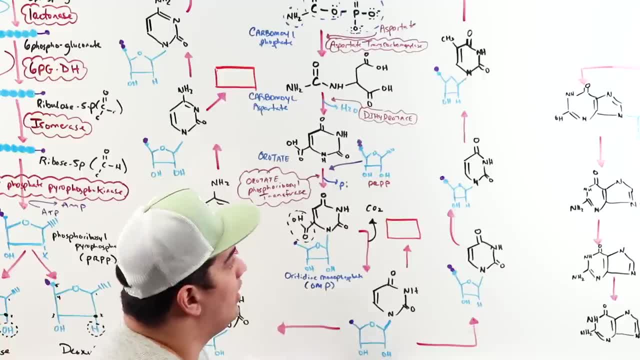 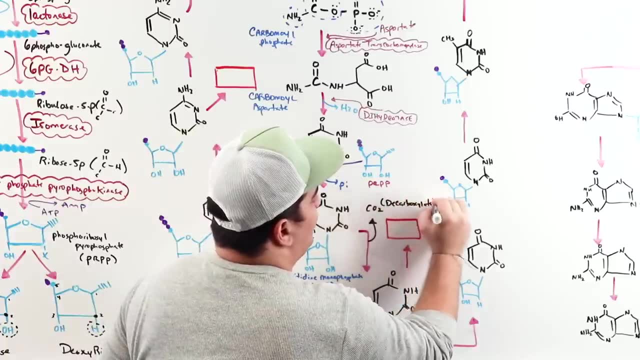 What kind of reaction is that called whenever you pop a CO2 molecule off something? It's called a decarboxylation reaction, right? So we're going to decarboxylate this puppy Now, whenever we decarboxylate it. 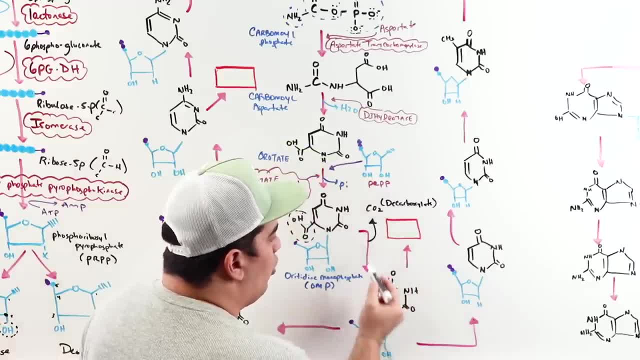 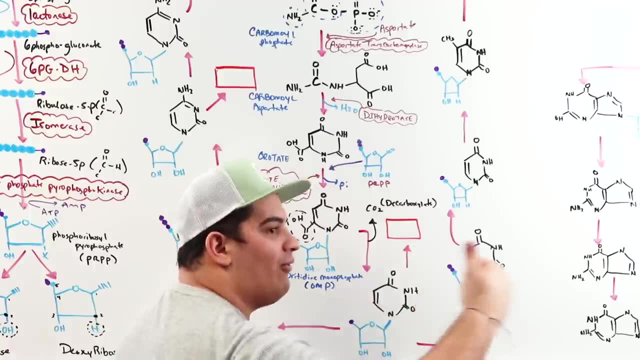 we're going to lose that molecule, that CO2 molecule. We're going to use an enzyme to help to convert O-M-P into the next molecule called U-M-P or oritidine monophosphate. Hey, that was one of the nucleotides. 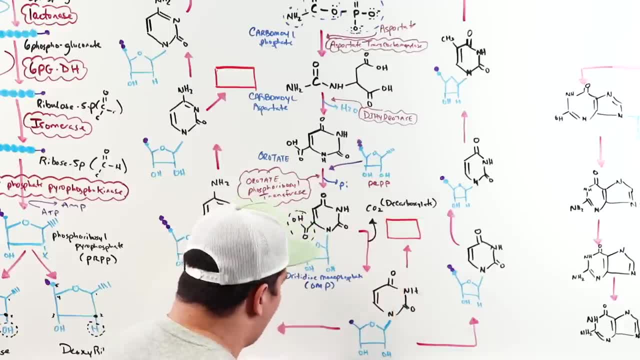 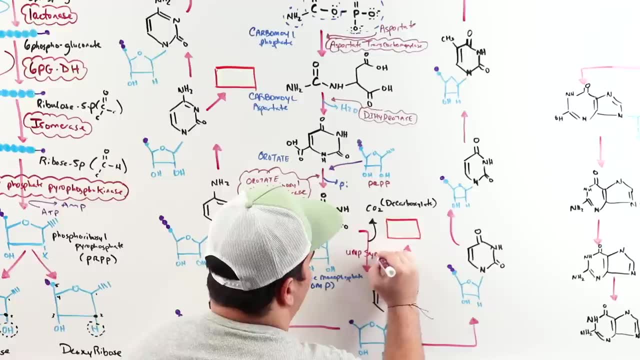 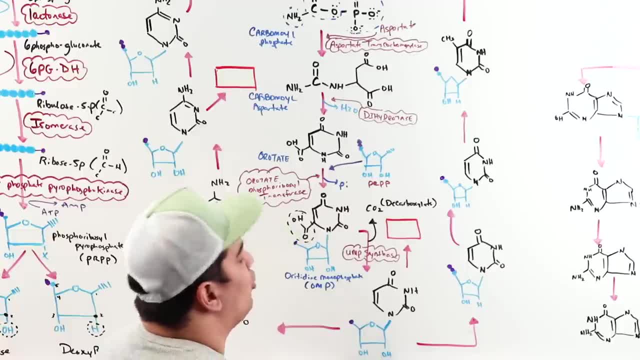 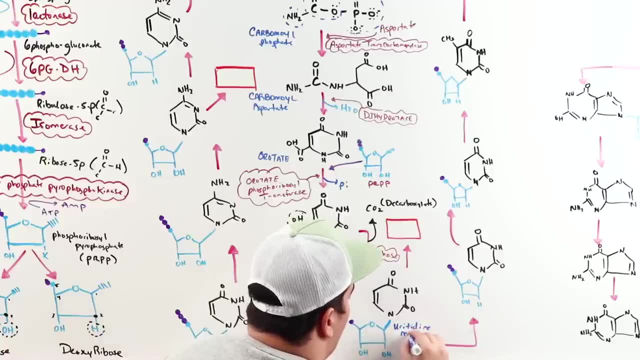 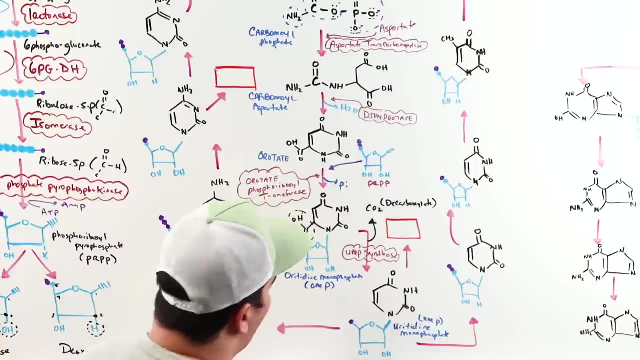 Pull a CO2 molecule off of it and convert it into uritidine monophosphate. So this is called uritidine monophosphate, which we can abbreviate as U-M-P. Now what we can do with this U-M-P is we can use this to go and synthesize another molecule. 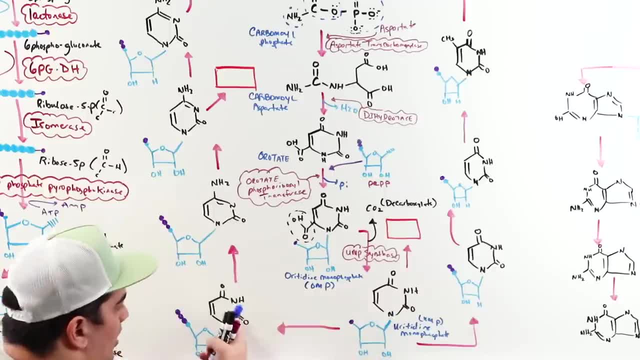 Let's take a look here. Let's make sense of this. Let's look at these two molecules I have here: U-M-P. Well, they pretty much look the same. What's the only difference? Oh, I added two phosphates onto here. 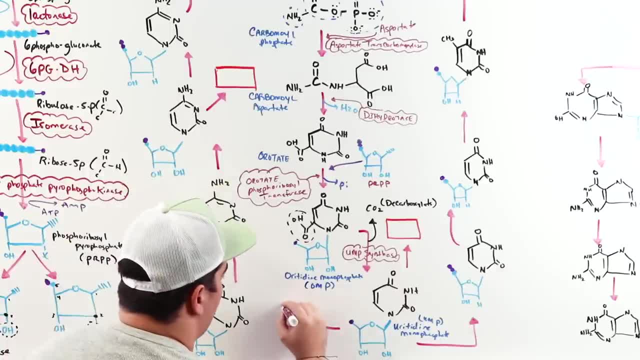 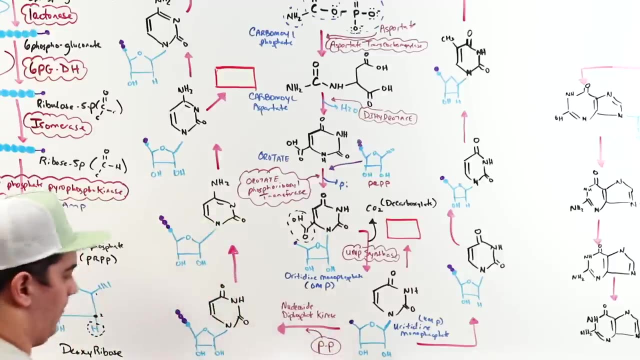 Well, there's an enzyme called nucleoside diphosphate kinase, And what it does is it adds a pyrophosphate group onto this molecule, which is two phosphates. Okay, If I add two phosphates now, look what I have. 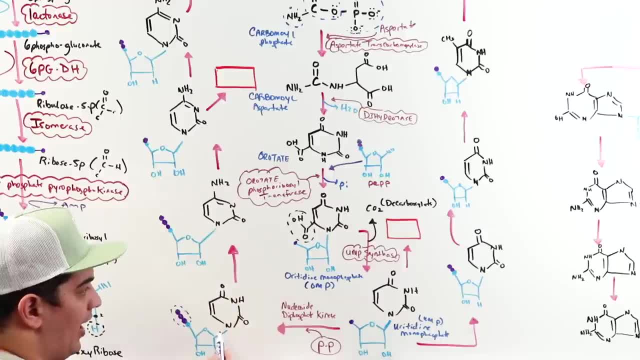 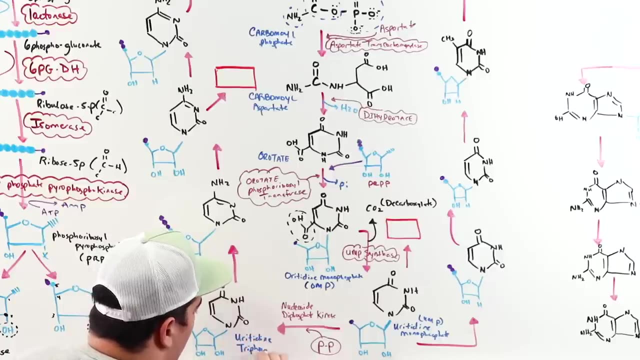 I have three phosphates. It's still uritidine, okay in this situation, But it's not monophosphate, It is triphosphate. So now we have what's called uritidine triphosphate, which can be abbreviated as U-T-P. 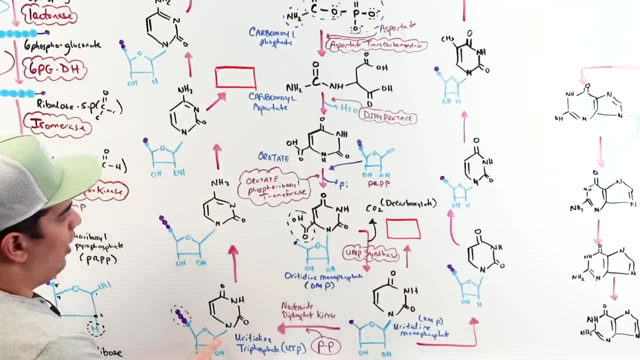 Look at the next step. Okay, Now, what I'm going to do is I'm going to take this uritidine. I'm going to take this uritidine triphosphate, and let's look and see what happened here. I have a carbonyl group here, bound to a nitrogen, and I come up here and now it's an amine. 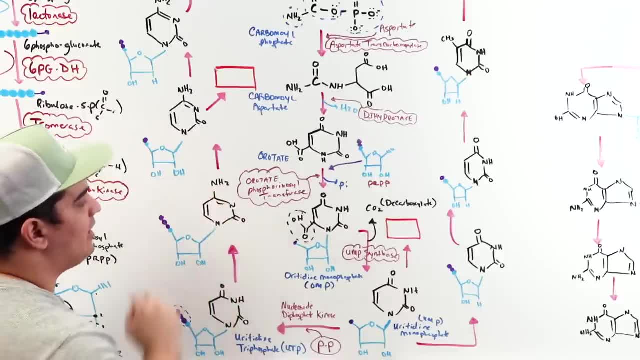 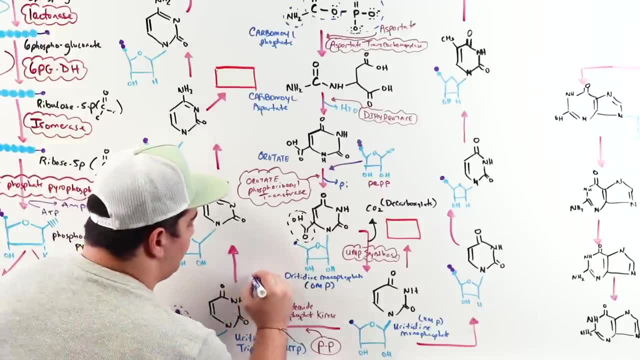 So I must have lost that carbonyl group somewhere in there and replaced it with an amine group. Technically, any time you do that, you're going to be utilizing glutamine. So somewhere along this reaction we must have added glutamine. 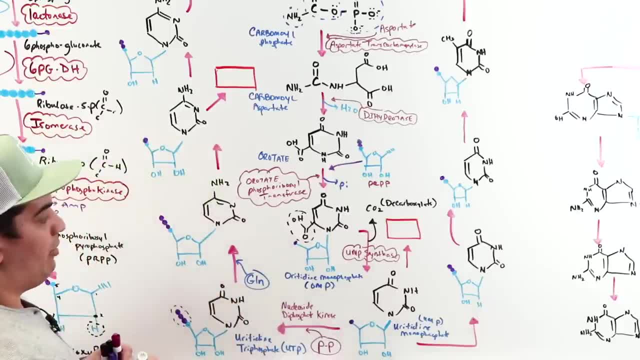 We'll just mark this as GLN And we use the amine group in that process, But when we did this, we still have the three phosphates, so that's still the same. Okay, Okay, Okay, Okay Okay. 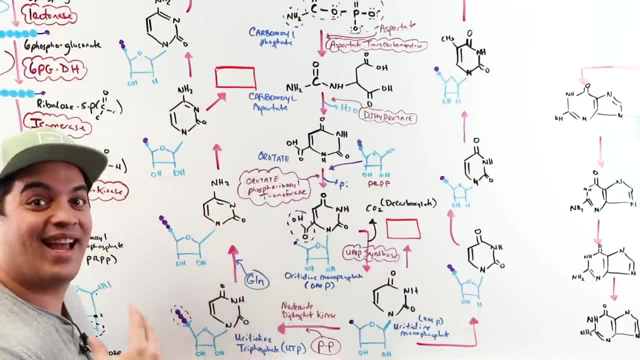 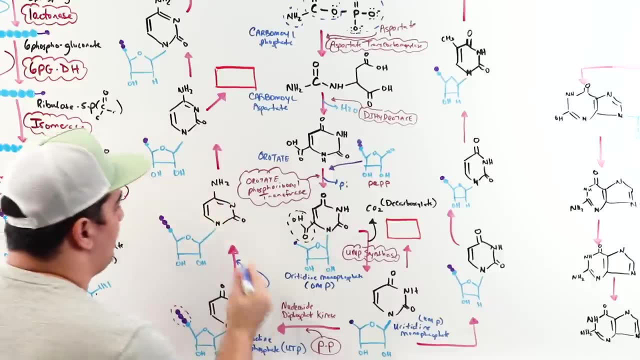 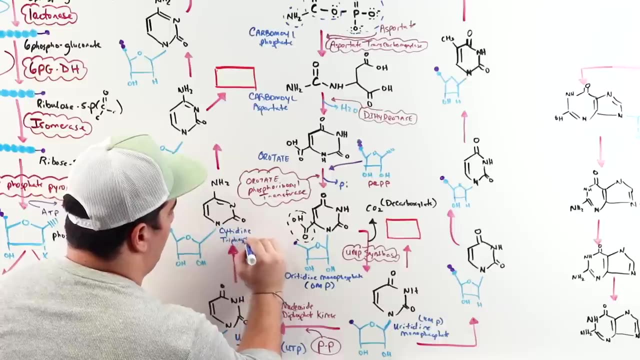 Okay, Okay, If we change it, this is now cytidine triphosphate. Go back to your structures and remember: this is cytidine triphosphate. So now we have cytidine triphosphate, which is abbreviated CTP. 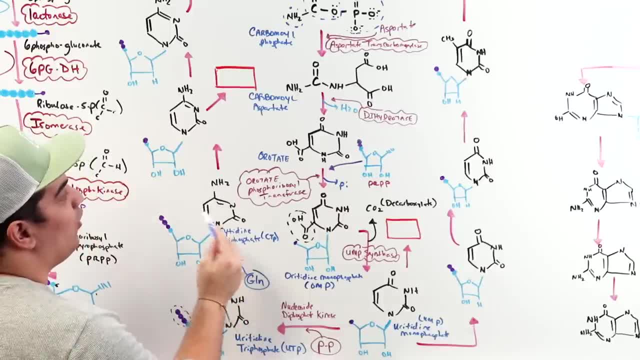 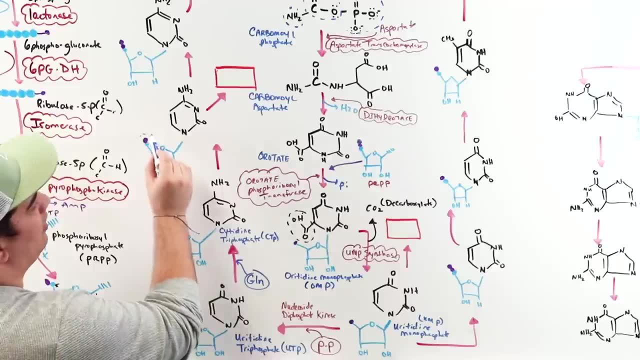 Now CTP is going to need to do what? Okay, Let's go to the next step. If we go to the next step, what happened? This was three phosphates. What do we have now? One phosphate. What does that mean? 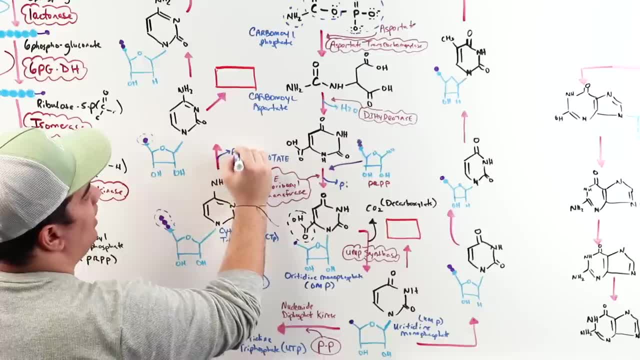 Somewhere along this reaction I popped off a pyrophosphate. Well, you can use pyrophosphates in a ton of different pathways And this might help to be able to convert a reaction, some other bio energetic process, and add that on there. 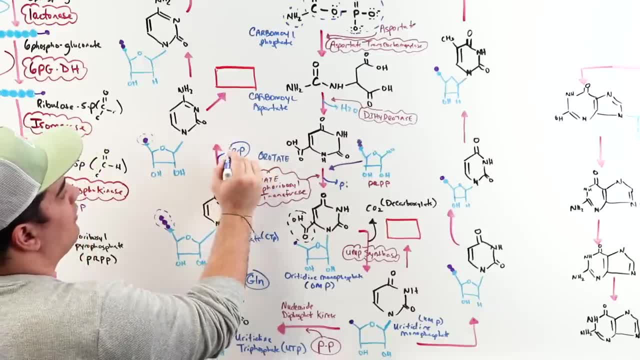 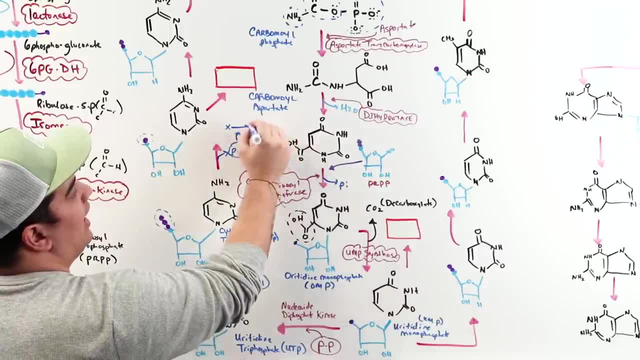 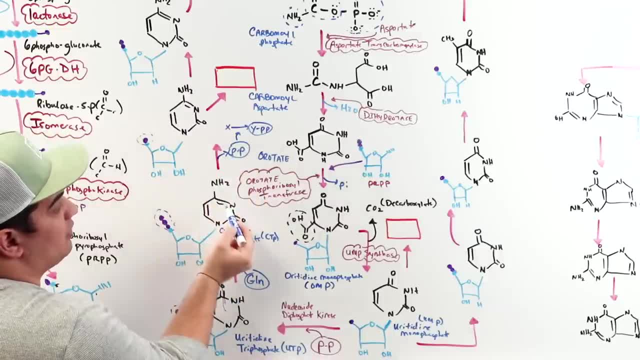 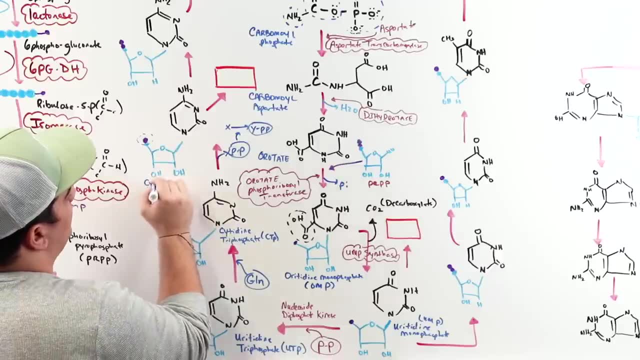 So this is now CTP, CTP, Cop that pyrophosphate off, and now this is no longer called CTP right, Which was this one previously. It's now CMP, which is referred to as cytosine cytidine. 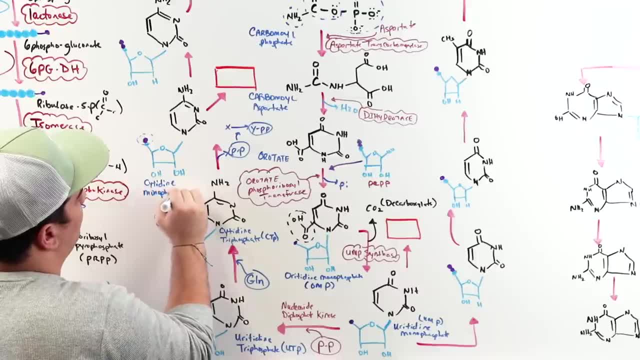 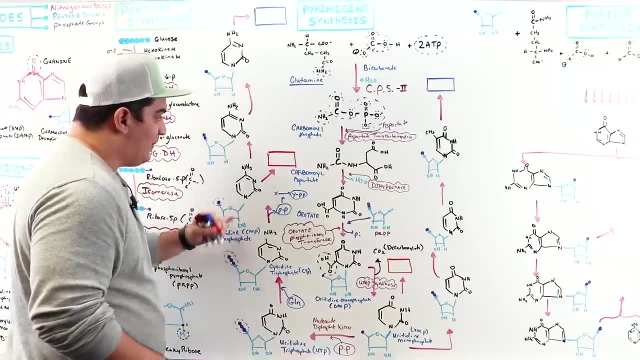 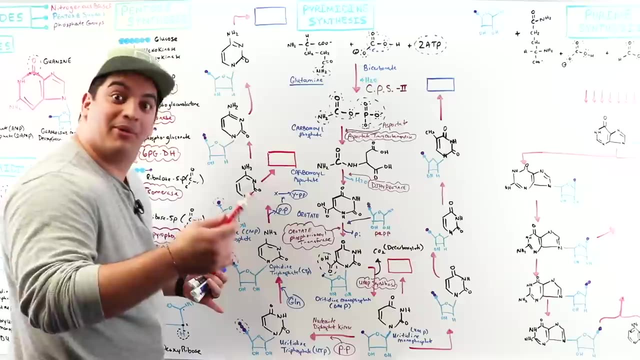 Sorry, cytidine monophosphate, OK, which is abbreviated CMP. All right, So now we technically can have CMP right To be utilized to make RNA nucleotides, because, again, cytidine is a component not just of RNA but also of DNA, but we don't have a deoxy in front of this. So 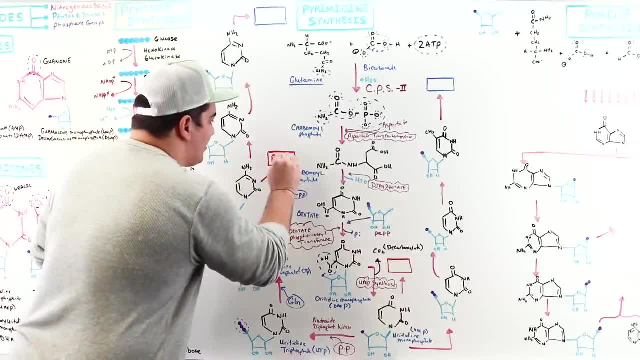 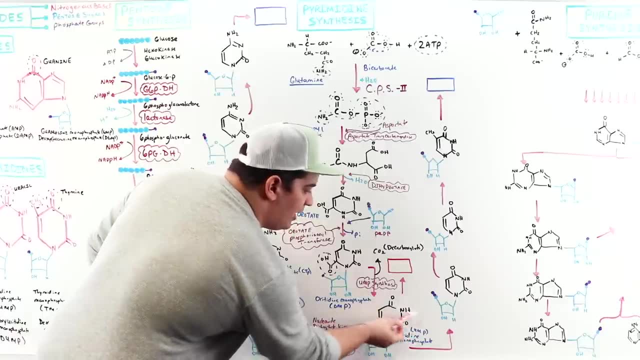 it's going to be used to make RNA. Go back a couple steps over here, where we had UMP. Remember? here we had uritidine monophosphate. What did we say UMP can be utilized for, And again, there's no D in front of it, So we're not going to be using it just yet. It's not for that thymine process. 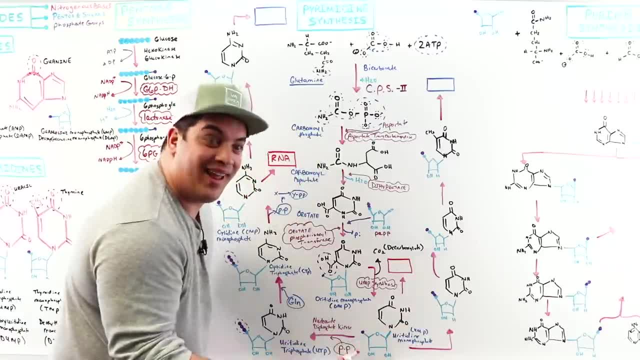 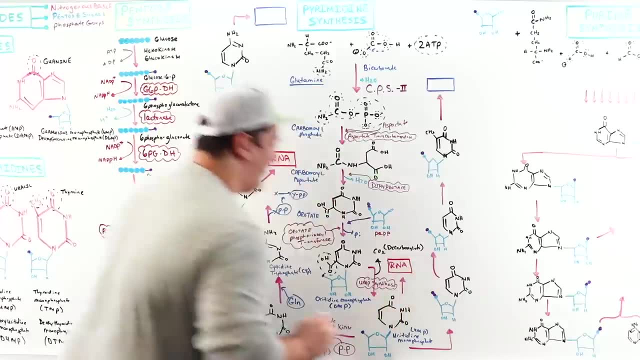 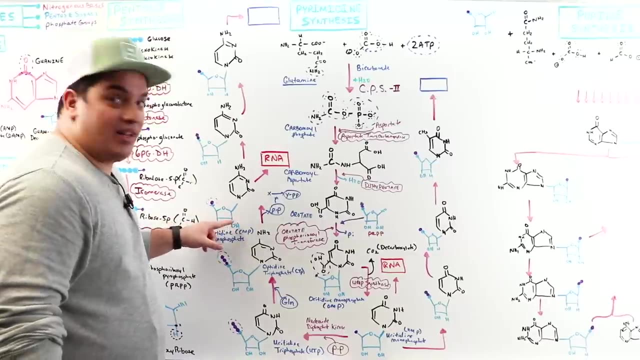 We said that uracil is commonly involved in RNA, So I could take UMP and utilize this to make RNA. Isn't that cool? All right, Now let's keep going, because cytidine monophosphate- we want to make sure that this is utilized to make DNA. So how do we do that? So we take the. 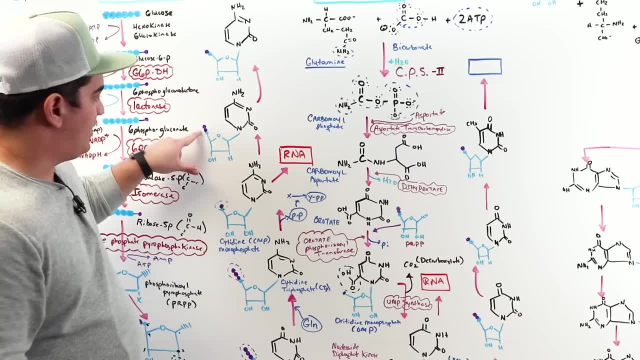 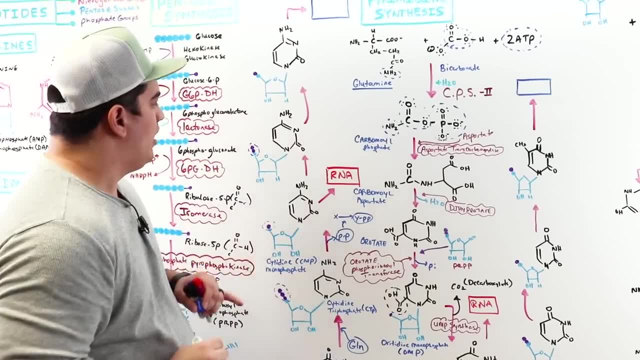 cytidine monophosphate. which is this molecule here? and let's look at the next step. What happened in the next step? Well, we only have one phosphate here and we added on a phosphate here. Okay, Look what else happened. guys, We have the hydroxyl group. 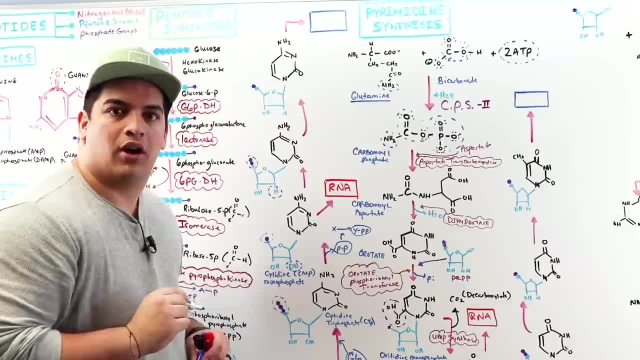 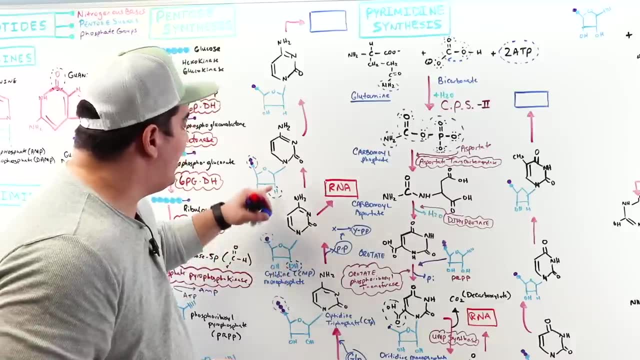 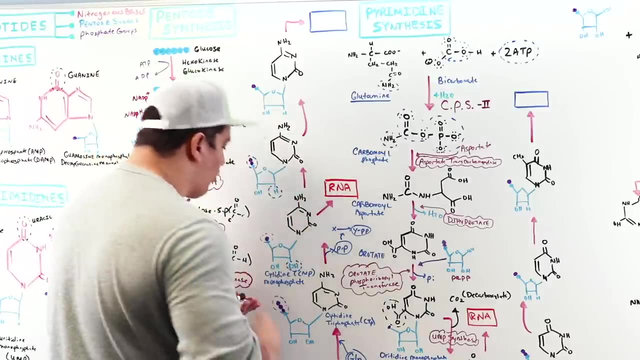 On the second carbon hydrogen. on the second carbon. What happened here, Zach? did you make a mistake? No, This is actually converting this ribonucleotide into a deoxyribonucleotide. So this enzyme that catalyzes this step is called a ribonucleotide reductase. So this is called. 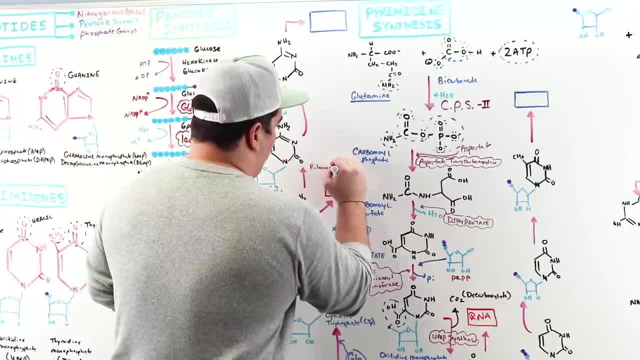 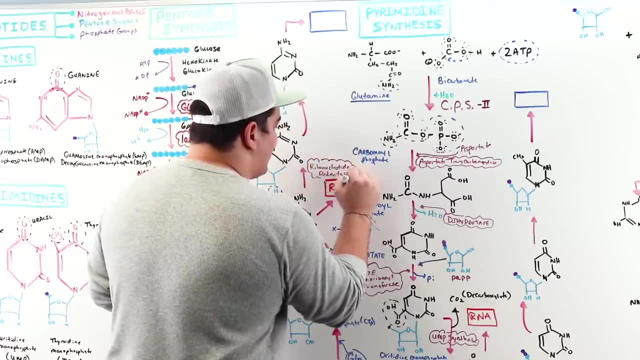 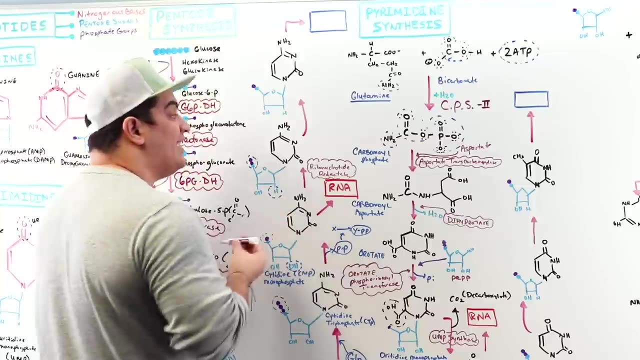 the enzyme that catalyzes this is called ribonucleotide reductase. What this does is it does two things: It adds a phosphate group onto this sugar here, and it converts a ribose sugar into a deoxyribose. So now this is no longer. 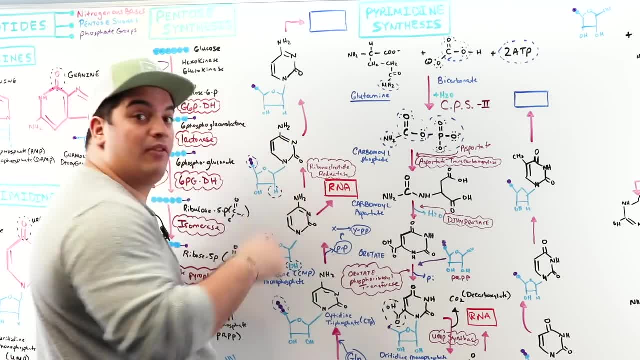 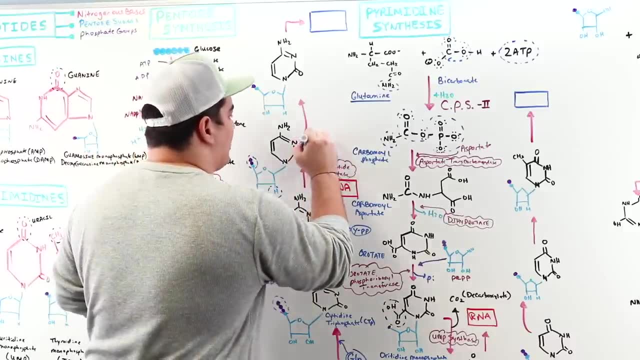 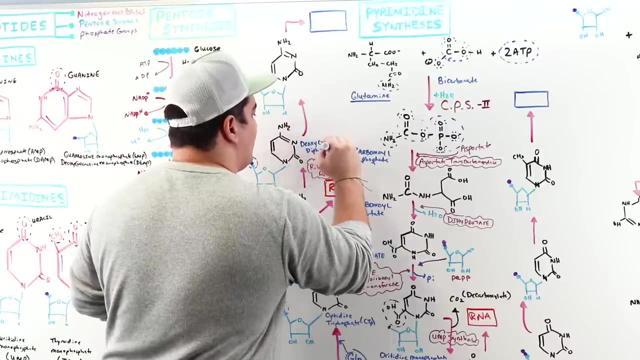 CMP. it's CDP, but it has a D in front of it because it's a deoxyribose. So we're going to call this one deoxycytidine, diphylocytosidine Diphyphosphate, or abbreviated DCDP. 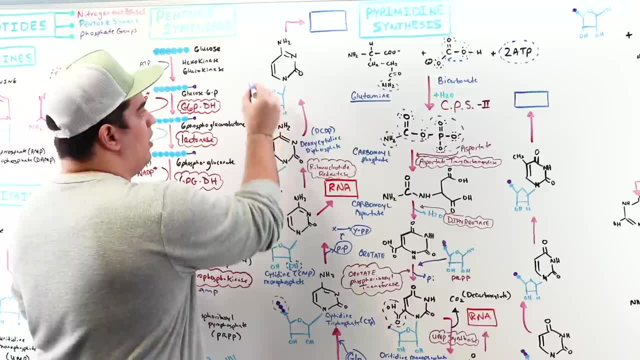 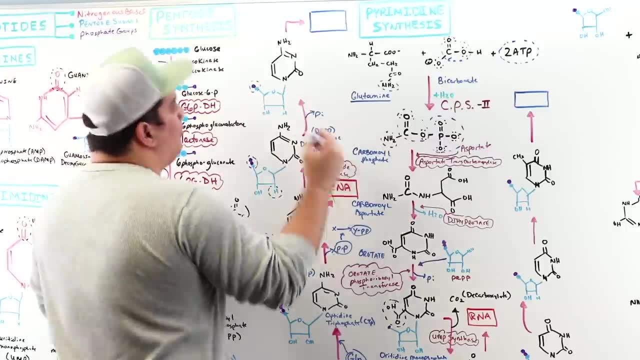 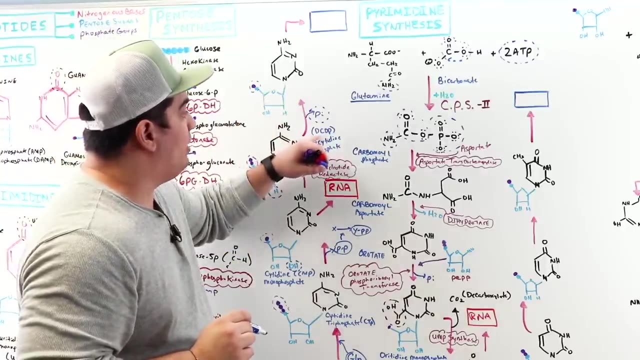 Now what happens in the next step? Next step: I have two phosphate groups. Oh, I only have one, but nothing else changed. So all I did was pop off a phosphate. And when I pop off that phosphate, what am I going to do now? Now I have one phosphate which is going to be considered to be. 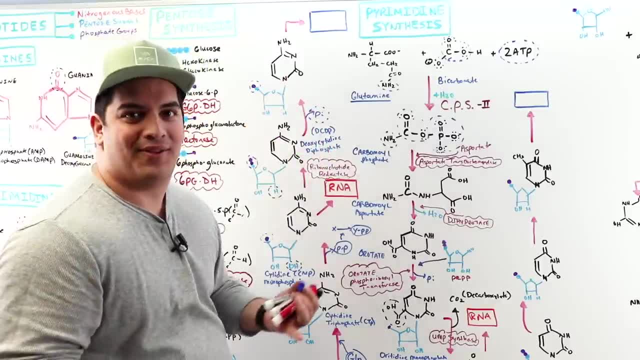 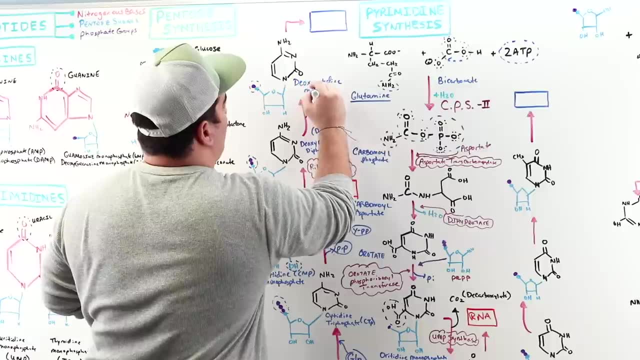 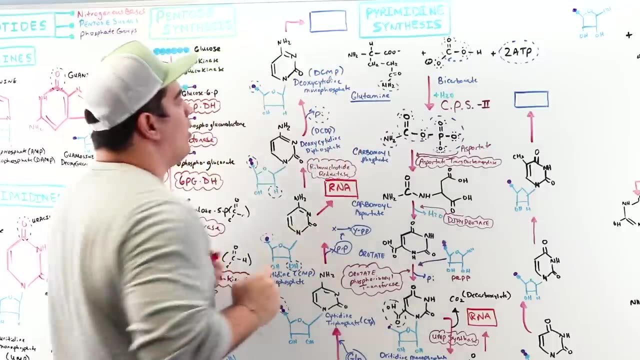 deoxycytidine monophosphate. So now this new molecule is called deoxycytidine monophosphate. Oh my gosh, this is so cool, right? So DCMP- What did I say? Cytosine is a nitrogenous base involved in DNA and in RNA. 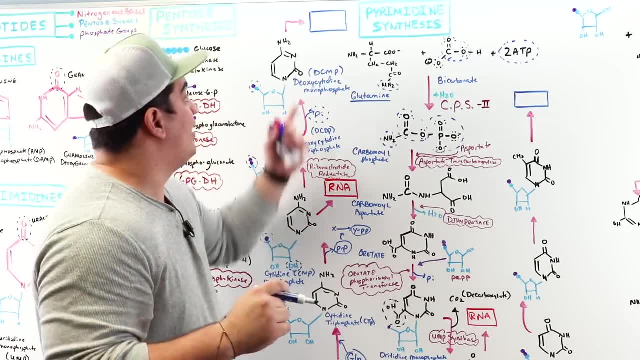 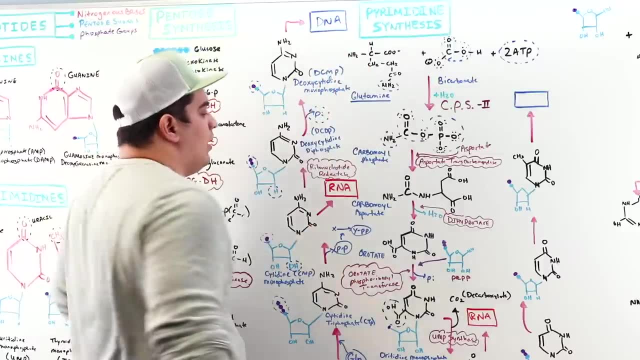 But in order for it to be in DNA, it has to have that D in front of it. Can I use this now to make DNA? Yes, And so we can incorporate this into making DNA. Okay, Okay, Okay, Okay Okay. 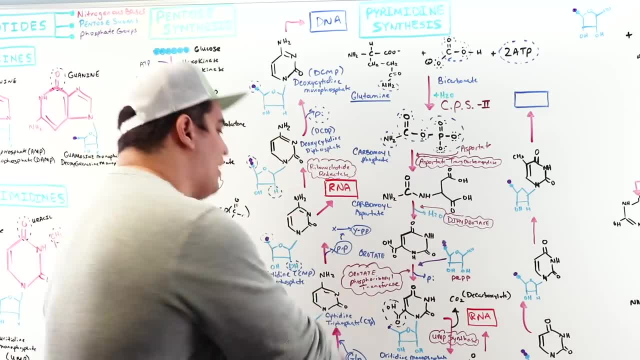 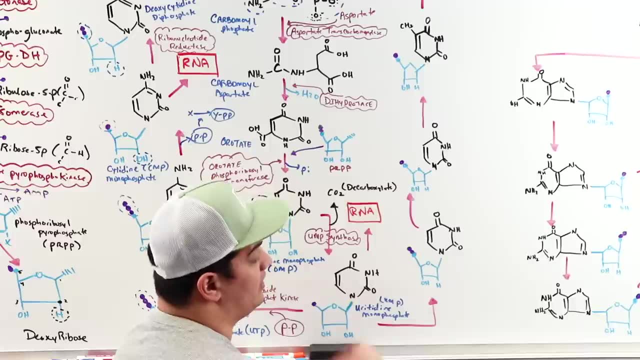 Hang in there, guys. We're almost done with pyrimidine synthesis. Let's go back down to the bottom and work our way back up, All right. So now let's come back here. We took the UMP and we made the CMP as well as the DCMP right? So we made those components for RNA. 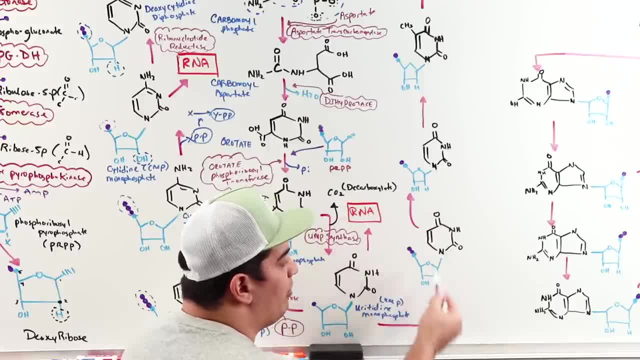 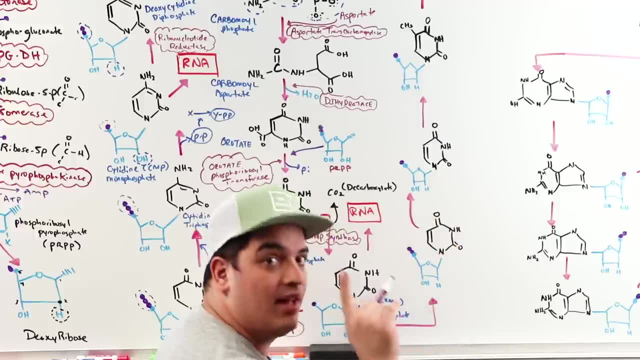 and DNA and we made UMP to make RNA. but there was one other pyrimidine. What was it? Thymine, right, Which technically we're going to make thymidine and deoxythymidine, because thymine is only used in DNA, It's not used in RNA. So in order for us to do that, we 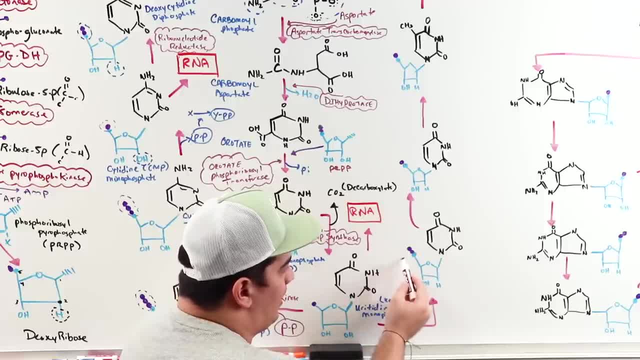 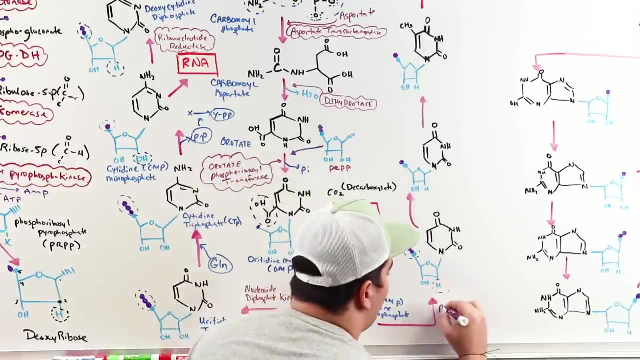 take this uritidine monophosphate and look what happened. You guys, this should sound familiar. We had one phosphate here. Now we have two phosphates here. Look guys, hydroxyl group here, hydrogen group here. I remember that reaction. What was that? It was the ribonucleotide. 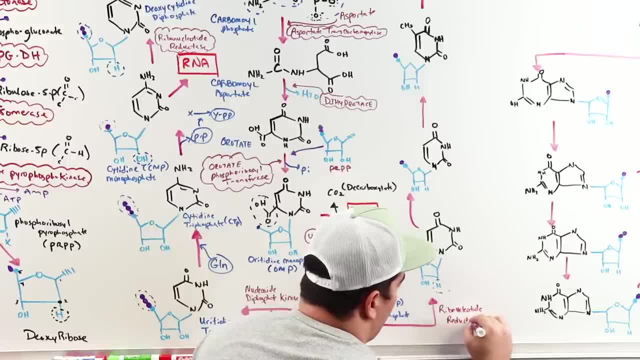 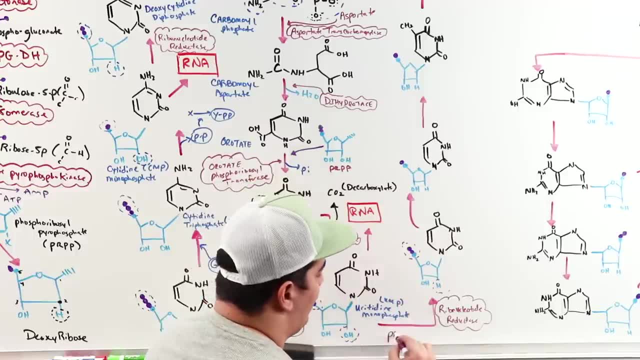 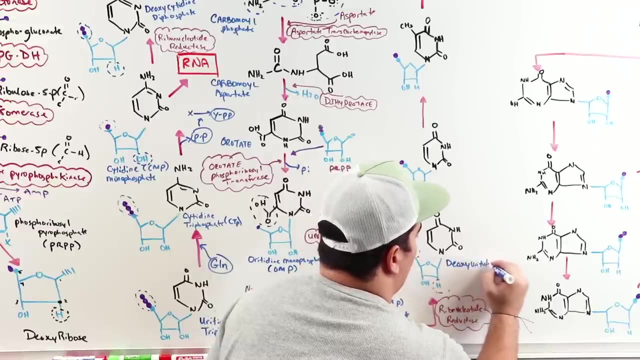 reductase enzyme. And what that enzyme did is it converted this ribose sugar into a deoxyribose sugar and added a phosphate. So we added a phosphate into this reaction. So this is now deoxyuritidine diphosphate, because we have two of those phosphates on there, So we can abbreviate. 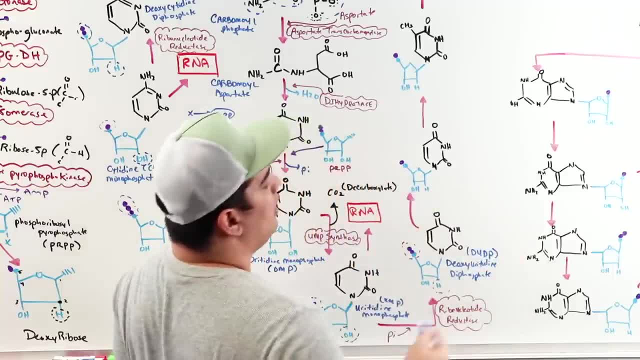 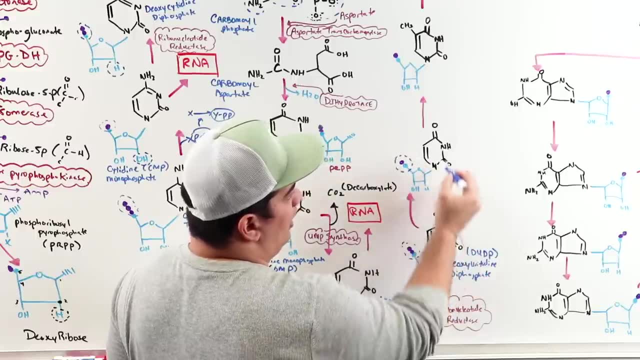 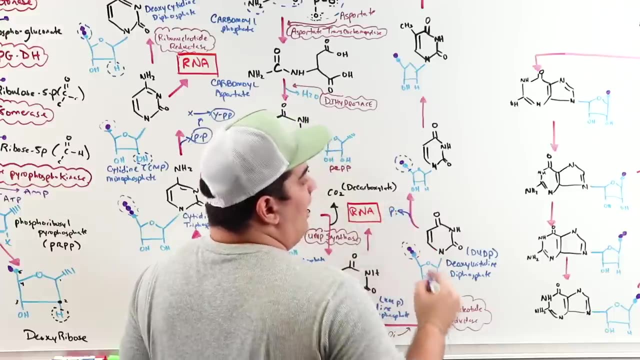 that D U D P. Look at the next step. We have two phosphates here We go to one phosphate. nothing changes in the pentose and nothing changes in the nitrogenous base. So all I did is I released a phosphate off in this pat process. If I release a phosphate off in that process now, this is just 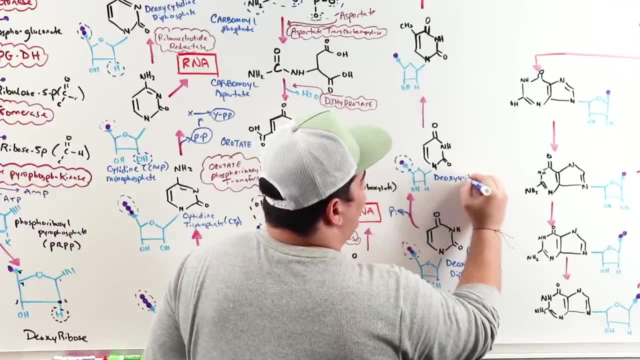 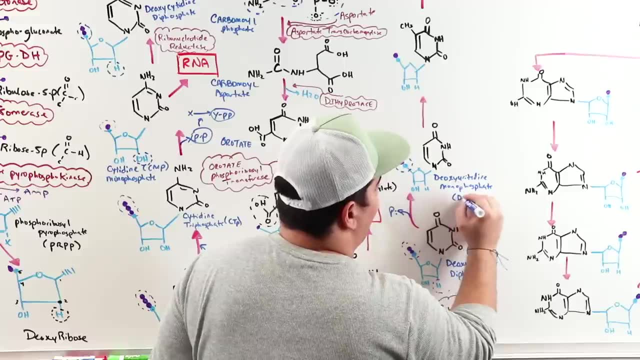 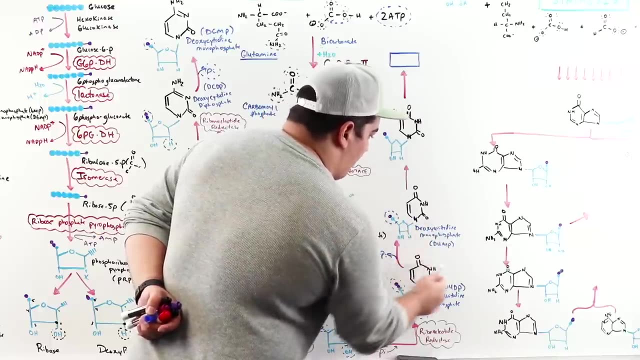 called deoxyuritidine monophosphate, which we can abbreviate D U M P. Now we come up. Now we take this deoxyuritidine monophosphate. Look at the next step. All right, There's still one phosphate group. 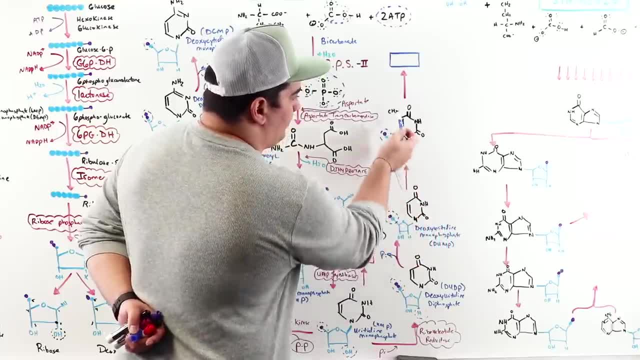 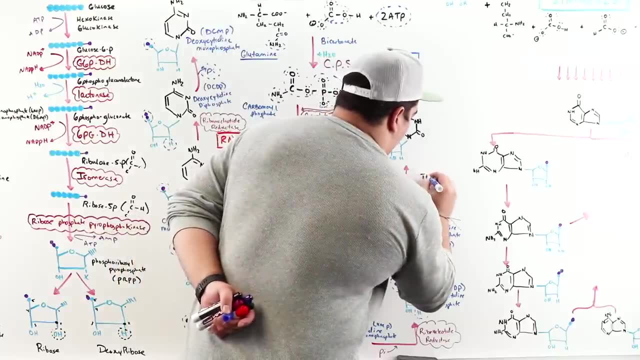 that hasn't changed. but holy crap, Look what happened. Now we take this deoxyuritidine monophosphate. what happened here? I added something. I added a methyl group and we're going to add this in the form of tetrahydrofolate. So tetrahydrofolate will be involved in this process and we're going to add. 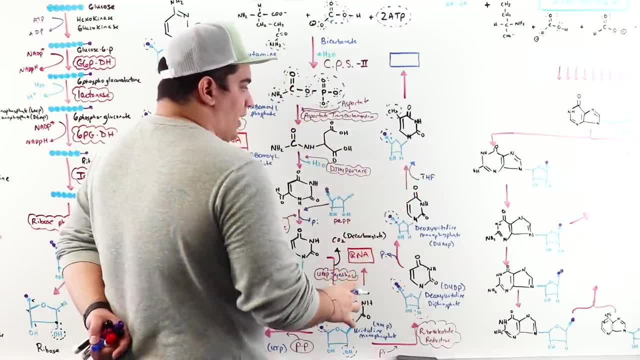 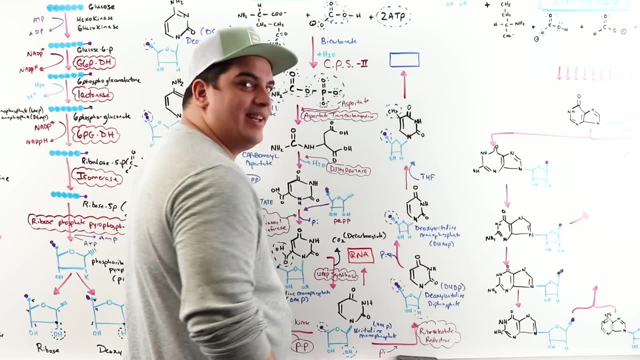 that son of a gun in there. When we add the tetrahydrofolate in here, we have to use a particular enzyme in this process and we're making a new nucleotide. Guess what this new nucleotide is? Thymidine. right, In this case, we're going to be making a specific type. We'll get the name. 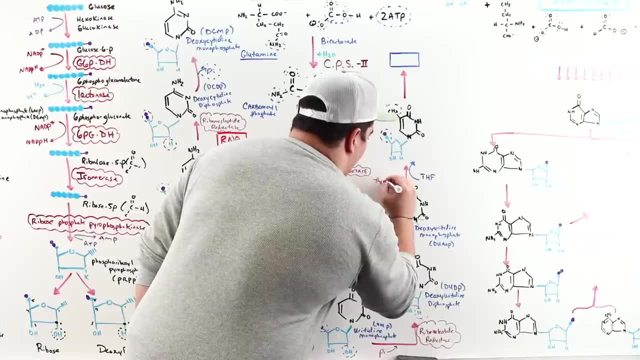 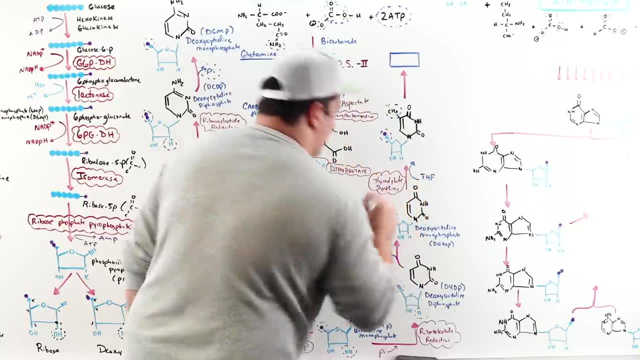 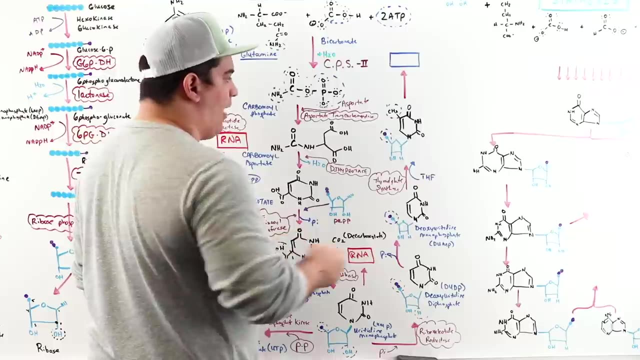 here in just a second. but this enzyme is called thymidylate synthase- Thank goodness for this easy name right- And we're going to use a tetrahydrofolate type of derivative and add on this whole methyl group here. Now this new molecule is going to be a thymidine type of molecule. Is it deoxy? Yes, 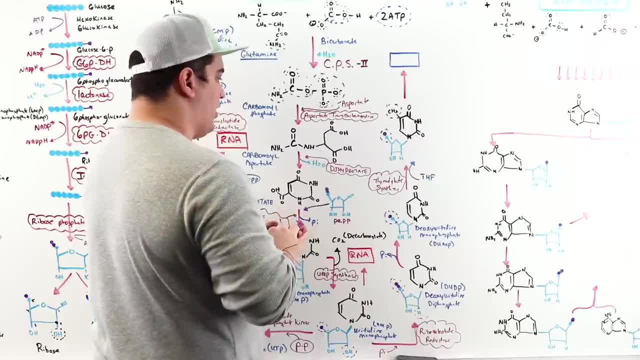 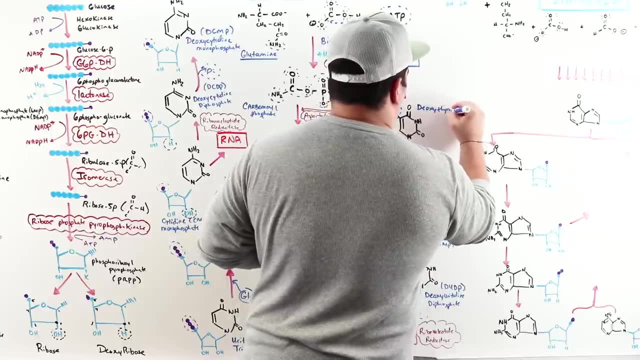 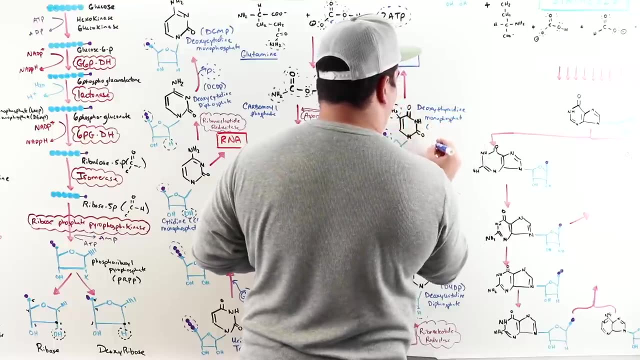 Is it thymidine? Yes, How many phosphates? One? Let's go through the name, get that nomenclature down. This is deoxythymidine monophosphate, which we can annotate as D-T-M-P. Thymidine is only used to. 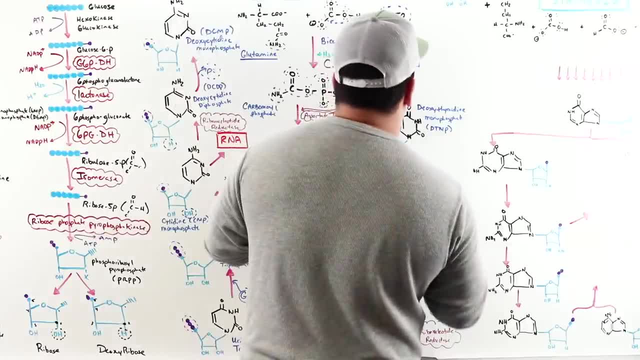 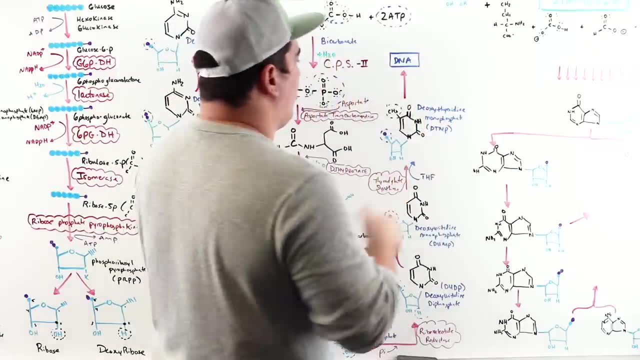 make DNA. So if we use this, we can incorporate it into our DNA structure. So we've just synthesized all of our pyrimidines. All right guys. so we went through the behemoth of the pyrimidine synthesis pathway. The next thing that we have to do is tackle the 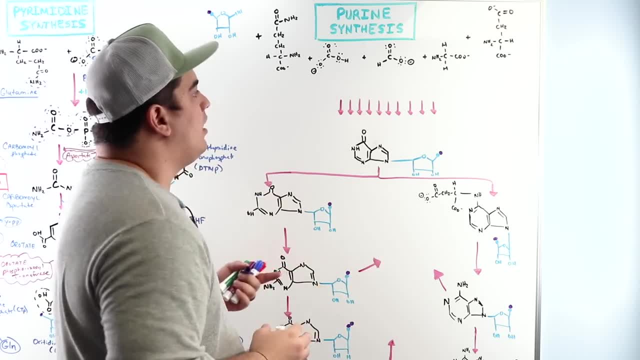 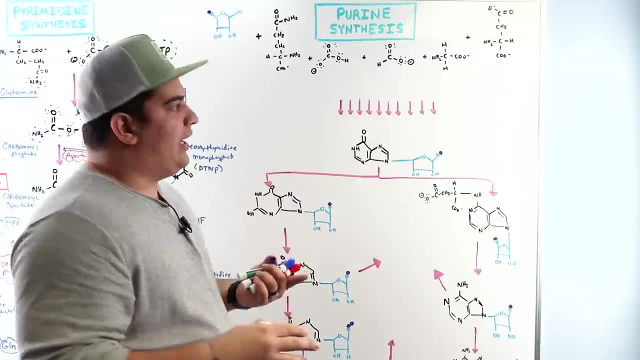 purine synthesis. Be thankful that this one isn't as crazy, because we're going to omit some of the steps in here. There's actually 10 steps in this reaction that aren't technically that high yield and it's kind of not necessary to really go over all of them, But what you should know. 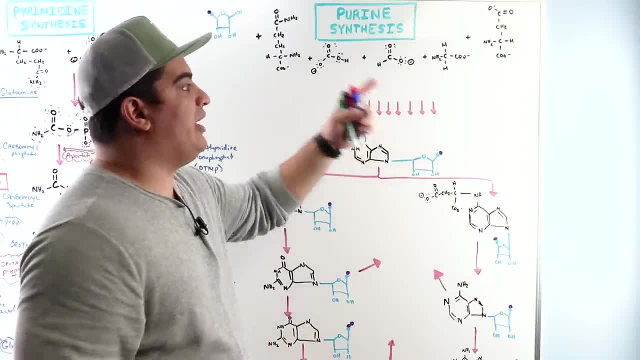 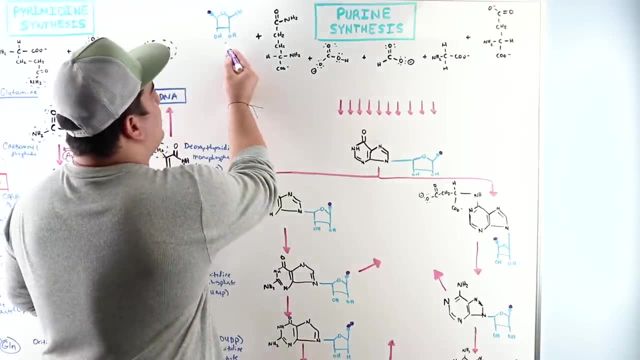 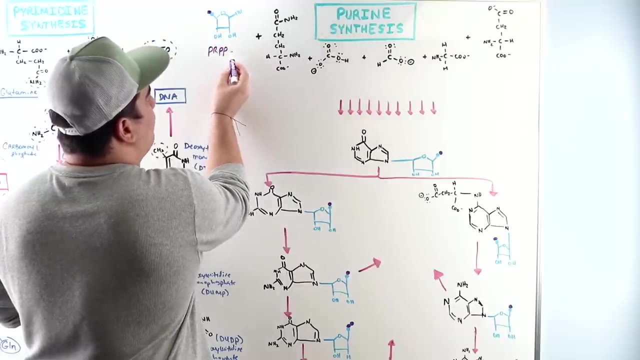 is, throughout those 10 steps, what substrates are being utilized to synthesize this product. So what are some of the substrates? If you guys remember, this is our P-R-P-P, the phosphoribosol pyrophosphate that we got from that pentose phosphate. 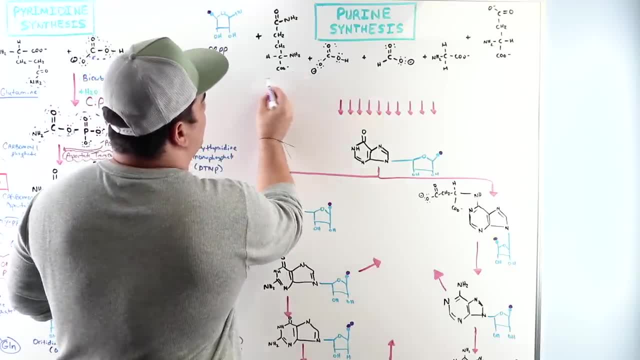 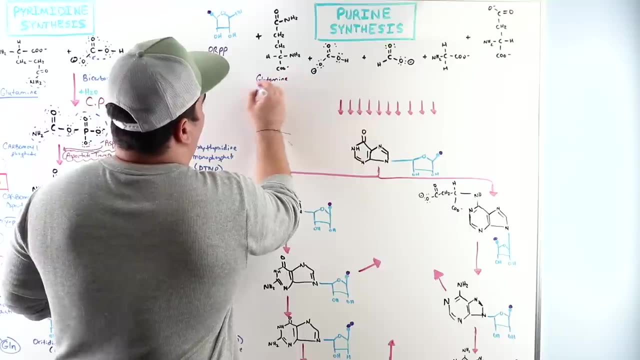 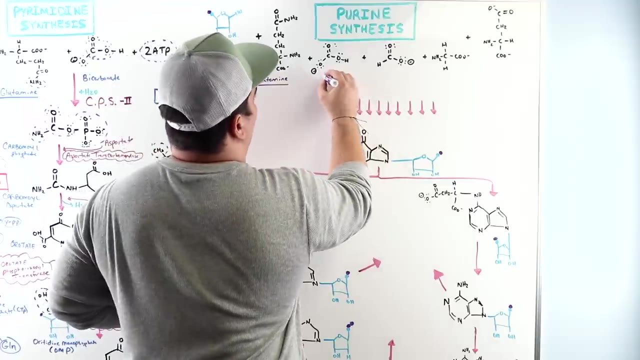 pathway right Then over here, this guy should look somewhat familiar. This is glutamine, So we got our glutamine here. And then we have another molecule here. This should look familiar. This is bicarbonate, So we're also going to have bicarbonate here. 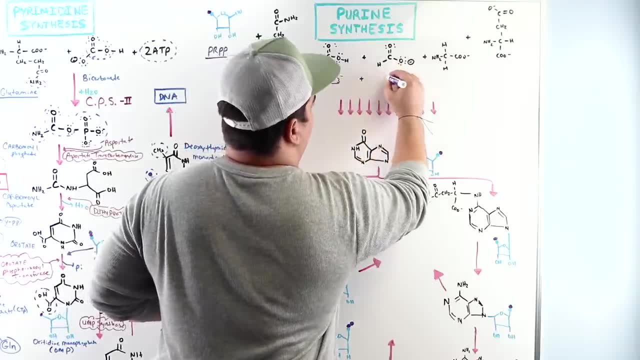 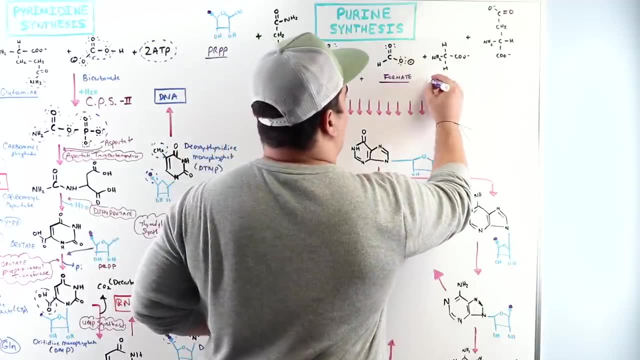 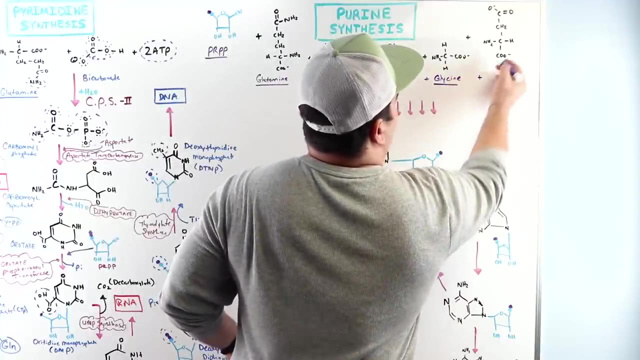 And then we're going to add a formate molecule here, So this is called formate. And then we're going to add in another amino acid here called glycine. So this is our glycine, And this last one over here is going to be aspartate. In this case, this is aspartate. 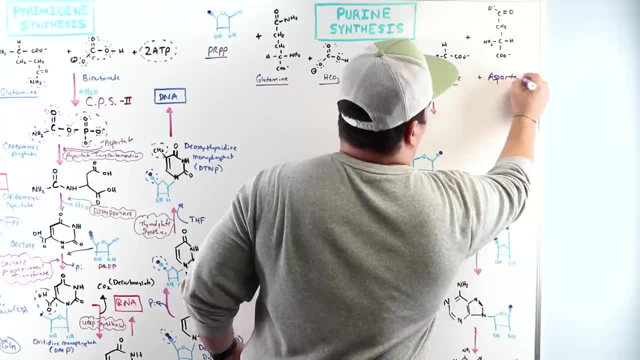 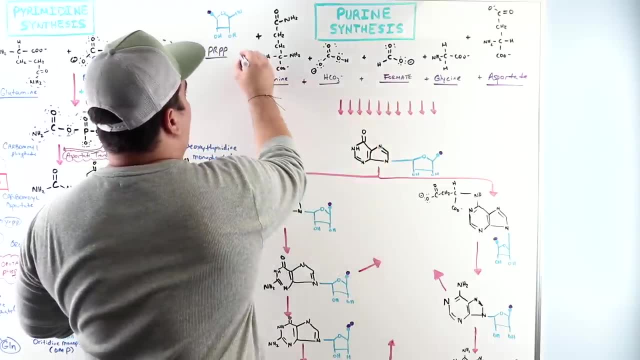 Had hydrogen, there it'd be aspartic acid, But here we have aspartate. Now we take all of these elements right. So again, P-R-P-P: glutamine, bicarbonate, formate glycine and aspartate. 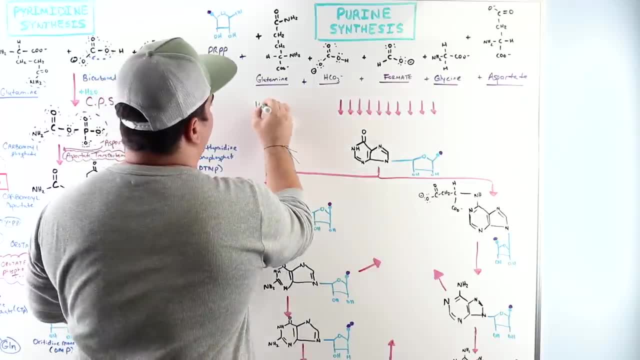 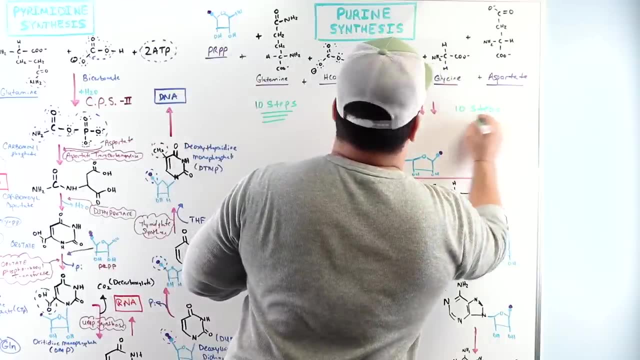 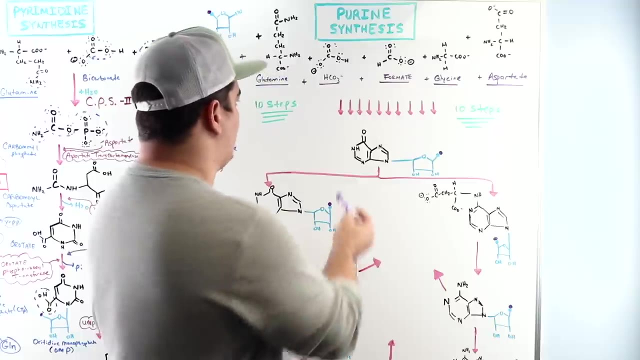 And through a series of 10 steps, we synthesize a specific molecule, And this molecule is called inosine monophosphate. So again, what is the name of this molecule here called? It is called inosine monophosphate. 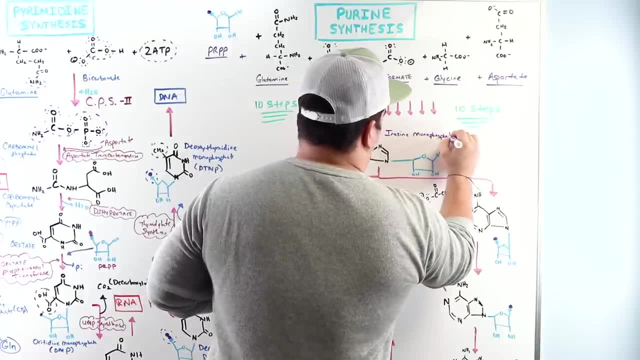 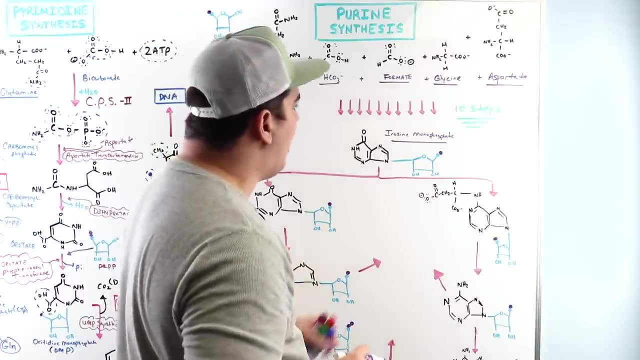 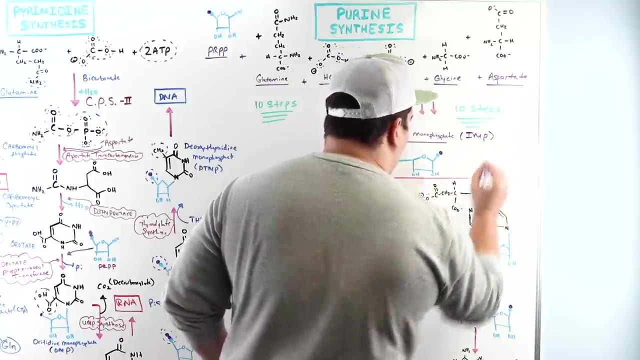 Inosine monophosphate, And all of these different molecules here were involved in synthesizing this structure. Now, inosine monophosphate, because we only have one phosphate here. And again, how would we abbreviate this? I-M-P We're going to use? 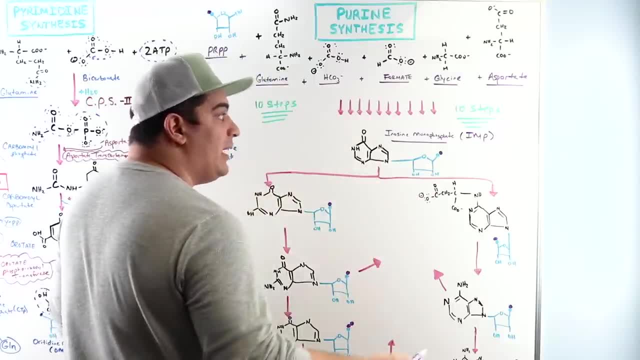 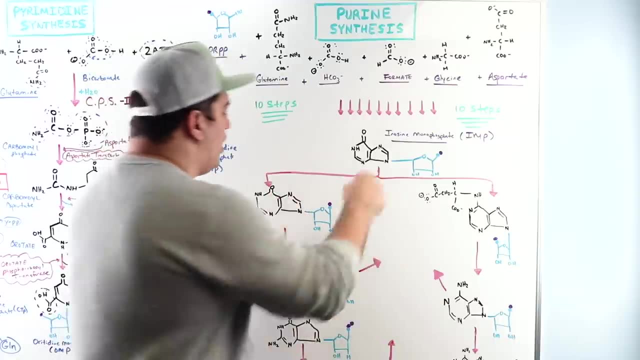 this as the precursor to synthesize AMP and GMP, or in the deoxy form: deoxy GMP, deoxy AMP. So how do we do that? Let's go with the pathway of the GMP first. So inosine monophosphate is going to react with a. 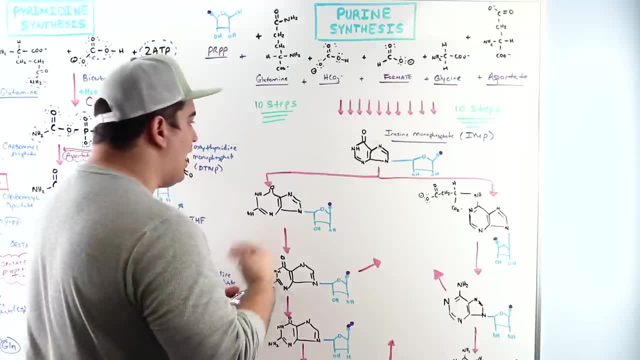 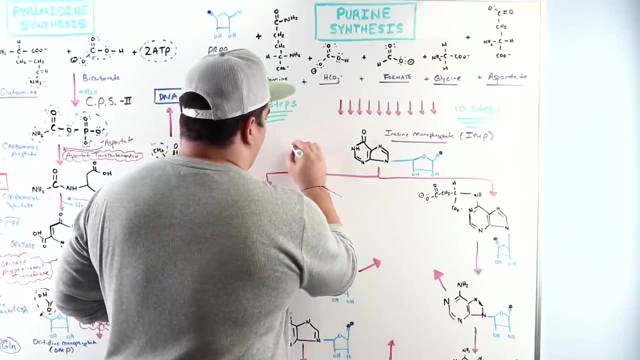 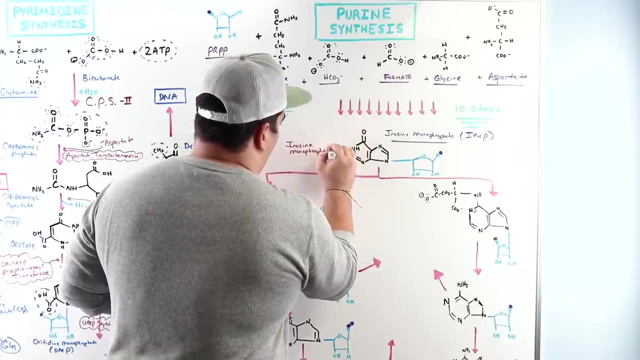 specific enzyme, And this enzyme is called inosine monophosphate dehydrogenase. That should have alarm bells ringing off in your head. So again, this is called inosine monophosphate dehydrogenase And that is going to be utilizing NAD. 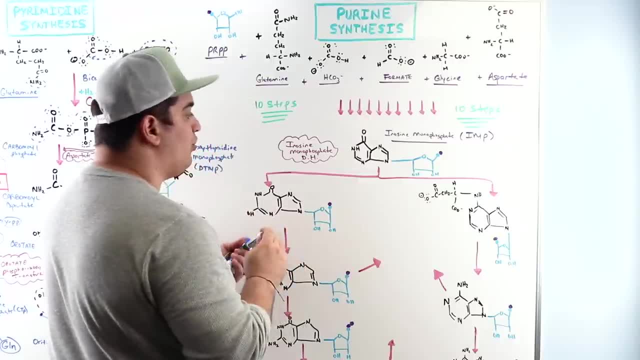 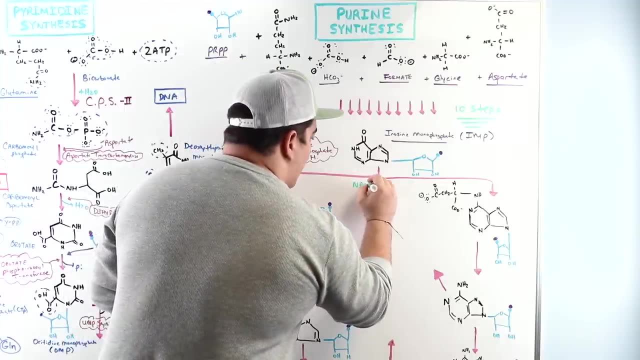 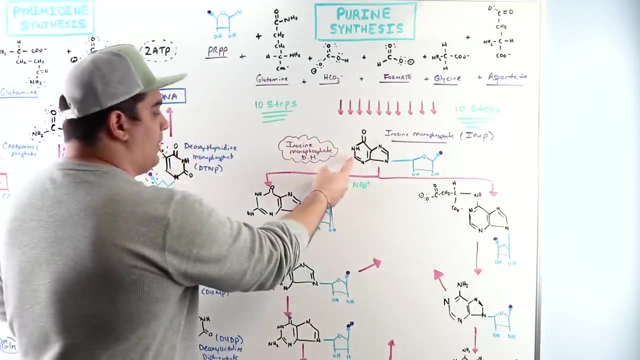 So NAD-positive molecules and converting them into NADH. So it's going to be getting reduced while oxidizing inosine monophosphate. So NAD-positive is going to be utilizing this reaction to make NADH In that process. look what happens. We add a hydroxyl group onto this, So here's going. 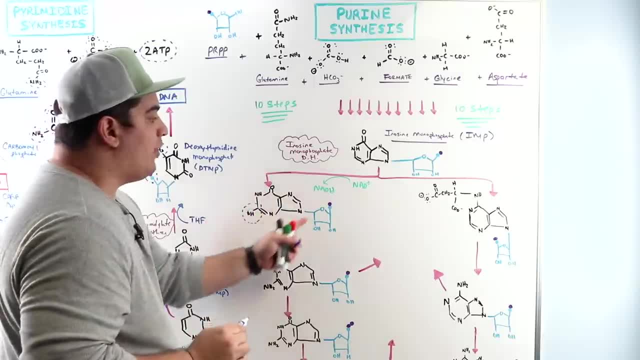 to be our hydroxyl group here. This is now a new molecule. It still has that pentose sugar, It still has the monophosphate, but now it has the NADH. So NAD-positive is going to be using this reaction. 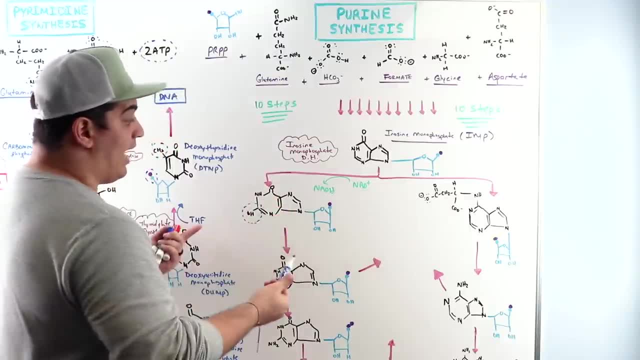 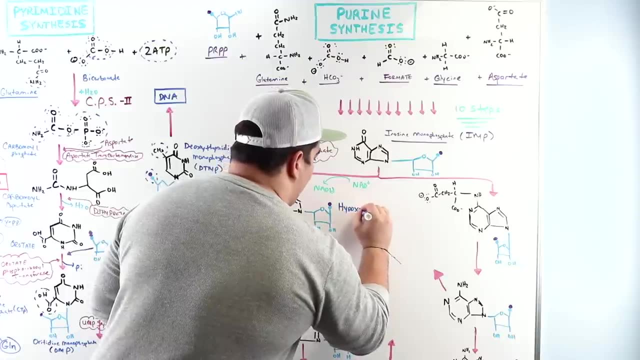 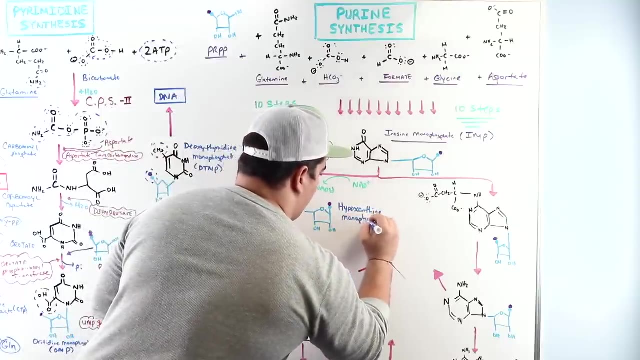 it has another component added on to the nitrogenous base. It's now a new name. What is the name of this guy? It is called hypoxanthine. How many phosphate does it have? One Hypoxanthine monophosphate. Okay, now, from here, the 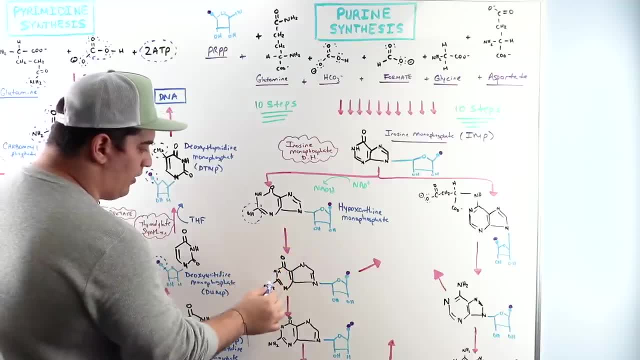 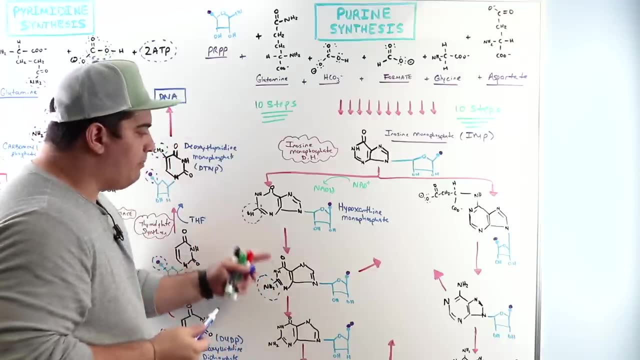 hypoxanthine monophosphate is going to go to the next step. Whoo, look what happened here. We switched the hydroxyl group and we turned this into an NH2.. Anytime we add an amine on, what did we pretty much probably use to add into it? 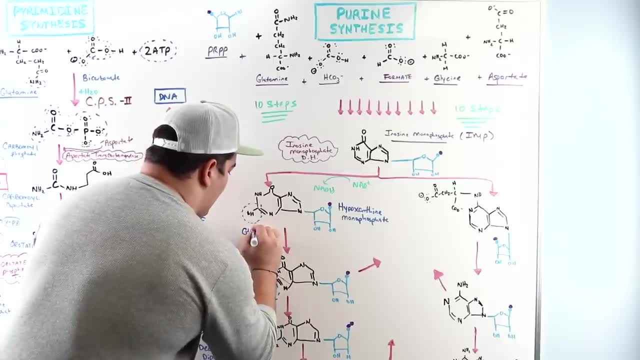 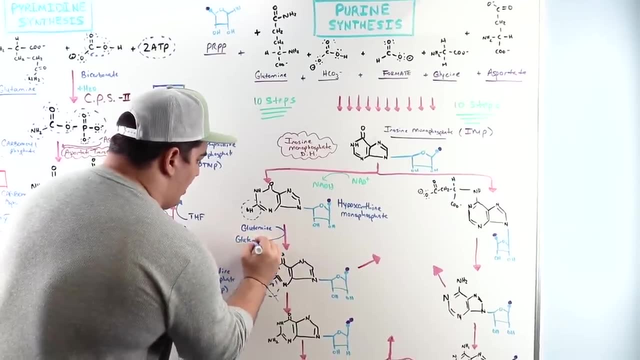 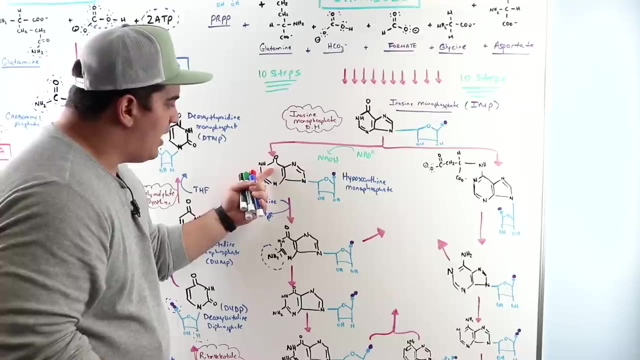 Glutamine. so somewhere along this process, I must have added glutamine and come pop that NH2 group on it. Whenever you get rid of an amine group on glutamine, it converts it into glutamate. Now, in order for me to do this, I'm going to take this hypoxanthine monophosphate and I'm going to construct anktotoxic 회 cable and put it on. Here we go. that's what we do: 1. we turn aconteceu up on and come pop on very sharp a group on. any time you get rid of a, an amine group on glutamine, it converts it into glutamate. now, in order for me to do this, I'm going to take this hate was empty monophosphate and i'm going to convert. 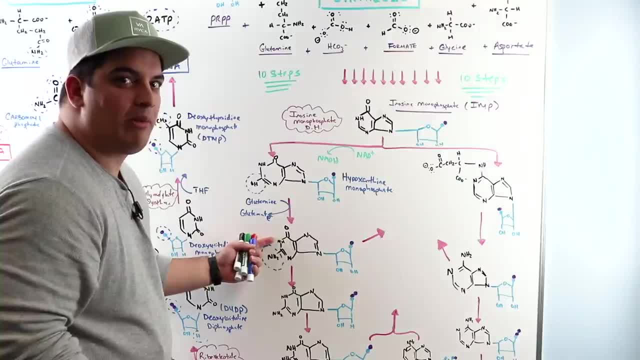 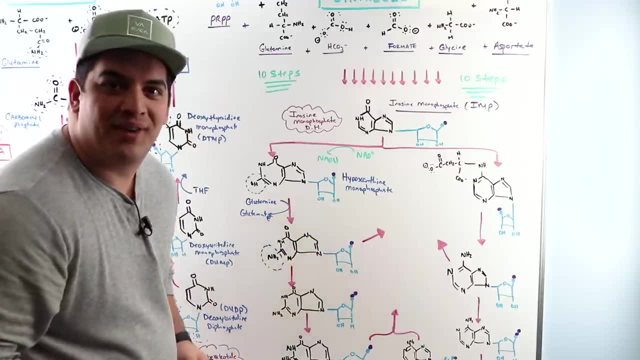 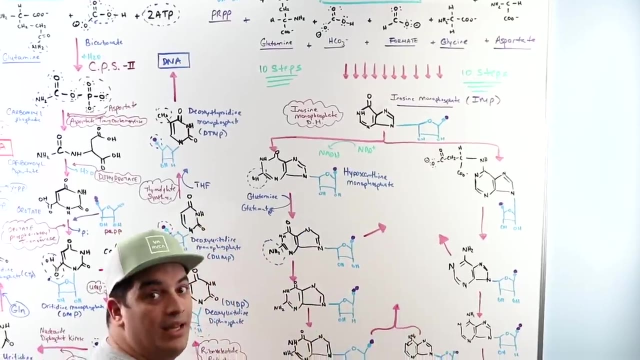 this into this new molecule. this should look familiar if you guys remember back from when we talked about the structures of the purines. this right here is guanosine monophosphate. so now we have guanosine monophosphate. so for synthesizing guanosine monophosphate, what should the enzyme be? 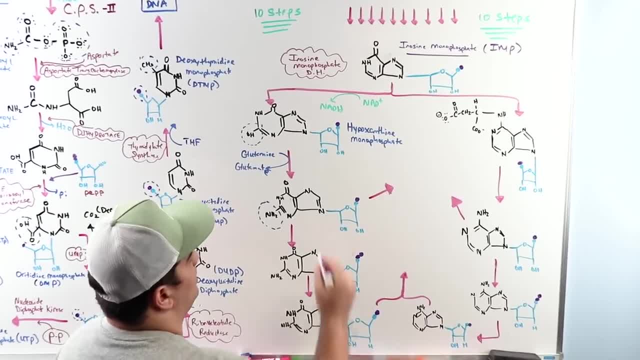 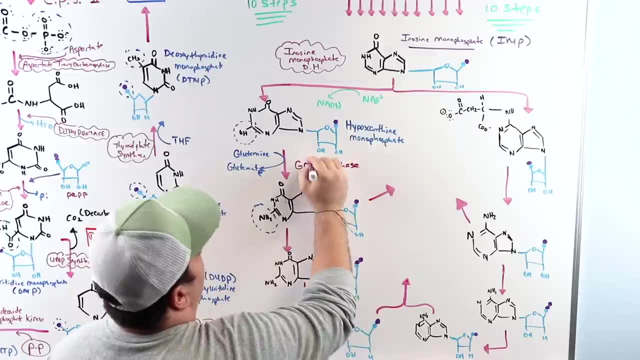 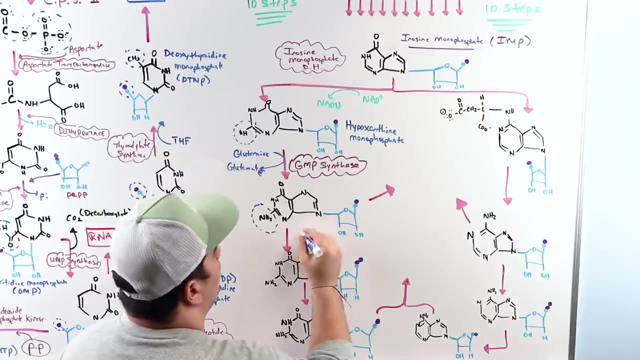 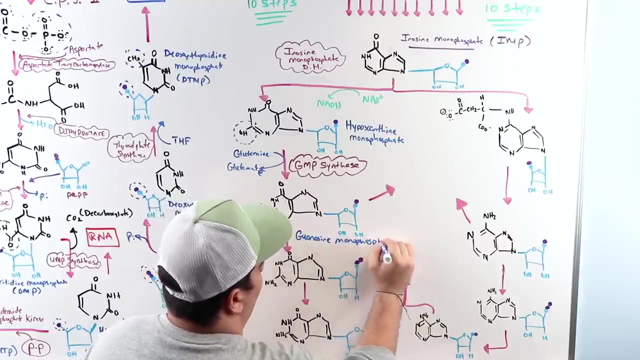 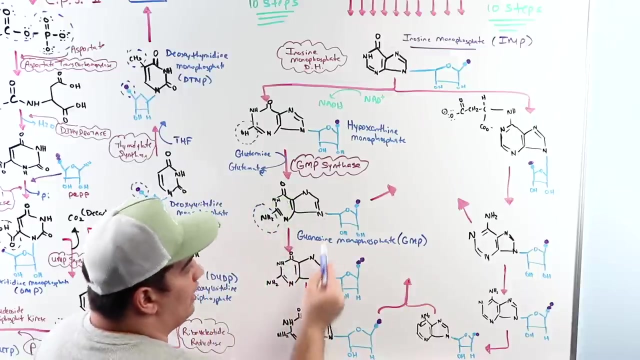 thank goodness, the enzyme in this process is called guanosine monophosphate- gmp synthase. oh, thank goodness. now we now make this new molecule, and this new molecule here is called guanosine monophosphate, which we're going to abbreviate as gmp. now, let's keep. well, actually. 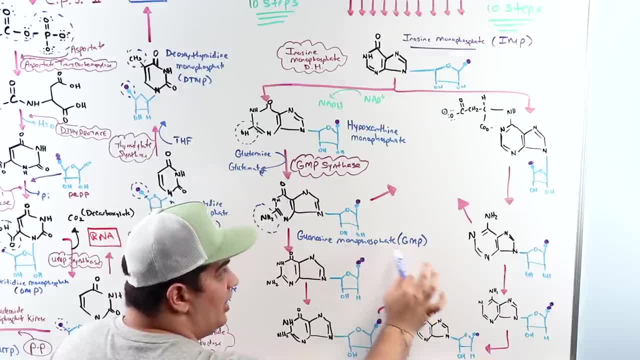 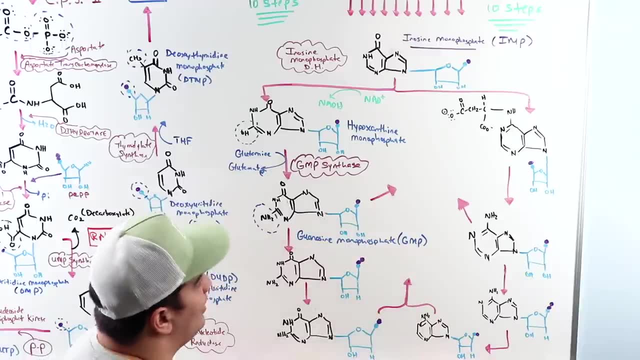 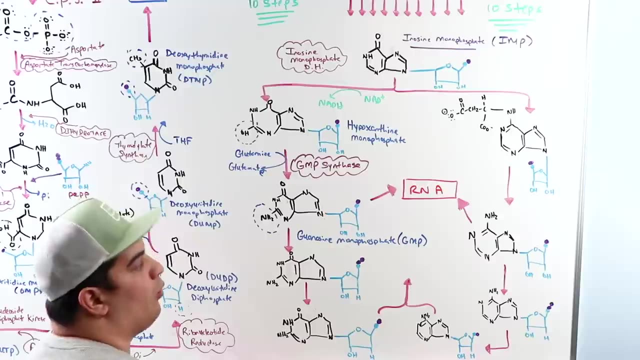 here. let's keep. let's now we said: remember, guanosine. monophosphate g can be utilized in rna and dna, so i can technically from this synthesize what rna. so now we can go ahead and make a rna molecule with this one of the components of the nucleotides. we also got to make dna right, so let's keep going. 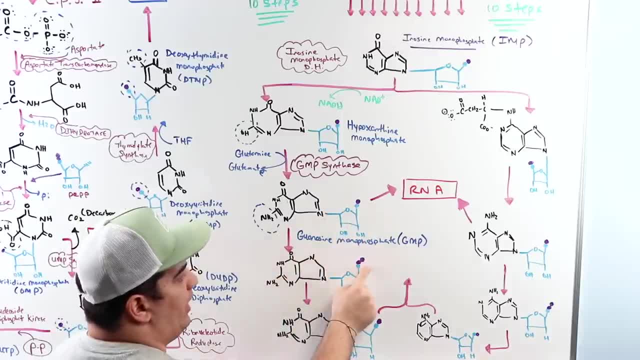 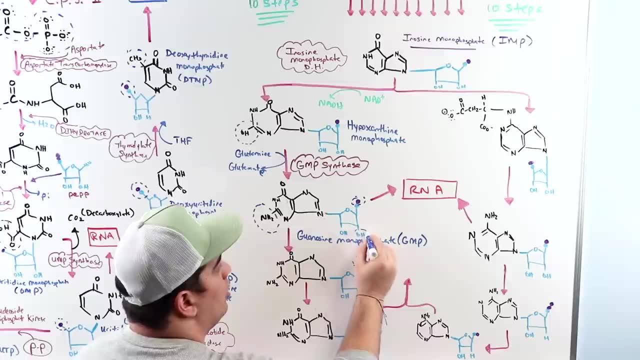 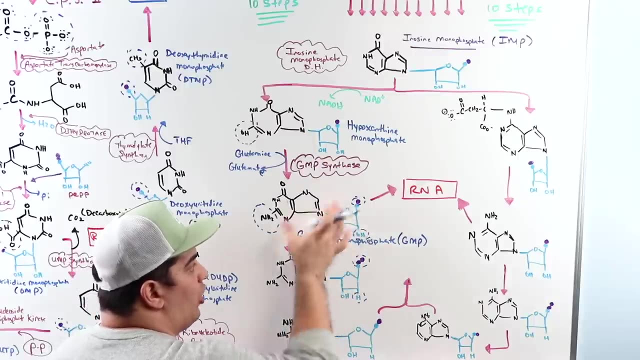 down. let's look at what happened here. we have a monophosphate. we added on another phosphate. oh guys, look, look, what happened here. one phosphate, two phosphates, oh, group here, hydrogen, group there. what was the name of that enzyme? you that converted this from a, um, a guanosine monophosphate to a deoxy guanosine diphosphate? 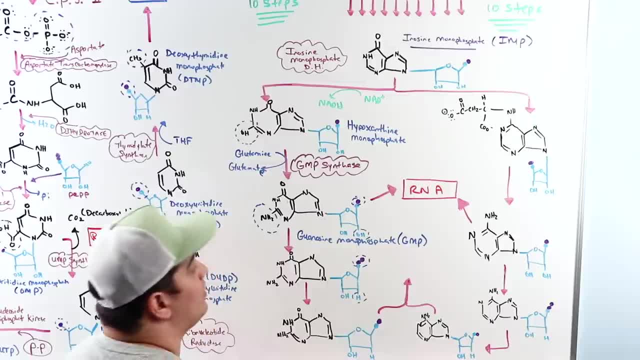 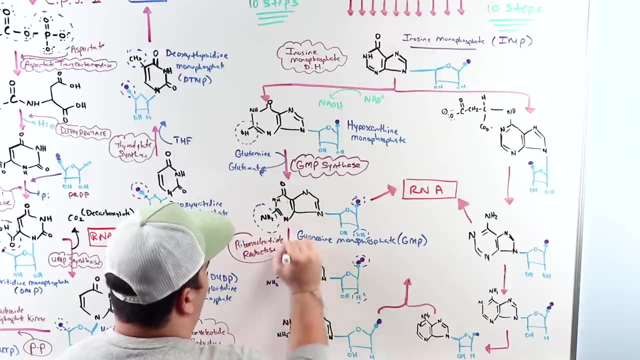 this is called the ribonucleotide reductase enzyme. so this step here is catalyzed by ribonucleotide reductase. and again, what do we do? we added in a phosphate group into this reaction and we converted the hydrogen group into this reaction and we converted the hydrogen group. 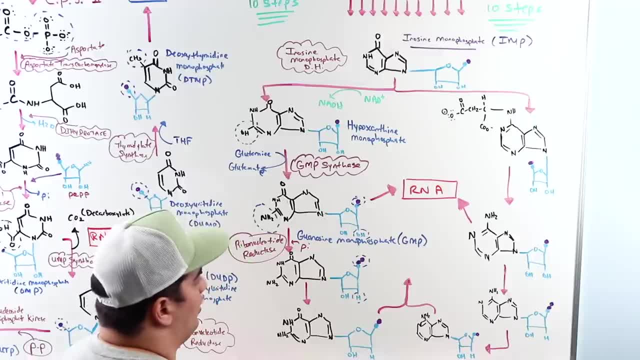 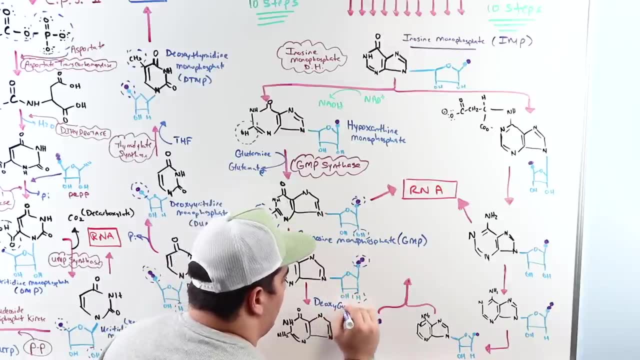 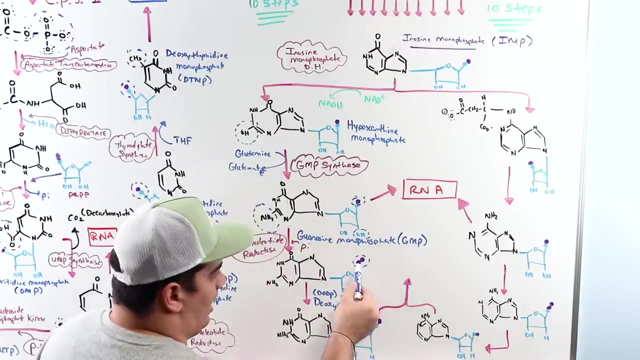 hydroxyl group into a hydrogen. now this new molecule is called deoxy, because we converted this into a deoxy sugar here, and this is guanosine. and how many phosphates? two, so it's diphosphate. what's the um abbreviation? it's d g d p. well, let's look at the next step. here i have two. 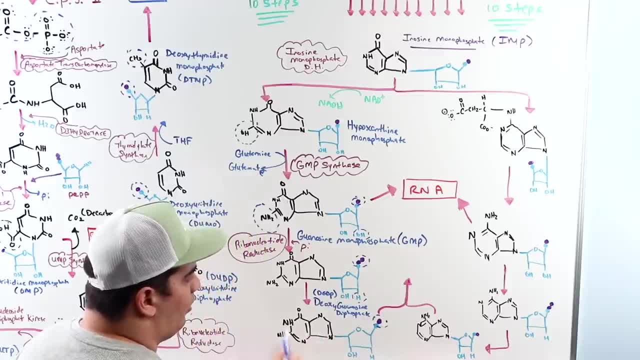 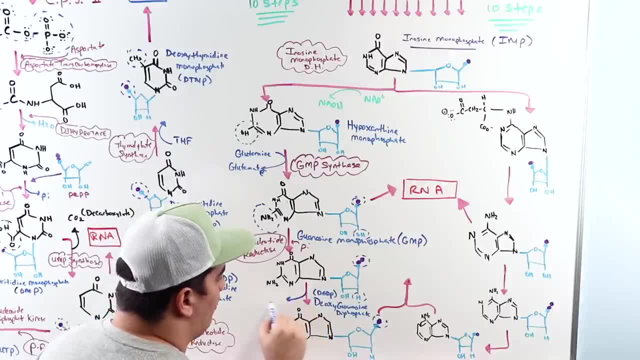 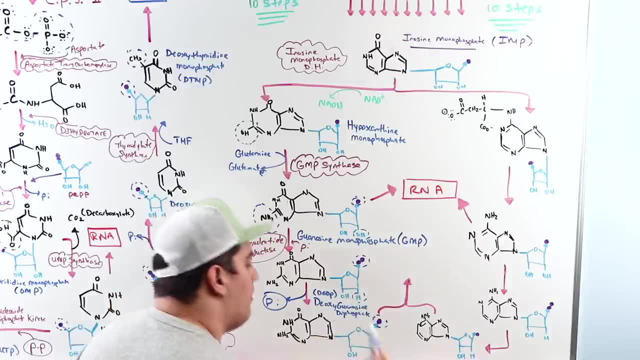 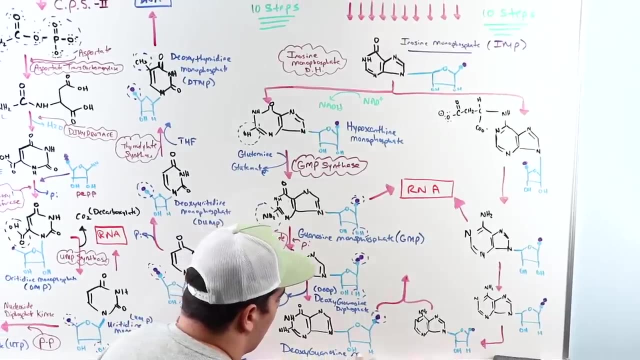 base here. So all I did was popped off a phosphate. I popped that sucker off. When I do that now, it's just deoxyguanosine monophosphate, So this here is called deoxyguanosine monophosphate. 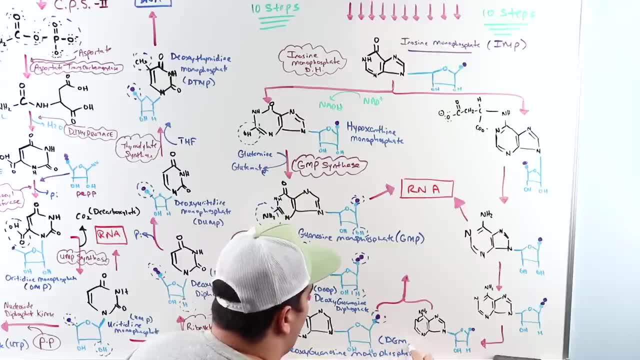 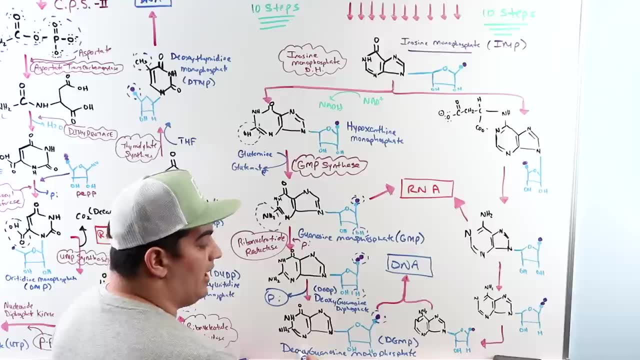 which we can abbreviate as DGMP, And that is used to synthesize what DNA? Because it can be used in making RNA and DNA, And we already talked about this. It's deoxy for DNA and guanosine monophosphate. 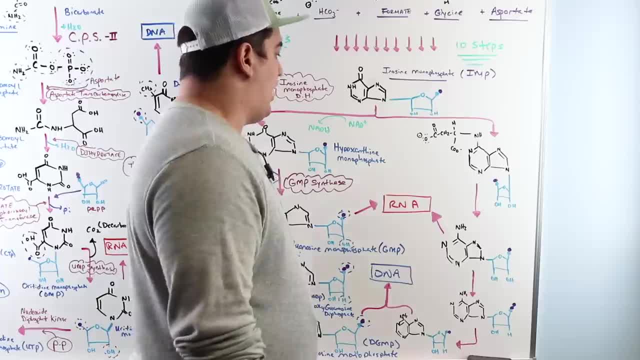 for RNA. Now let's go do the adenosine. All right. So now we took inosine monophosphate and we synthesized the guanosine monophosphate or the deoxyguanosine monophosphate. Now we got to go. 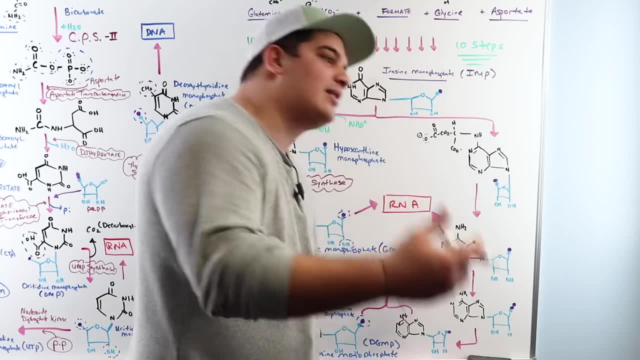 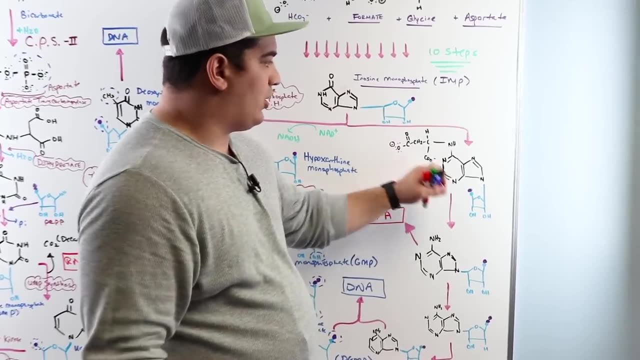 synthesize adenosine monophosphate and deoxyguanosine monophosphate. So let's go do that. So if you look here at the adenosine monophosphate and compare it to this next molecule, what looks different? Oh, I don't got this thing on there previously. 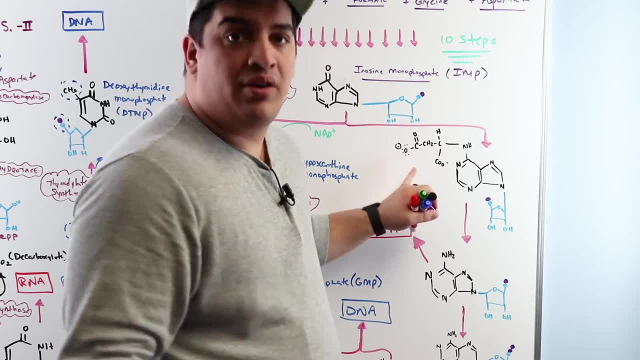 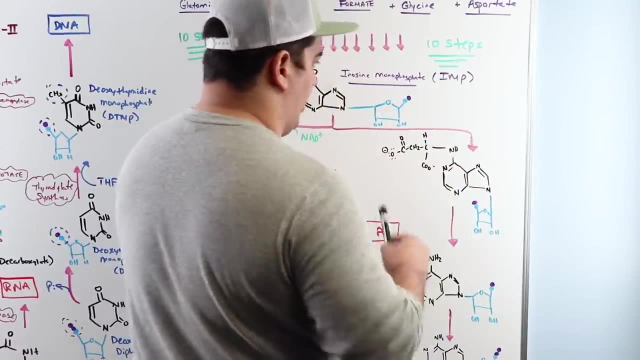 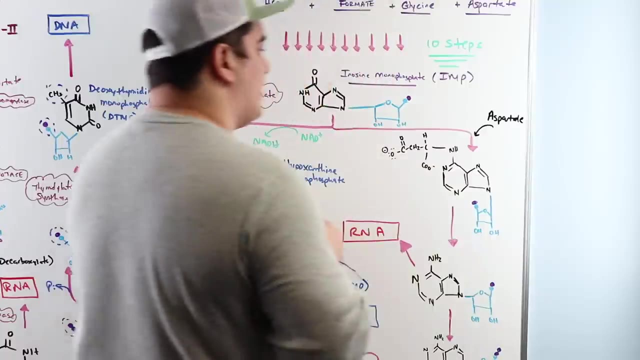 What the heck is that? Well, that's actually aspartate. We're going to add this on here. So in this process we use aspartate and we add that molecule on here. So here we're going to just have aspartate. aspartate, which is an amino acid. We're going to add this on here. 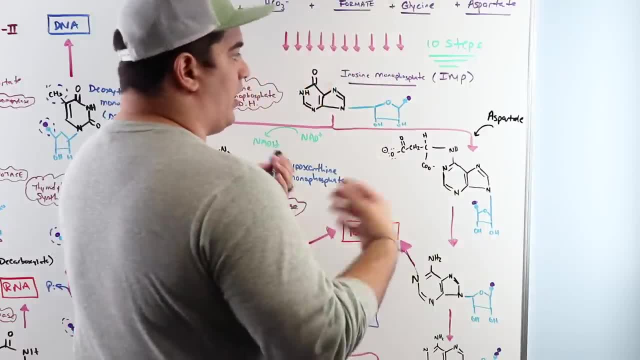 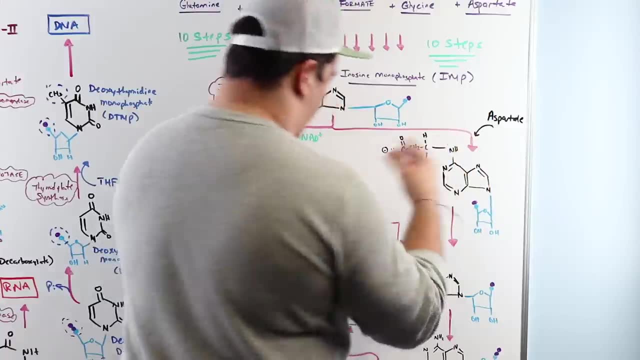 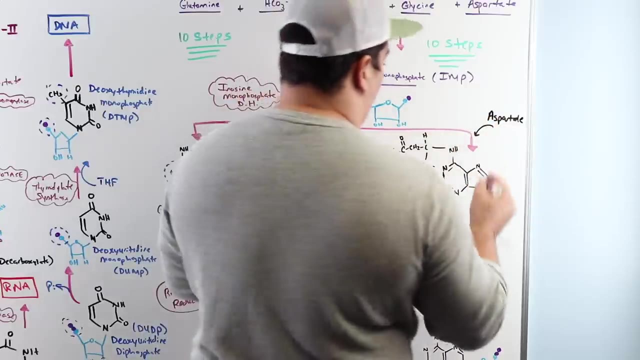 And we're going to make this new molecule called adenylosuccinate. So, thank goodness, they made the enzyme called adenylosuccinate synthase. So the enzyme that's catalyzing this step of inosine monophosphate plus the aspartate, making this next molecule called adenylosuccinate. 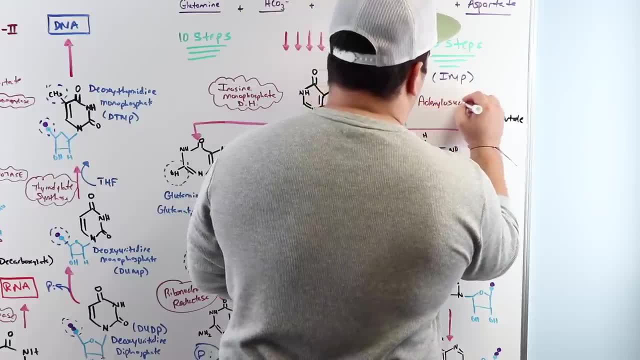 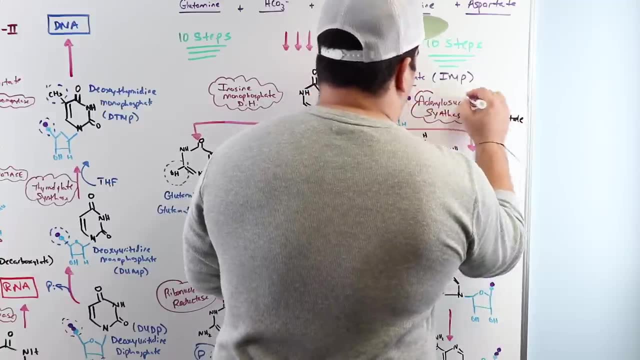 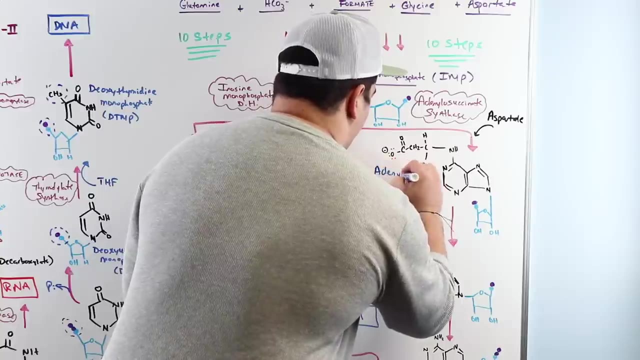 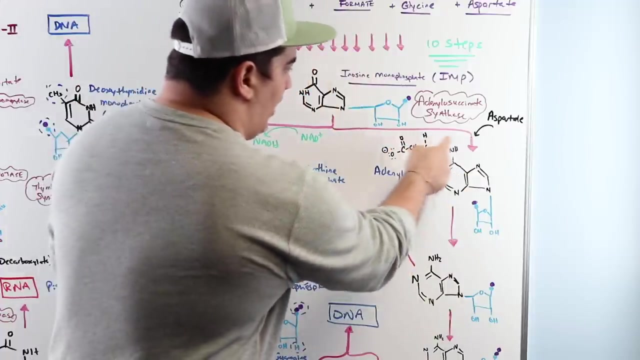 is called adenylosuccinate synthase And that is going to catalyze this new molecule. So we're going to step and make this next molecule here And this next molecule is called adenylosuccinate. Now, adenylosuccinate. compare. the next molecule Here we have the aspartate. 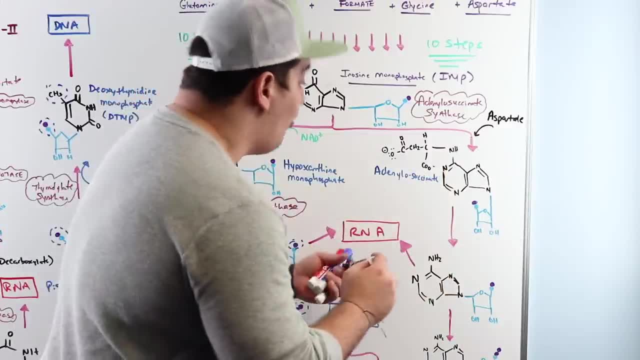 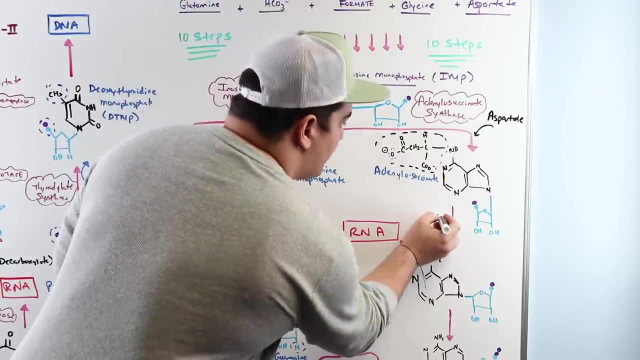 What the heck? Now that thing is gone. Where did it go? This whole thing here pops off, And when it pops off, except without this amine group there, because it didn't have previously have an amine group, it pops off And when it pops off except without this amine group. 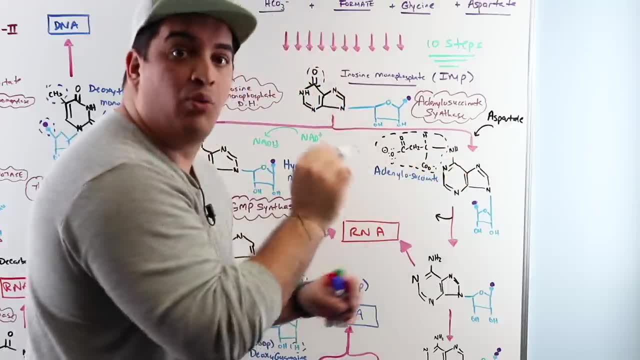 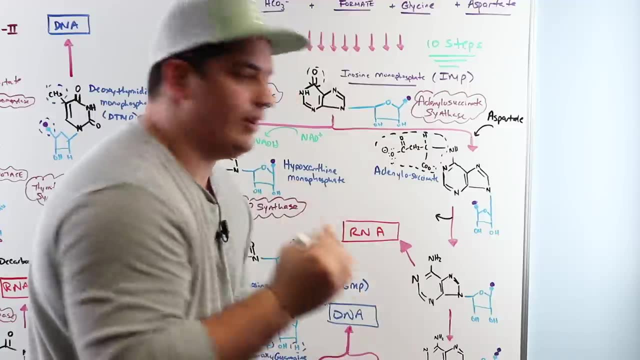 here that amine got added. That's what we wanted. We wanted that amine group there. We're going to pop this thing off And this new molecule here is called fumarate. So we're going to make this next molecule which is going to pop off here called fumarate. Doesn't that sound? 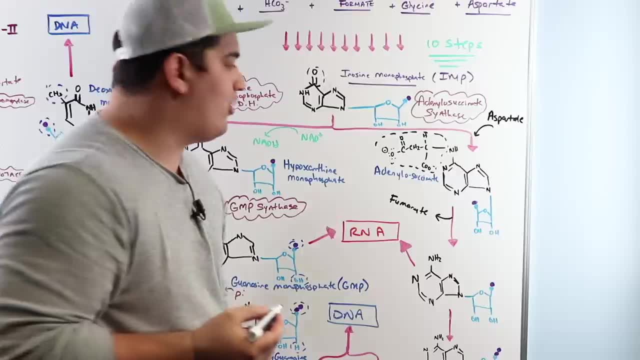 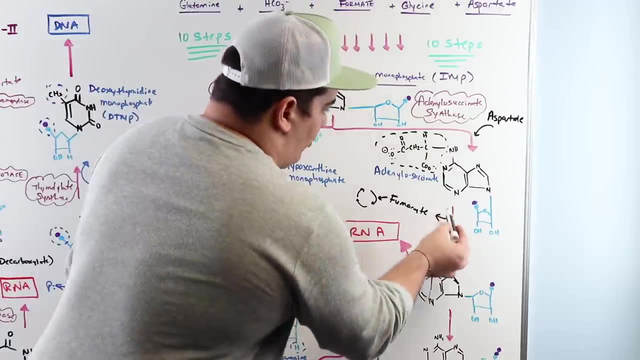 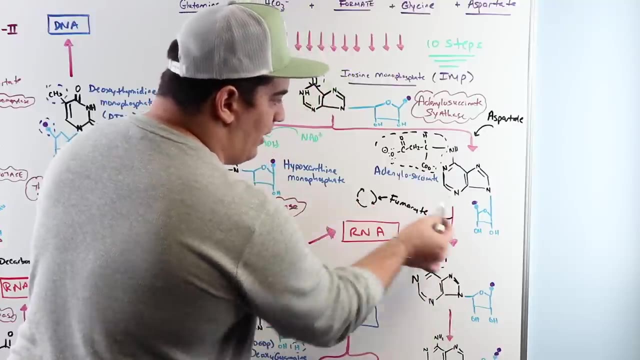 familiar. Where'd the fumarate molecule come from? The Krebs cycle, So this can then get shuttled in and maybe be involved in the Krebs cycle Now, after we pop off the fumarate and we leave this amine group on. now we had to pop this adenylosuccinate. We had to remove a specific 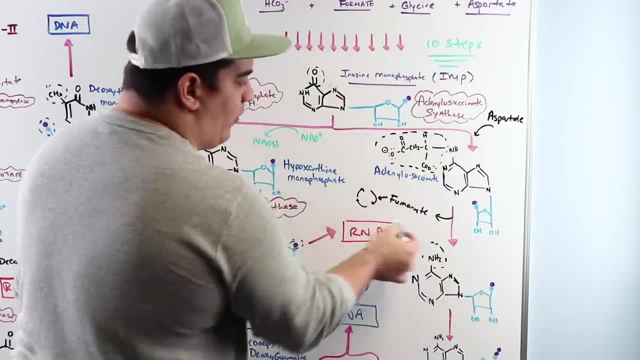 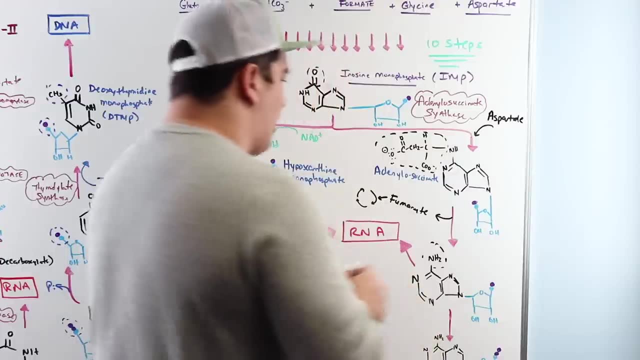 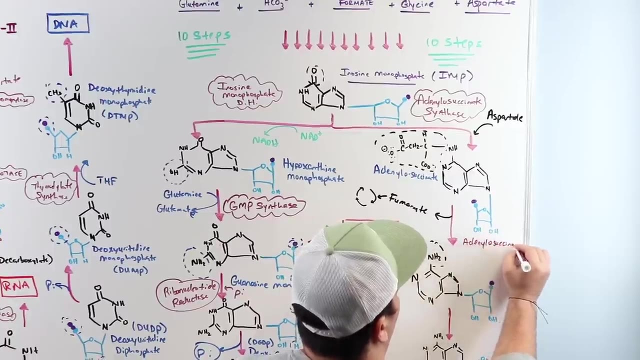 molecule off of it right Which was removing a part of the aspartate in the form of fumarate. So we technically cut the adenylosuccinate. So we're going to call this enzyme here which catalyzes this step, adenylosuccinate lyase, Because that thing going to cut adenylosuccinate. 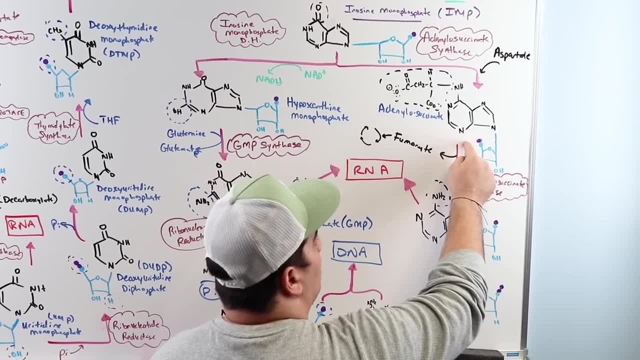 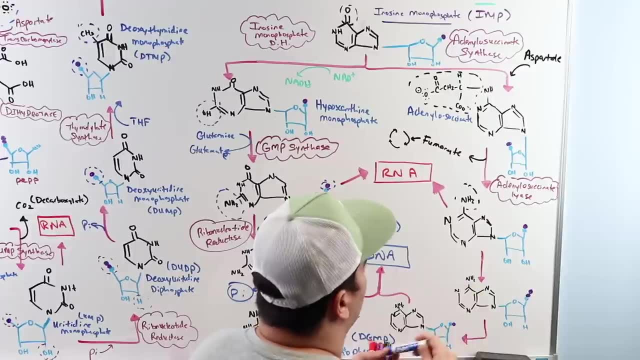 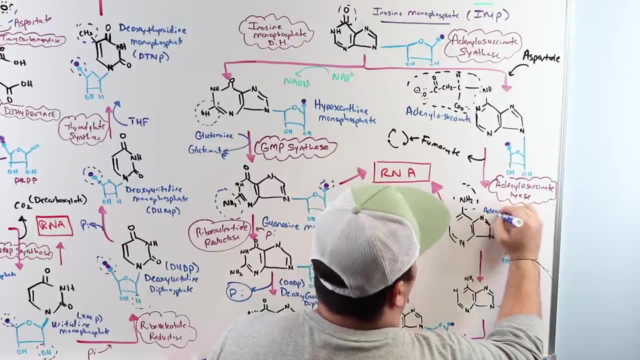 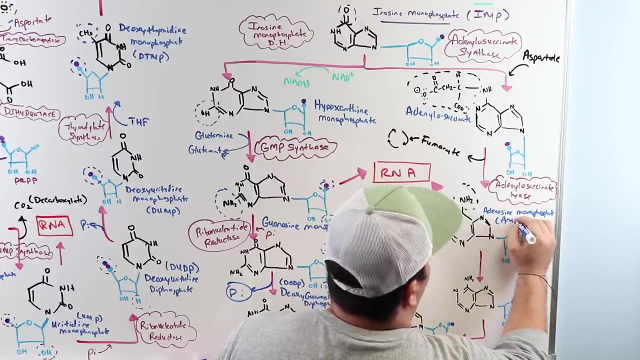 And then we're going to convert this adenylosuccinate molecule into adenosine monophosphate. This should look familiar. So now this new molecule is called adenosine monophosphate. So we're going to put the adenosine monophosphate which we denote as AMP. What can AMP be utilized for? 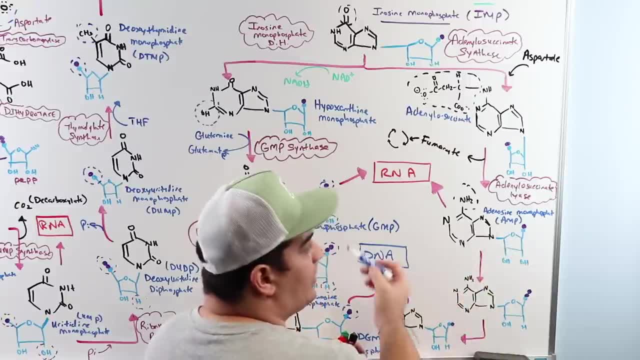 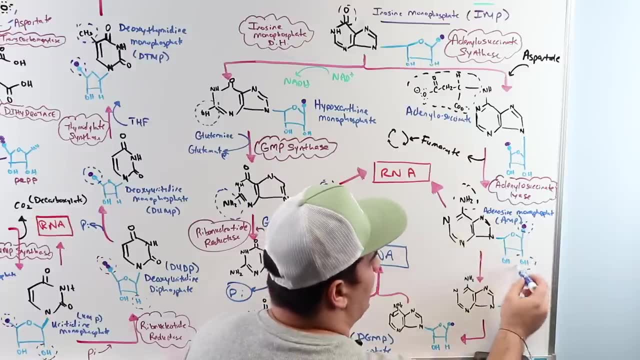 Synthesizing RNA, But again we need to get the deoxy form. So how do we do that? Look here: Here's one phosphate group. Here's two phosphate groups. I'm going somewhere. Here's the hydroxyl group. Oh, it's gone. What was? 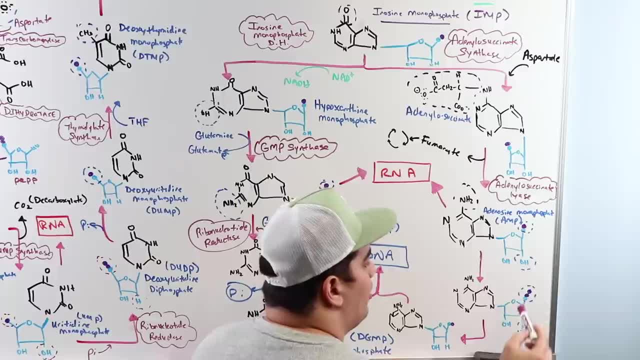 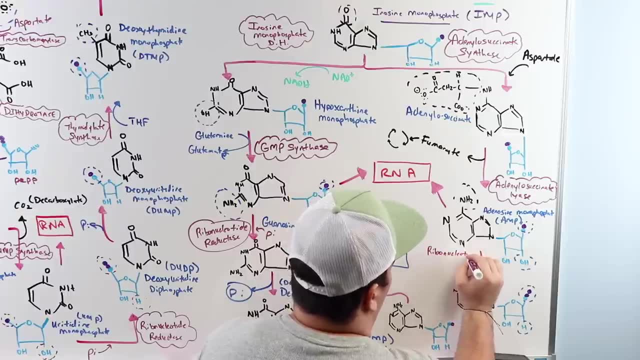 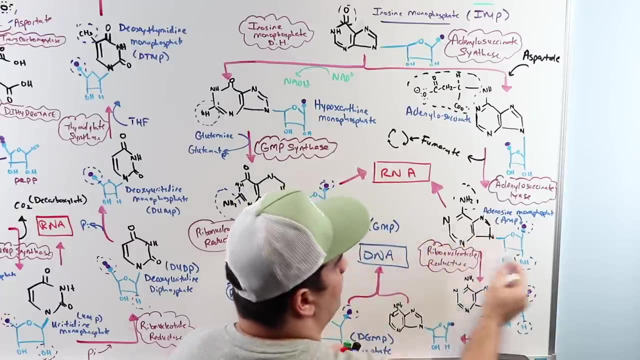 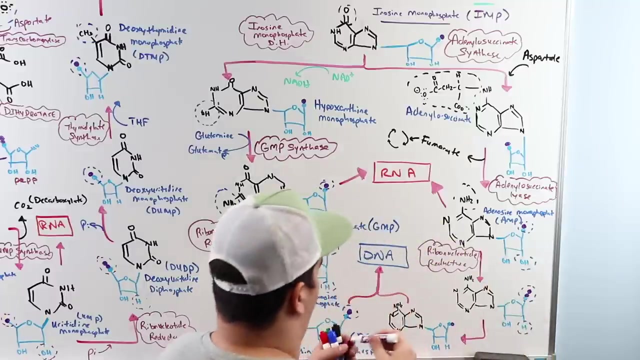 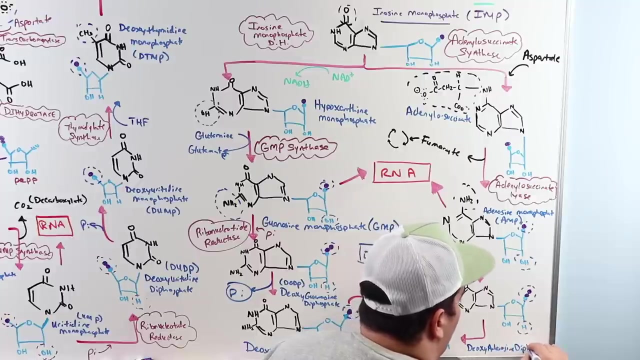 the name of the enzyme that catalyzed this step and converted it from a ribonucleotide to a deoxyribonucleotide- Ribonucleotide reductase. And this ribonucleotide reductase will convert this adenosine monophosphate to deoxyadenosine diphosphate. Adenosine di phosphappe. 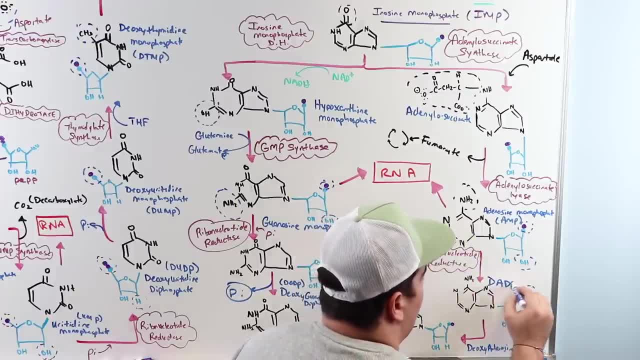 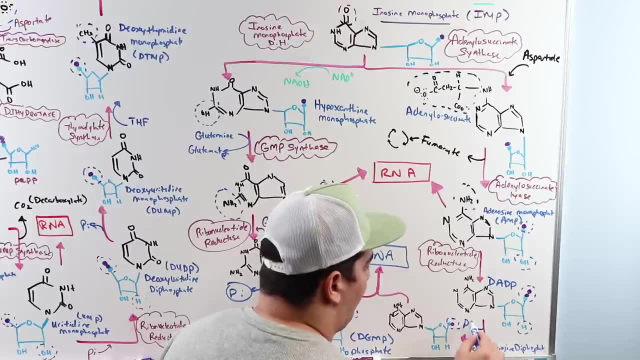 And we're going to abbreviate this as D Detoxyadenosine, DHalphosphate. Well, I need the-. What am I going to do now? I had two phosphates, One phosphate. I popped off that phosphate and now